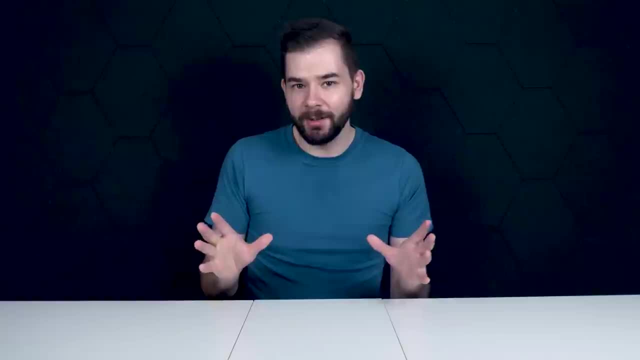 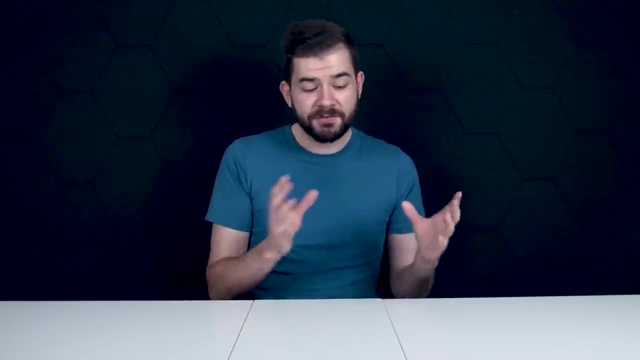 A quick disclaimer. This video is intended as a primer on first order logic, to help students who are learning the subject for the first time. If it's something that you're already familiar with, this might not be the video for you, Or maybe you'll see a fresh perspective. 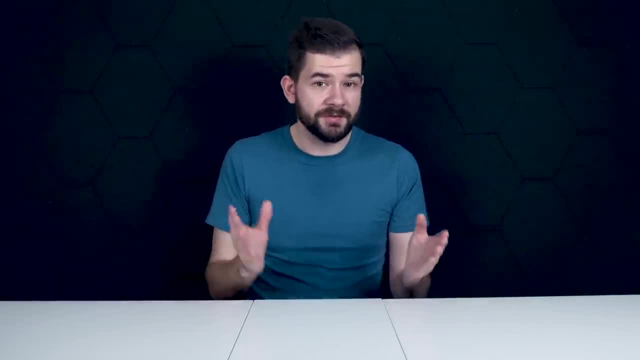 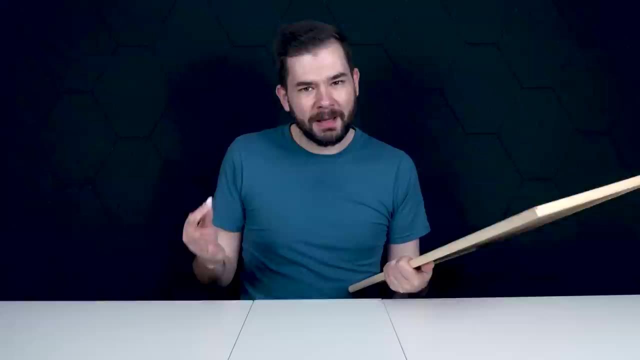 new ways of thinking about or new ways to teach the material that you'd never considered before. I probably shouldn't discourage people from watching my own video, but I just want to be upfront about what this video entails. So what is mathematical logic? Well, it's the study of 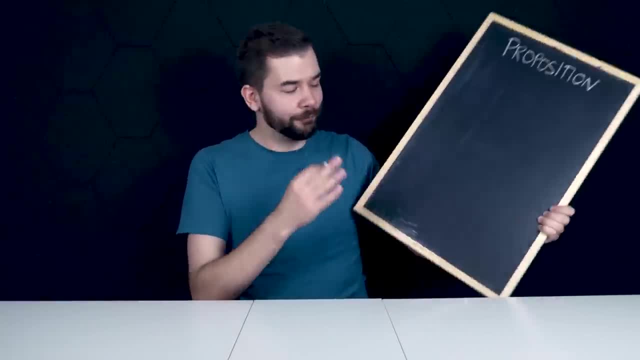 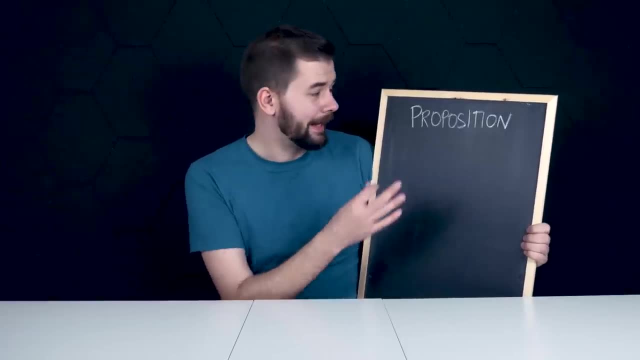 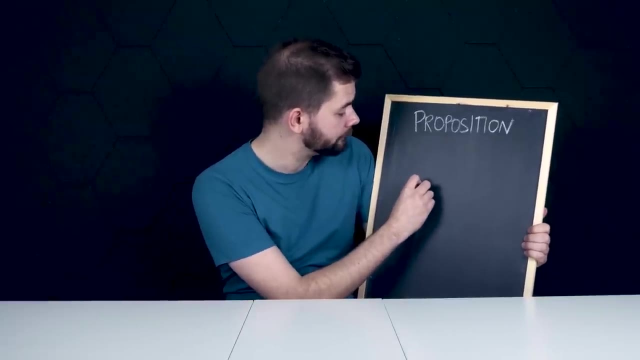 the truth of mathematical statements, which we call propositions. But much of what we learn today can be applied in non-mathematical contexts as well. A proposition is a claim that can either be true or false. So if I take a number like X and I make the claim X equals one, then this: 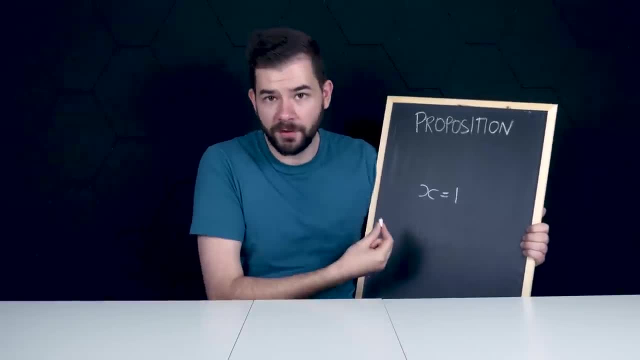 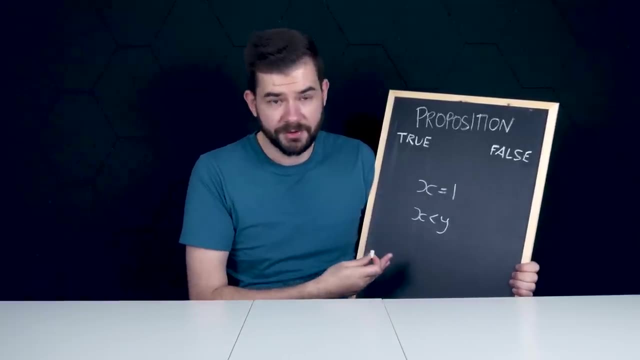 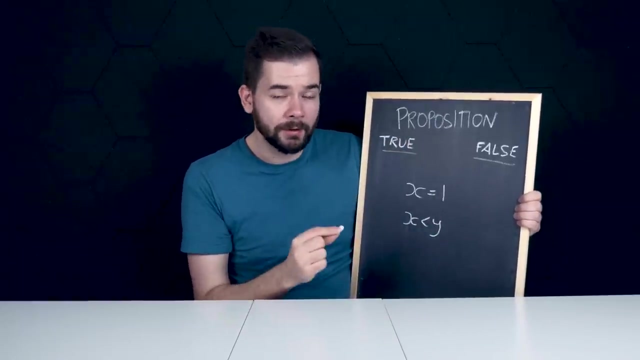 is a proposition because X is either one or it is not one. It's true or false. If Y is also a number, then X is less than Y is also a proposition. It's a claim. either true or false. Propositions can be true, false, but never both. That's known in logic as: 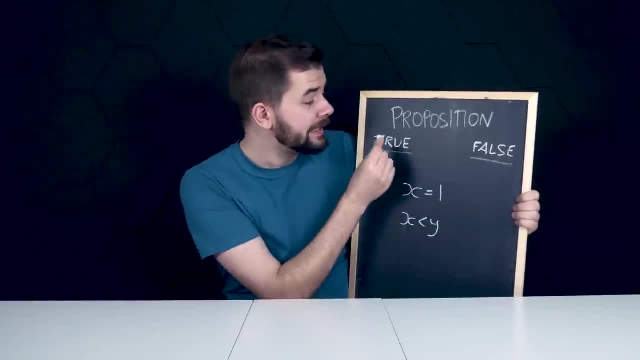 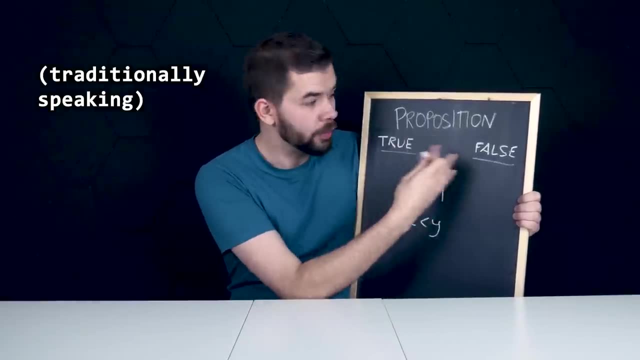 the law of non-contradiction, And propositions must either be true or false. There is no middle ground. That's a law that's known as the law of excluded middle, because there's no middle territory. The other law that you'll find at the foundation of logic is the law of identity. 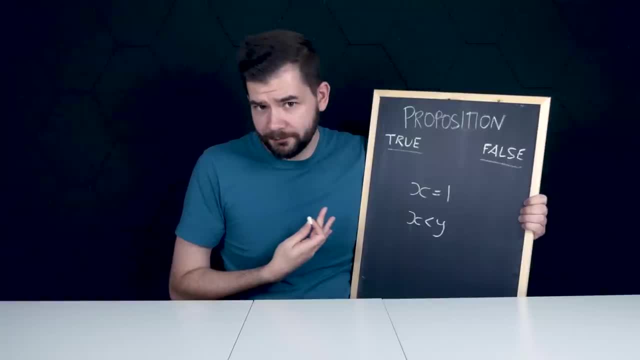 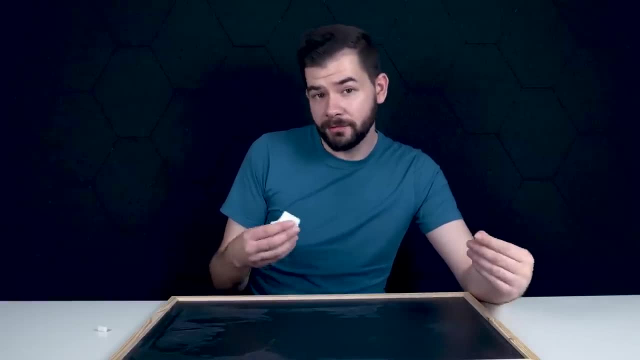 which says that, no matter what, always be true to yourself- I'm kidding, It is that for any entity X, X is always equal to X. I should note here that propositions should not be subjective, and it sometimes depends on how the terms are defined, For example for the proposition. 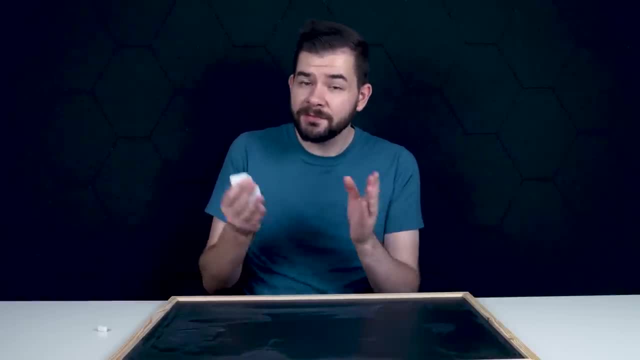 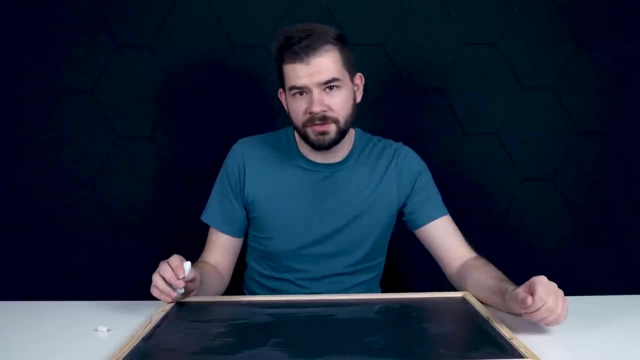 I like pie to be valid and non-subjective. it depends on how the terms are defined. Am I talking about the number pie or am I talking about the food pie? Either way, the proposition is true, because who doesn't like pie and who doesn't like pie? Fortunately. 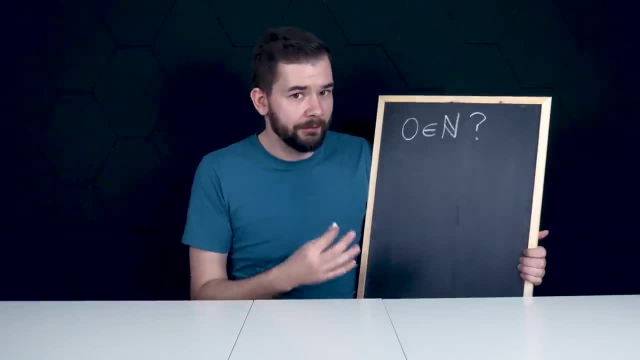 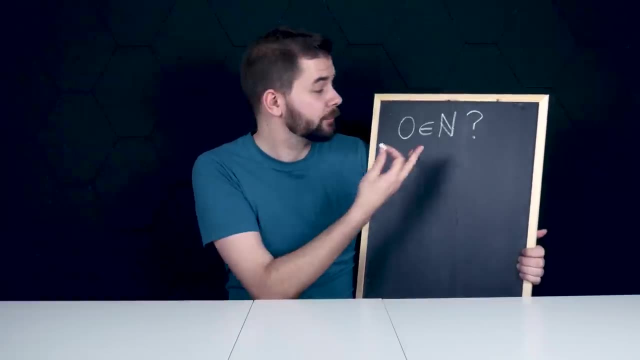 mathematical propositions rarely stray into that kind of subjective territory. The worst that can happen is something like this, where you make the statement zero is a natural number. There's no broad consensus as to whether zero is included in the natural numbers, so it's really up to the 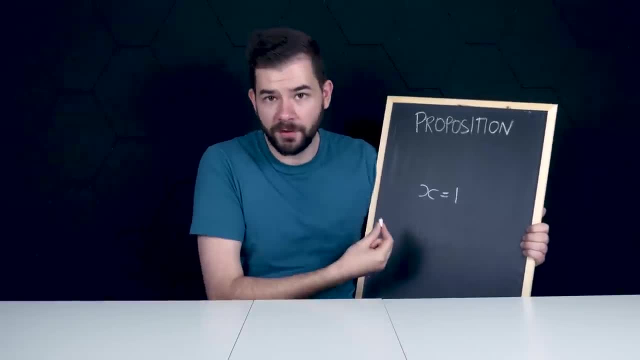 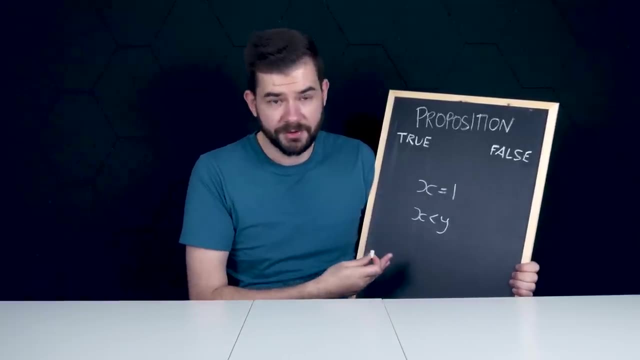 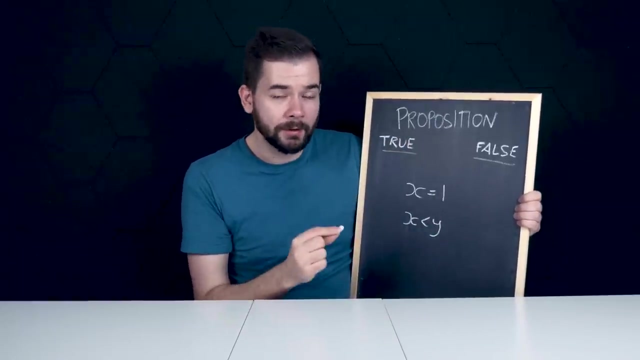 is a proposition because X is either one or it is not one. It's true or false. If Y is also a number, then X is less than Y is also a proposition. It's a claim. either true or false. Propositions can be true, false, but never both. That's known in logic as: 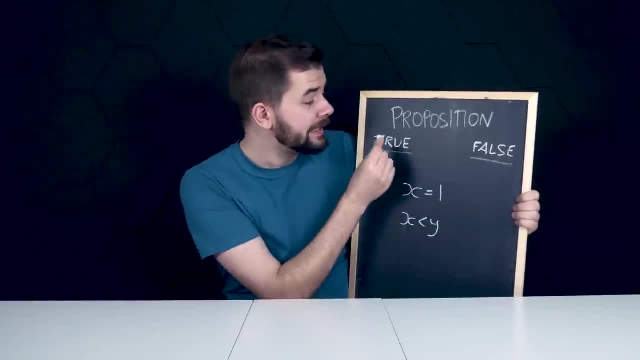 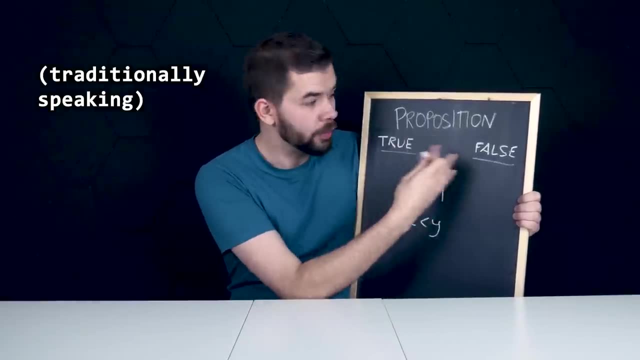 the law of non-contradiction, And propositions must either be true or false. There is no middle ground. That's a law that's known as the law of excluded middle, because there's no middle territory. The other law that you'll find at the foundation of logic is the law of identity. 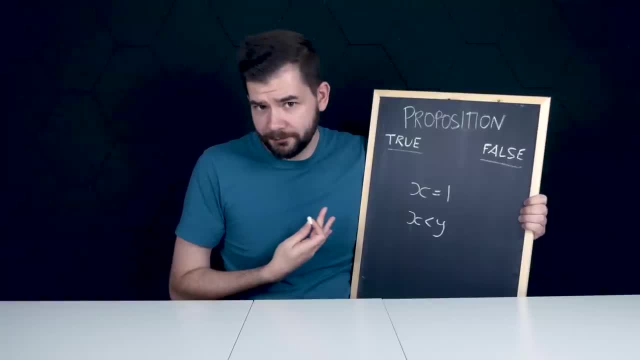 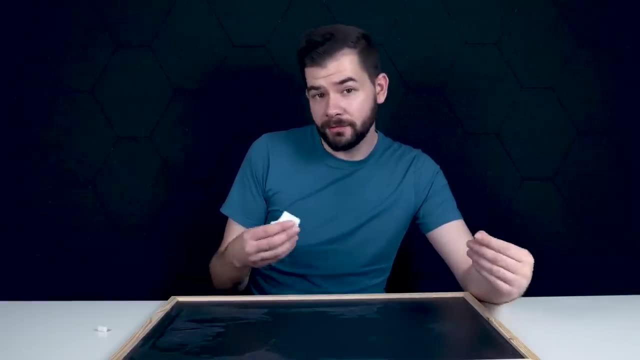 which says that, no matter what, always be true to yourself- I'm kidding, It is that for any entity X, X is always equal to X. I should note here that propositions should not be subjective, and it sometimes depends on how the terms are defined, For example for the proposition. 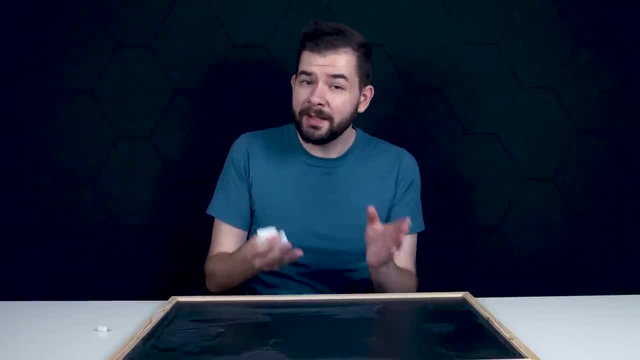 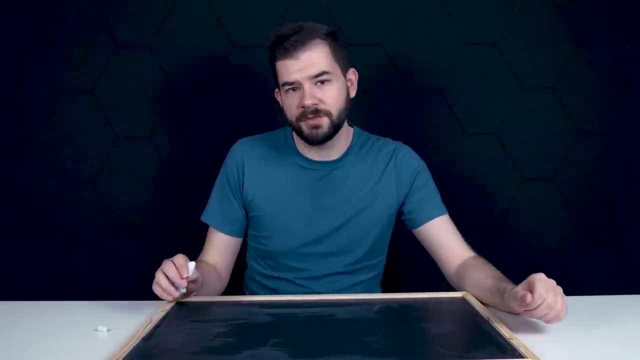 I like pie to be valid and non-subjective. it depends on how the terms are defined. Am I talking about the number pie or am I talking about the food pie? Either way, the proposition is true, because who doesn't like pie and who doesn't like pie? Fortunately, mathematical propositions rarely. 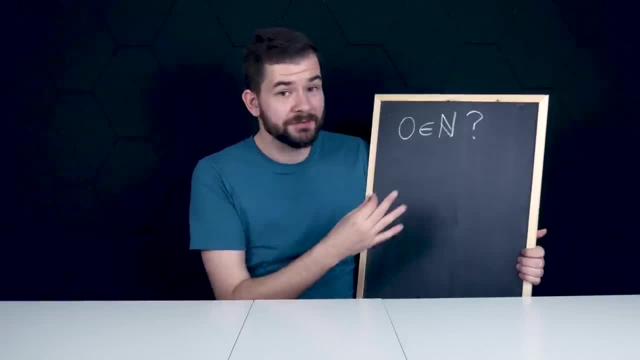 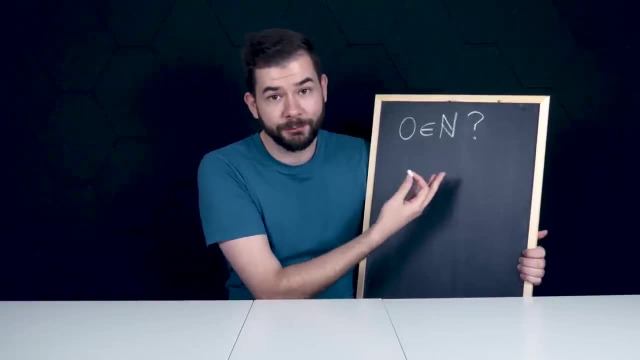 stray into that kind of subjective territory. The worst that can happen is something like this, where you make the statement zero is a natural number. There's no broad consensus as to whether zero is included in the natural numbers, so it's really up to the 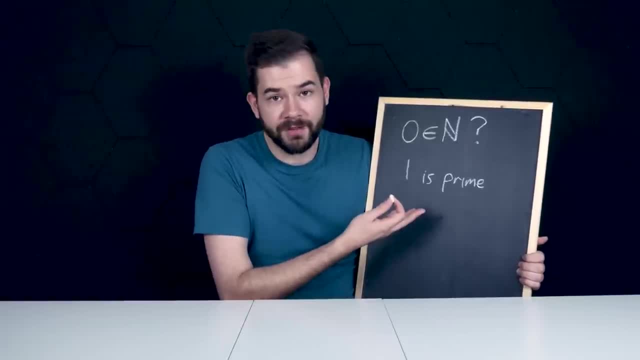 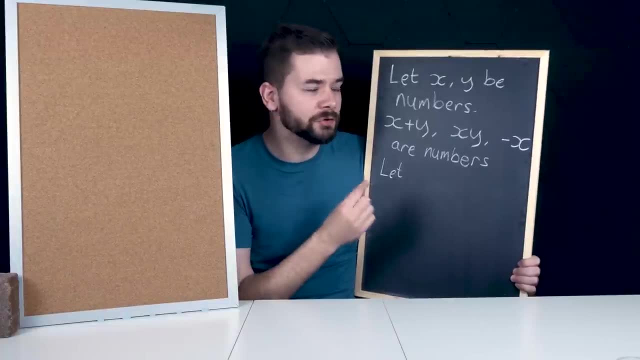 author. Another one might be. one is prime, which we would all say is false. but I spent a whole video discussing how sometimes it is and sometimes it isn't. A bit like how in algebra I can let X and Y be numbers and then combine them through the usual operations to create new numbers. 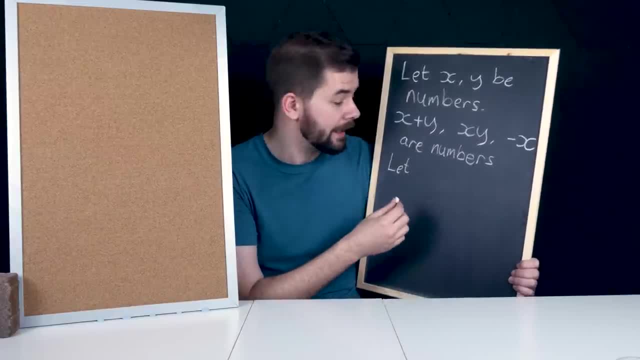 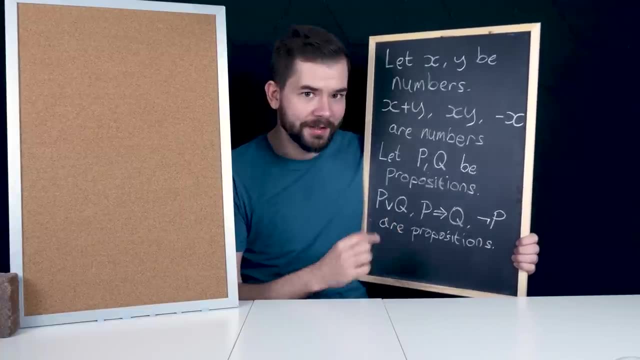 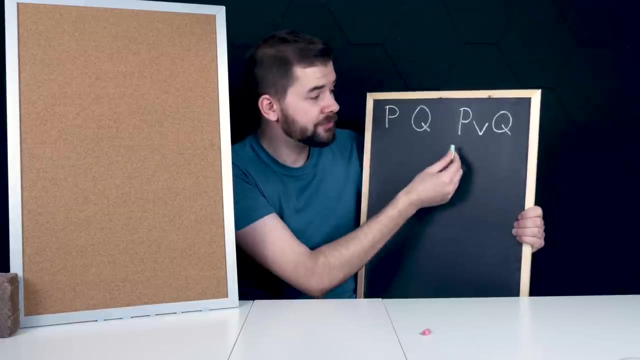 I can also do the same with propositions. So if I let say be propositions, then I have some operations I can do to combine these to make new propositions. So let's break down what these symbols mean. The first one is or, So P or Q is true whenever P is. 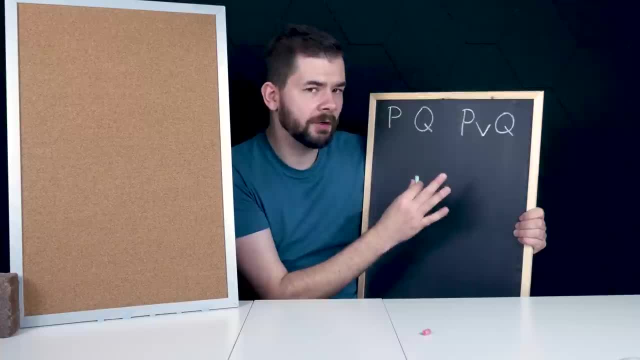 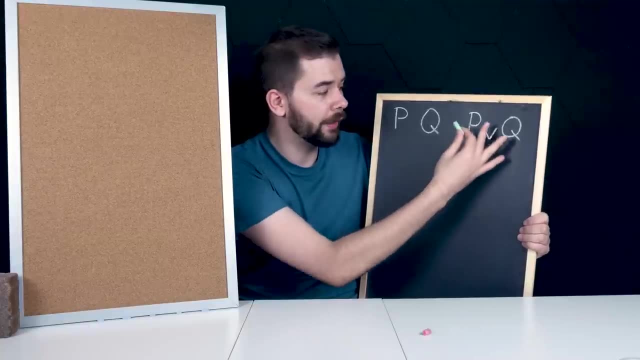 true, Q is true, or if they're both true, It's only false when both P and Q are false, And I can actually draw up all the combinations of true and false here to show you exactly when this is true in something that's called a truth table. So let's look at an example. If I say X is greater, 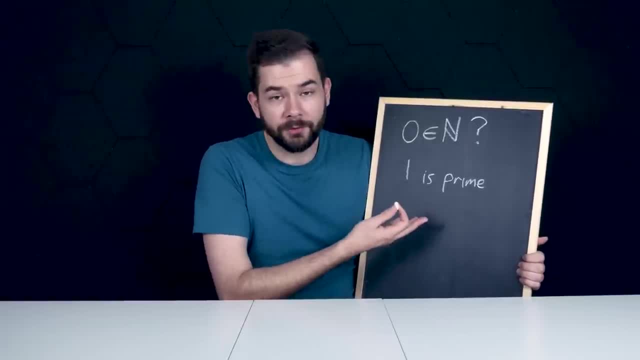 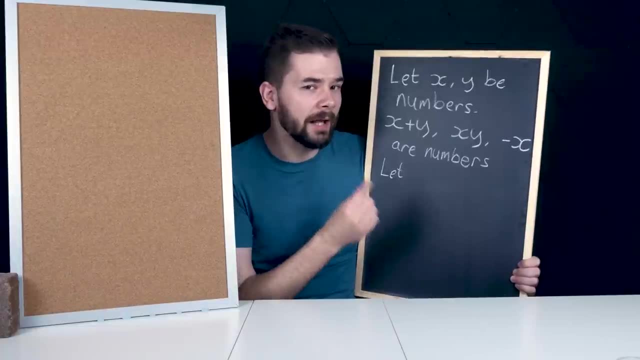 author. Another one might be. one is prime, which we would all say is false. but I spent a whole video discussing how sometimes it is and sometimes it isn't. A bit like how in algebra I can let X and Y be numbers and then combine them through the usual operations to create new numbers. 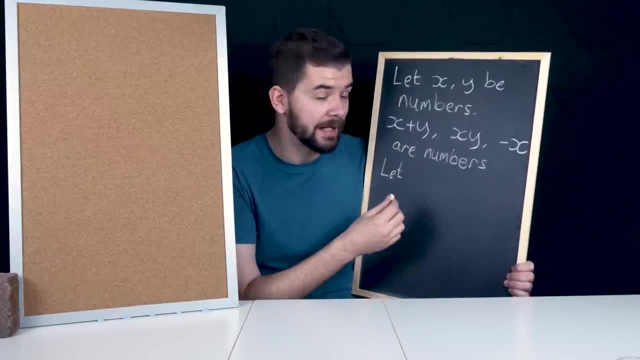 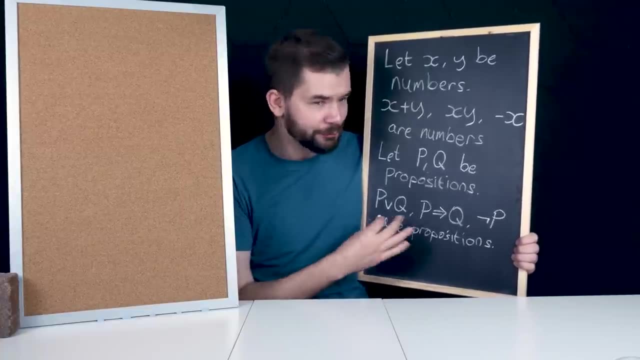 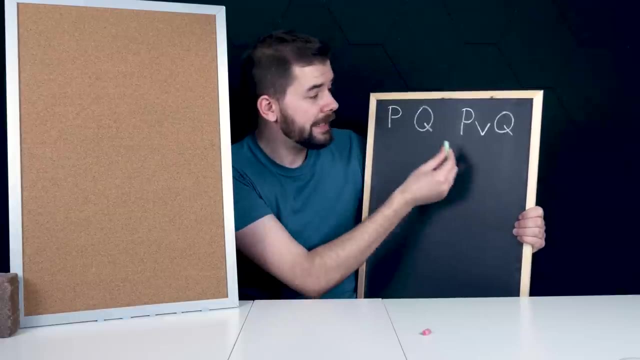 I can also do the same with propositions. So if I let say be propositions, then I have some operations I can do to combine these to make new propositions. So let's break down what these symbols mean. The first one is or, So P or Q is true whenever P is. 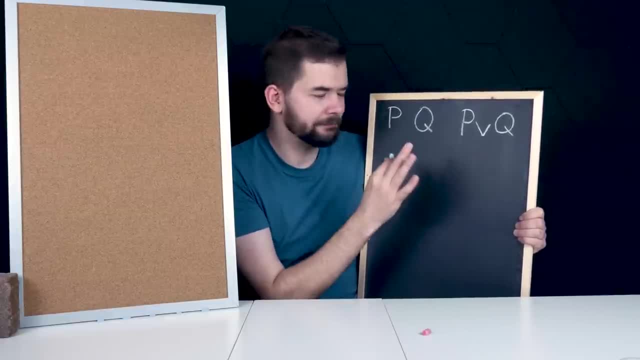 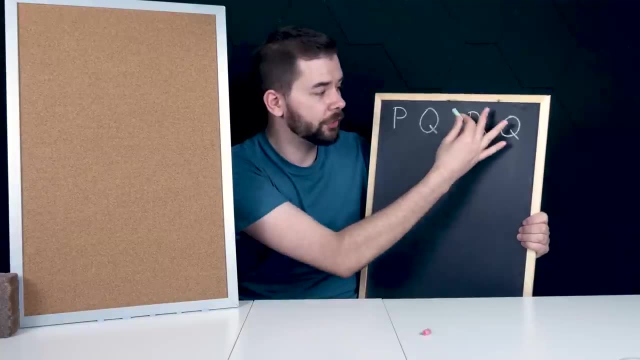 true, Q is true, or if they're both true, It's only false when both P and Q are false, And I can actually draw up all the combinations of true and false here to show you exactly when this is true in something that's called a truth table. So let's look at an example. If I say X is greater, 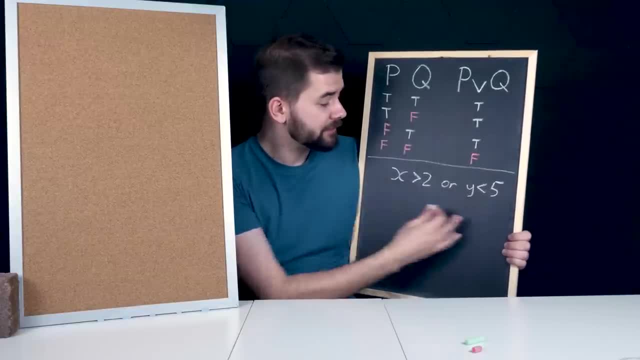 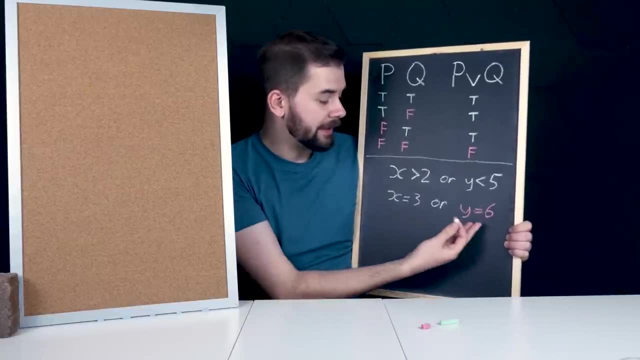 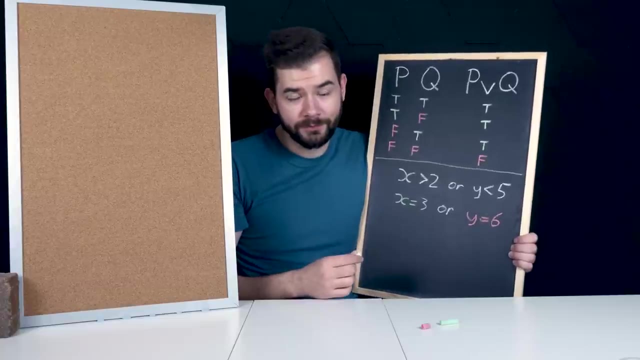 than two or Y is less than five, then this overall statement is true. if one or both of these conditions hold. So let's look at the case where X is three and Y is six, Then it is true that either X is greater than two or Y is less than five, because one of them holds Or is in contrast to. 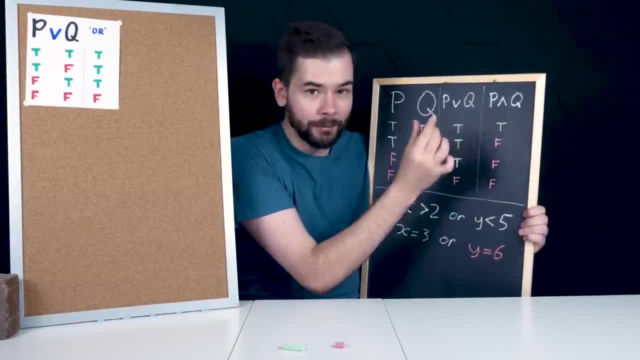 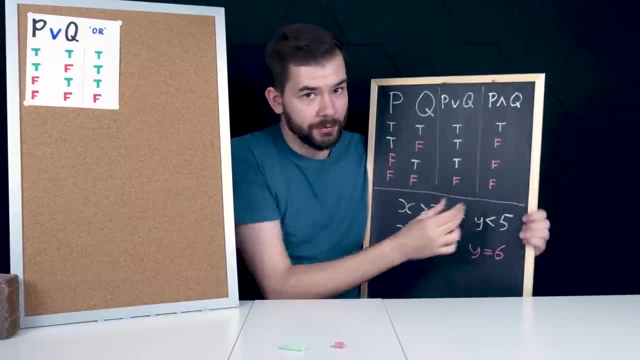 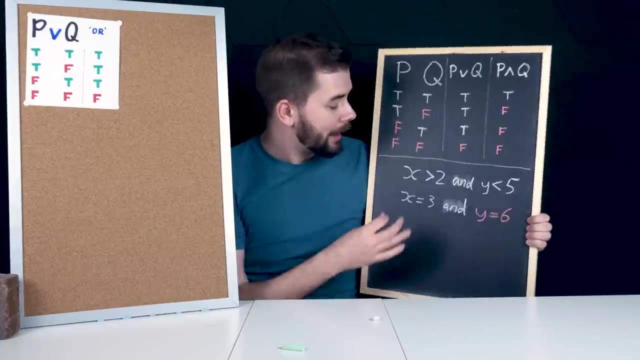 this one here which says P and Q. So the proposition P and Q is true if both P and Q are true and false otherwise. So if I go back to this earlier example and change this from an or to an- and now I'm saying X is 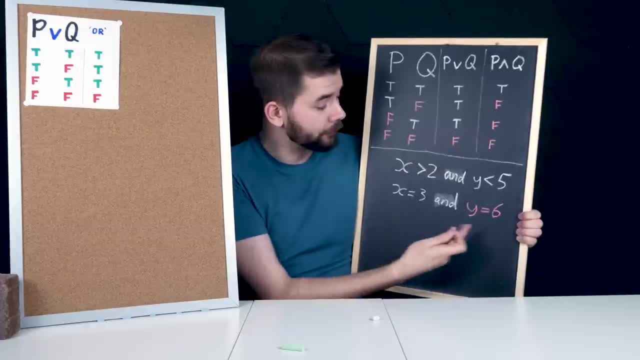 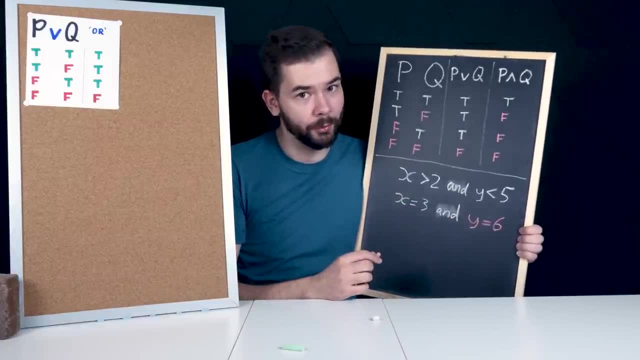 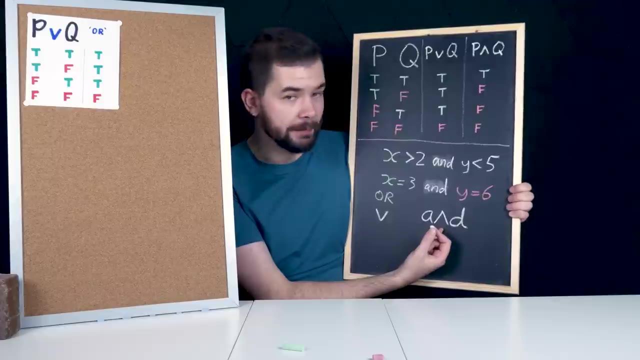 greater than two and Y is less than five. this overall statement with these numbers is now false, because it requires both of the conditions to be satisfied in order to be true overall. Now, it's common in symbolic logic to use a V-shaped symbol for or and an inverted V-shape for and, And. this 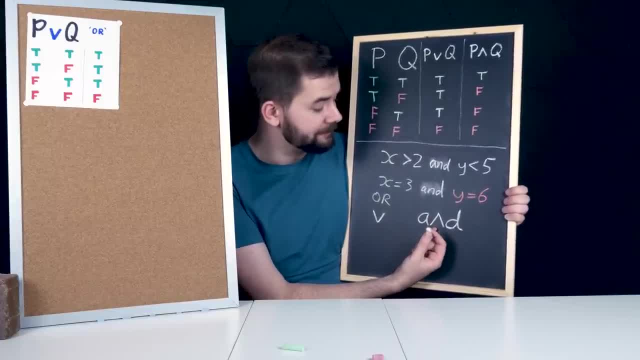 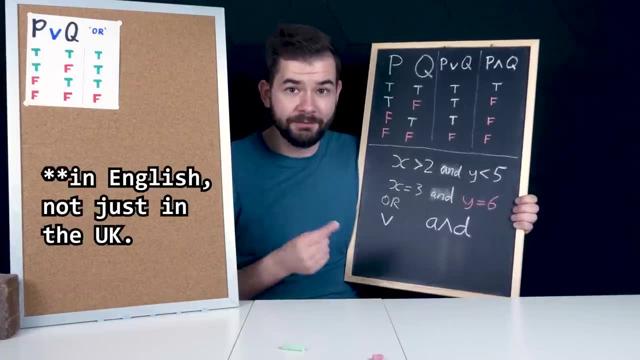 is my personal way of remembering, which is which The inverted V looks like the letter N in and And. in fact, in the UK it's common to use N as an abbreviation for and in terms like fish and chips. Or maybe that's just up north where none of us 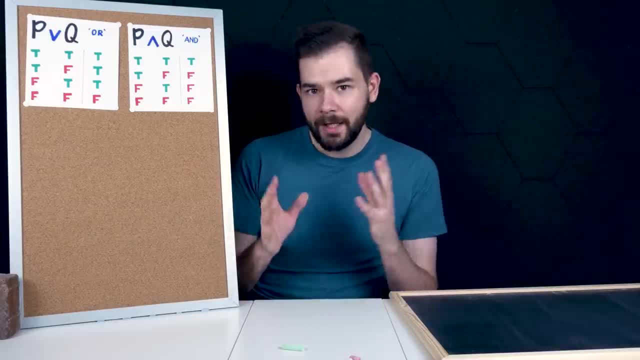 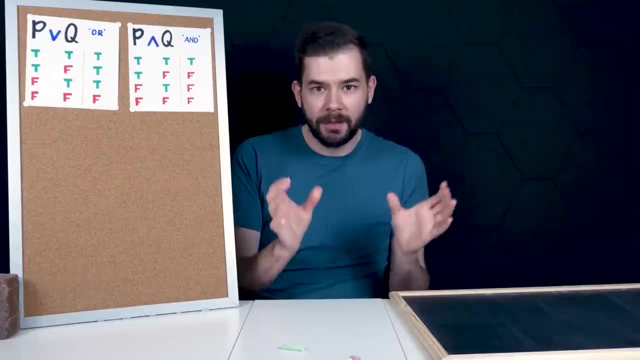 talk proper Now. these should align with your intuition. If I made a statement like the bus was late and it was raining, then your mind automatically paints a picture of both conditions: Me stood in the rain and mildly upset that the bus hasn't arrived yet. Or, if you know me personally, 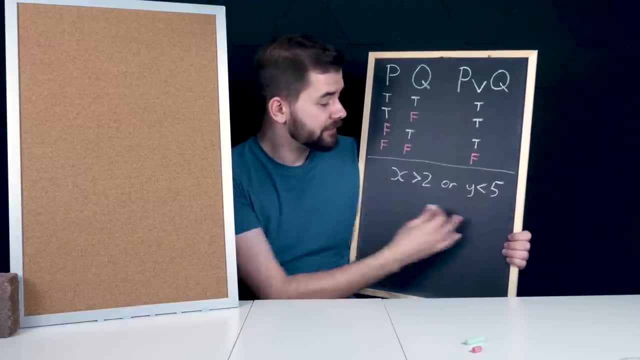 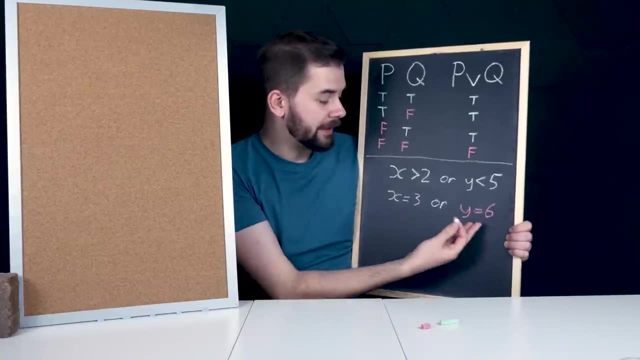 than 2 or Y is less than 5,, then this overall statement is true if one or both of these conditions hold. So let's look at the case where X is 3 and Y is 6. Then it is true that either X is: 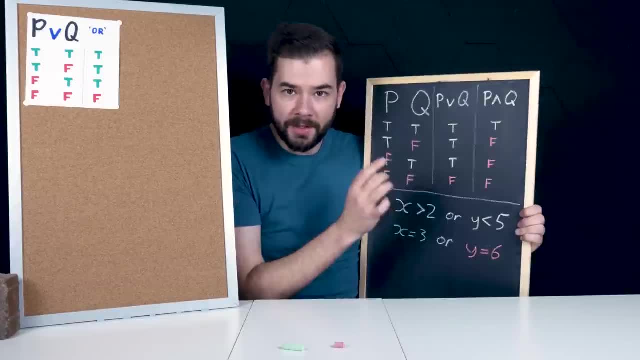 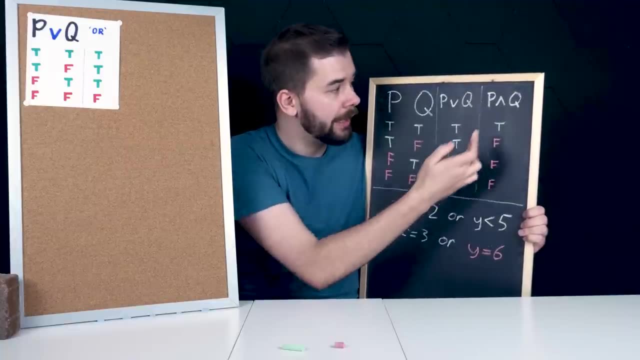 greater than 2 or Y is less than 5 because one of them holds Or is in contrast to this one here which says P and Q. So the proposition P and Q is true if both P and Q are true and false otherwise. 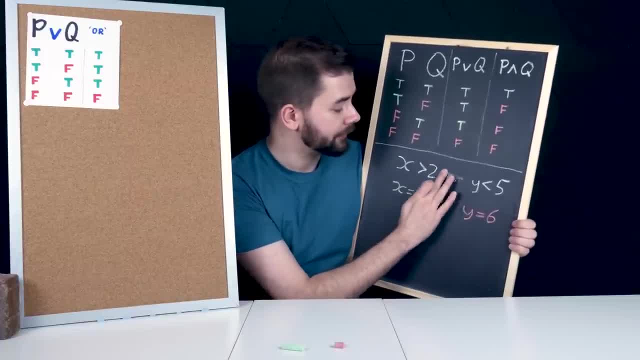 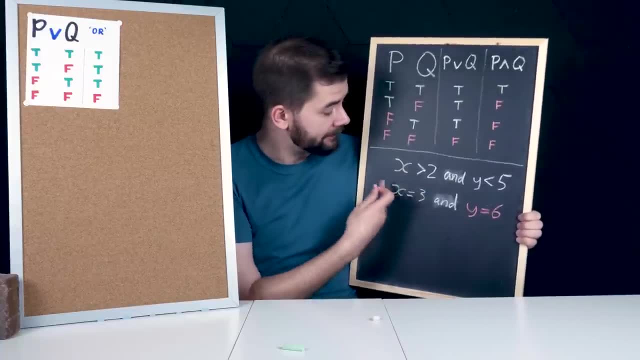 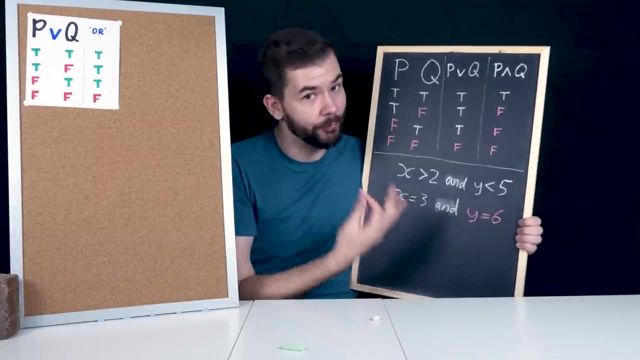 So if I go back to this earlier example and change this from an or to an, and now I'm saying X is greater than 2 and Y is less than 5, this overall statement with these numbers is now false, because it requires both of the conditions to be satisfied in order to be true overall. Now, it's common in 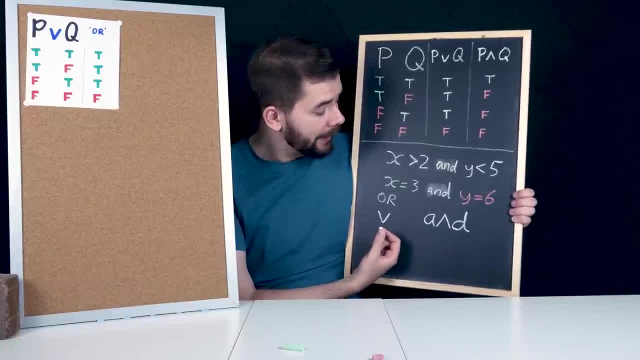 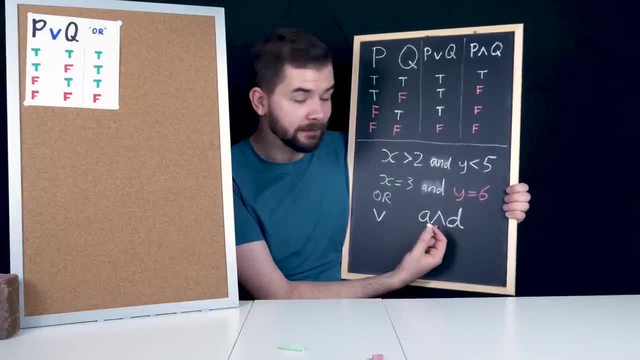 symbolic logic to use a V-shaped symbol for or and an inverted V-shape for and, And. this is my personal way of remembering, which is which The inverted V looks like the letter N in and And. in fact, in the UK it's common to use N as an. 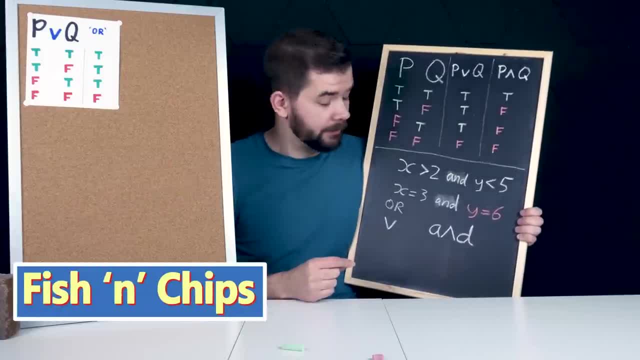 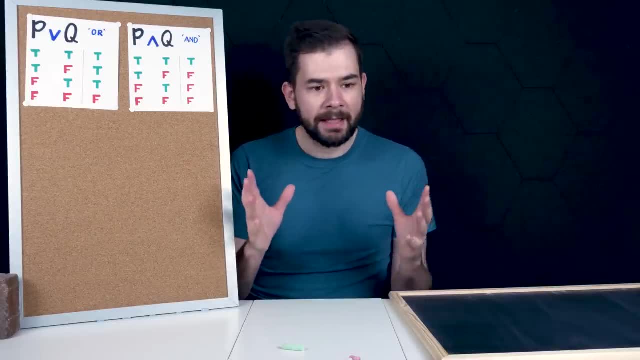 abbreviation for and in terms like fish and chips. Or maybe that's just up north where none of us talk proper. Now, these should align with your intuition. If I made a statement like the bus was late and it was raining, then your mind automatically paints a picture of both conditions. 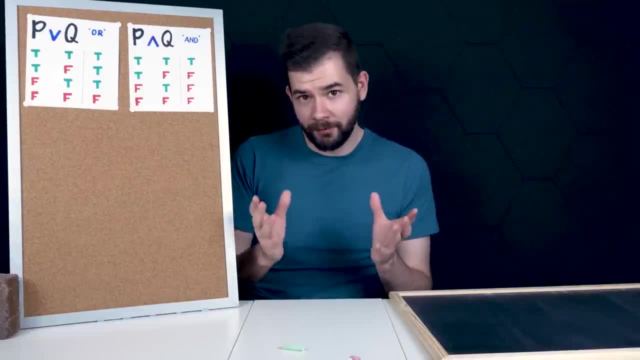 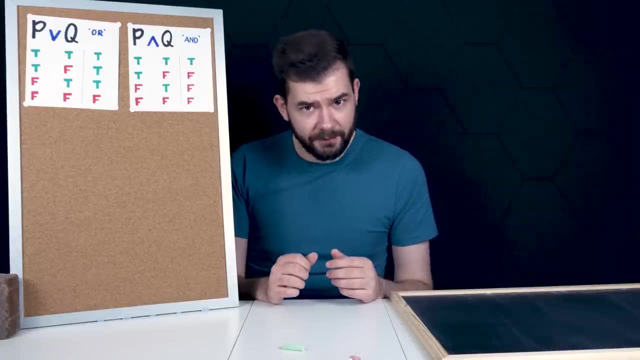 Me stood in the rain and mildly upset that the bus hasn't arrived yet. Or if you know me personally, you're picturing me more than a little mildly upset at the current state of UK public transportation services. An or should align with your intuition as well If I said I'd like to drink tea or I'd 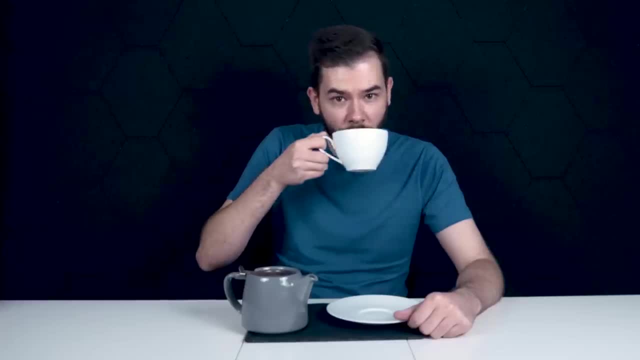 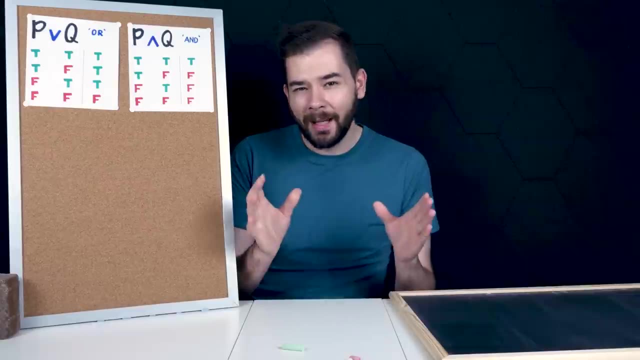 like to drink coffee, then you suppose that I'd be happy drinking tea, that I'd be happy drinking coffee, that I'd be happy with both drinks, though probably not in simultaneity. What might perturb your intuition a little bit is that an or statement is true if one of the input statements is true. 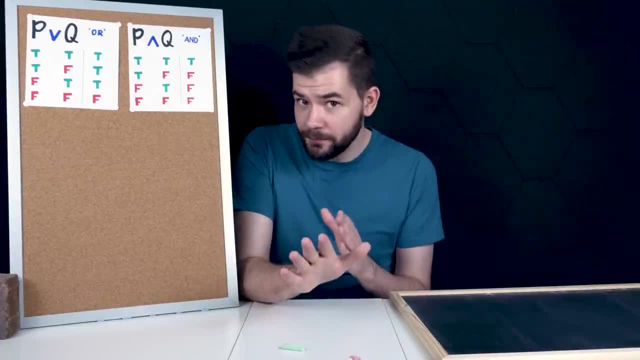 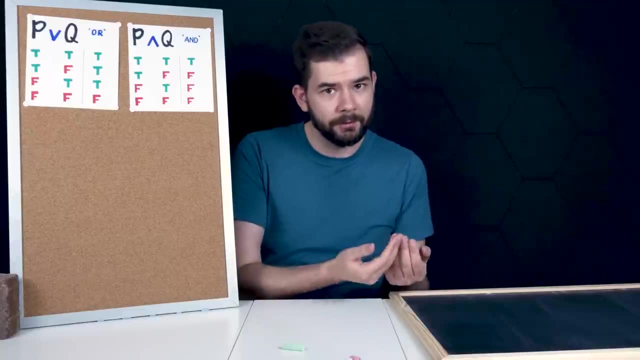 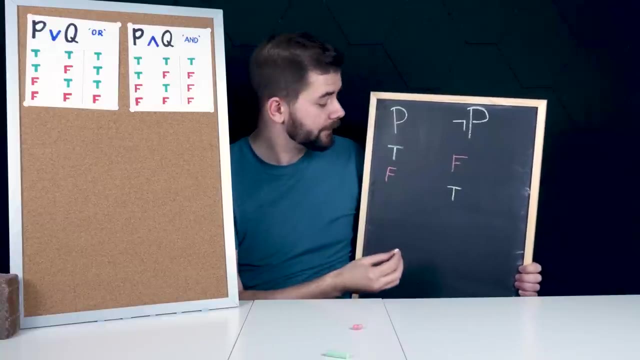 and we don't really care which one. A classic- and I use the term generously, joke- is a logician- gives birth and is asked: is it a boy or a girl? And they respond yes. Another logical operator is not or negation. So if p is a proposition, 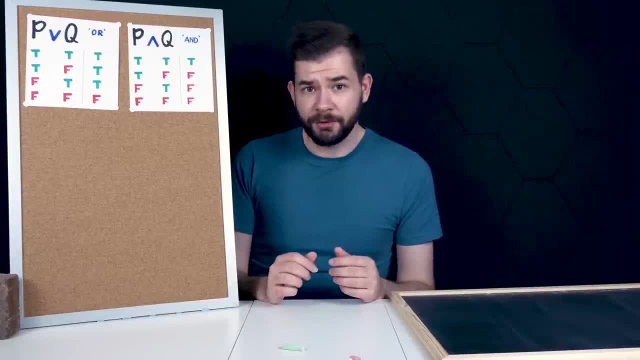 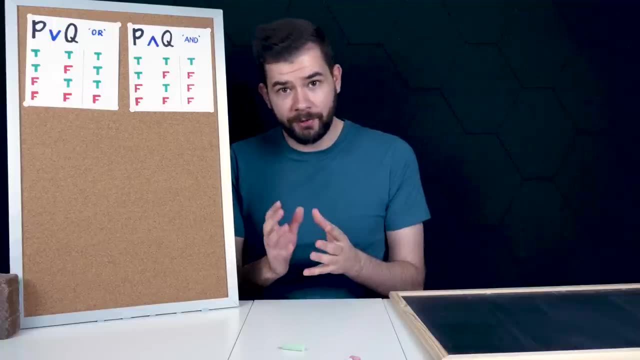 you're picturing me more than a little mildly upset at the current state of UK public transportation services, And or should align with your intuition as well. If I said I'd like to drink tea or I'd like to drink coffee, then you suppose that I'd be happy drinking tea, that I'd be happy drinking. 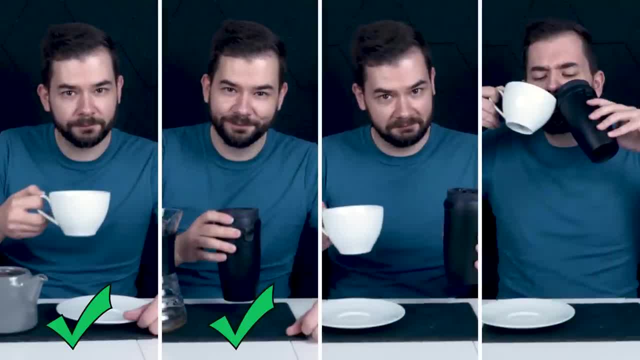 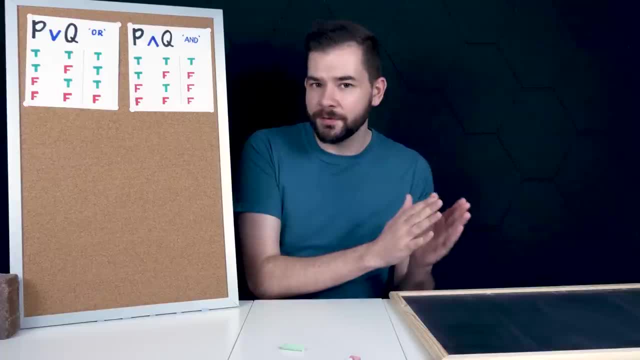 coffee that I'd be happy with both drinks, though probably not in simultaneity. What might perturb your intuition a little bit is that an or statement is true. if one of the input statements is true- And we don't really care which one- A classic. 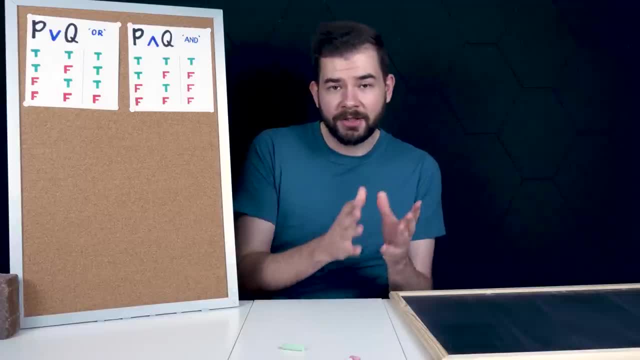 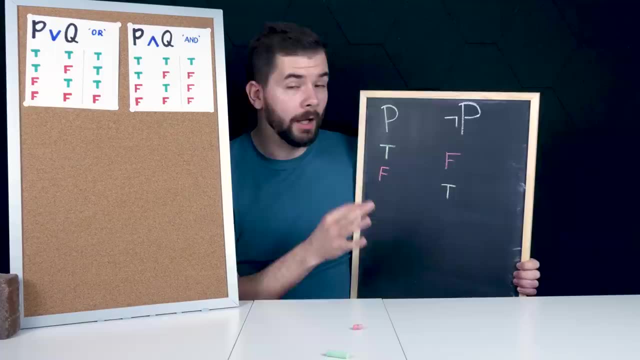 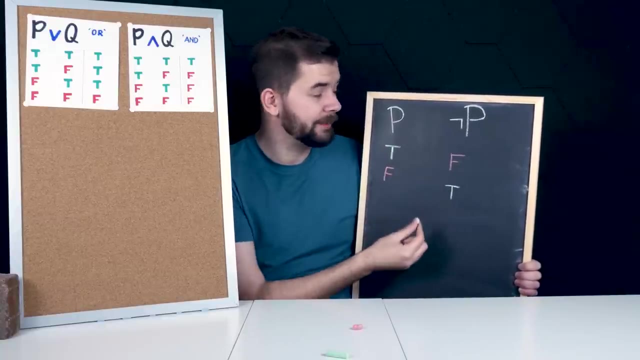 and I use the term generously joke is: a logician gives birth and is asked: is it a boy or a girl? And they respond yes. Another logical operator is not or negation. So if P is a proposition, then not P is true exactly when P is false and false exactly when 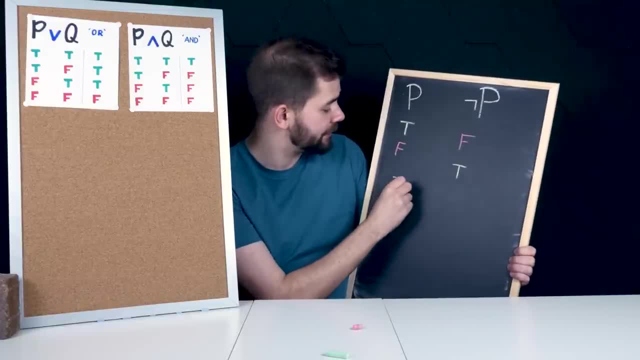 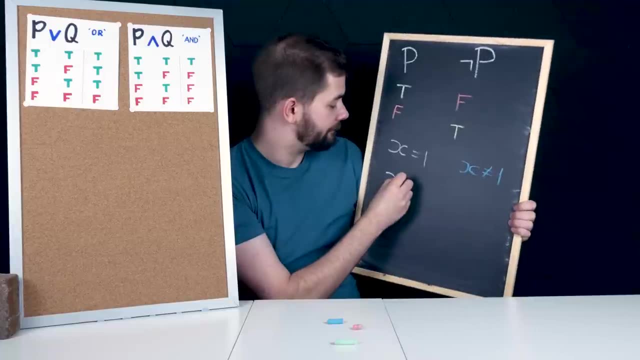 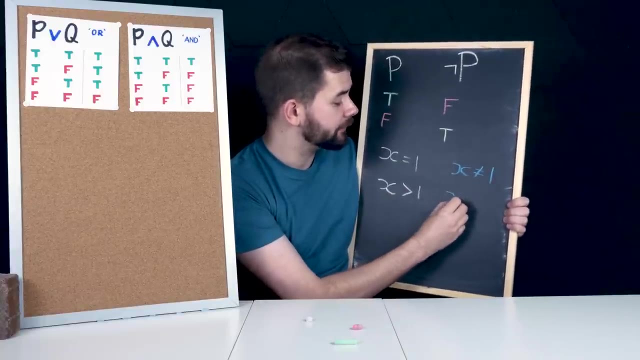 P is true. So, for example, if P is the proposition X is equal to one, then not P would be the proposition X is not equal to one. If P is the proposition X is greater than one, then not. P is the proposition X is not greater than one. And of course the usual way to say this is: X is less than. 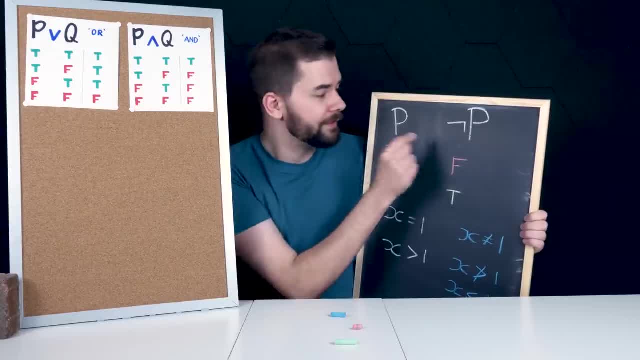 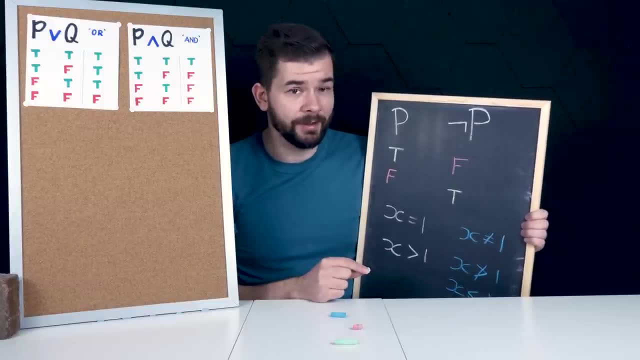 or equal to one. Don't forget about the or equal to. We use this symbol for negation and I have no idea why. Maybe because whoever first used it felt really sorry for that one key on the keyboard that's used for literally nothing else. 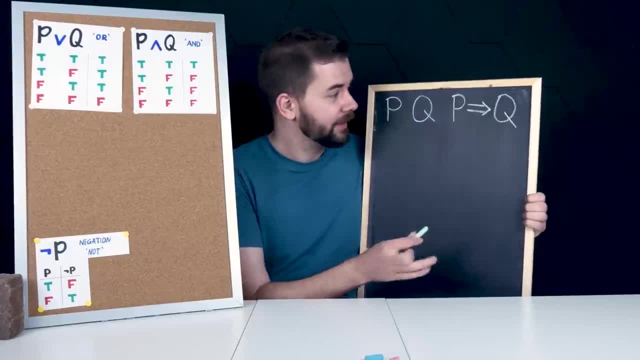 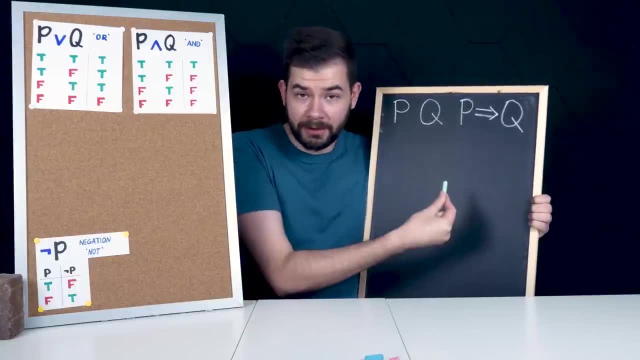 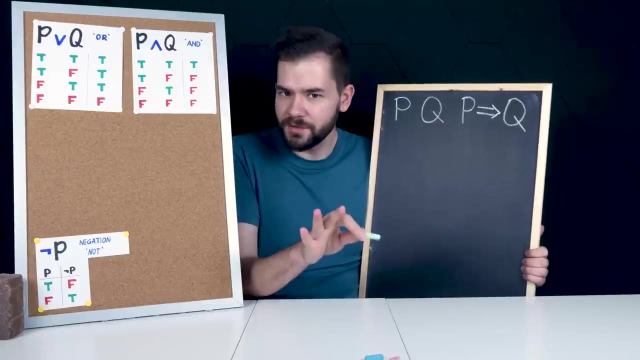 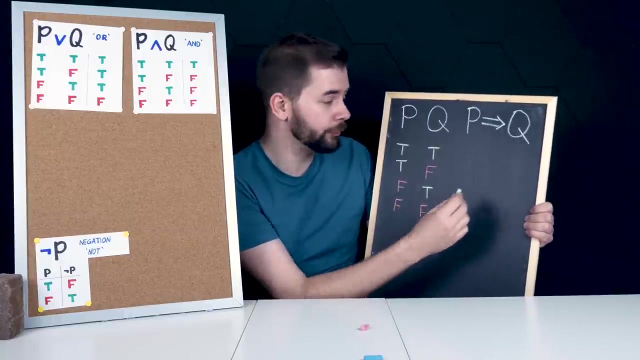 So P implies Q. we often read: if P, then Q. Now brace yourself, because the first time you see this it might look a bit strange, but it does make sense, I promise. So P implies Q is true whenever P and Q are both true or when P and Q are both true. 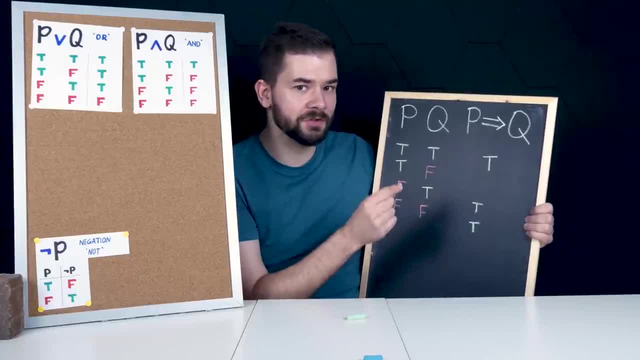 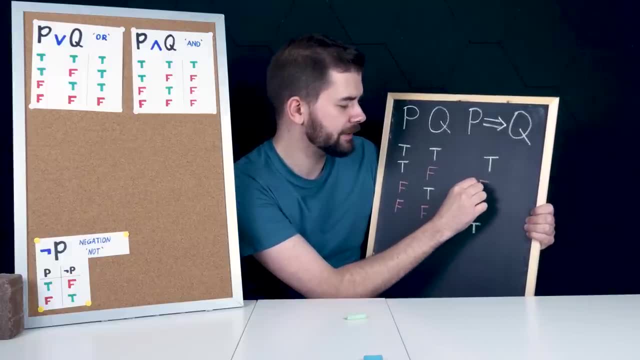 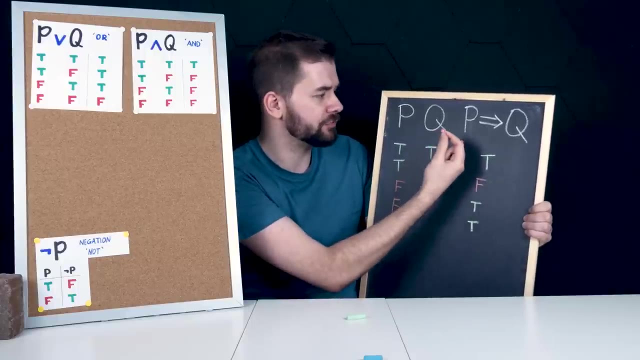 The only situation in which P implies Q is false is if P is true yet Q is false, And hopefully that should feel intuitive, because it doesn't really make sense for Q to follow logically from P if we can possibly have a situation in which P is true yet Q is still false. Now this might seem. 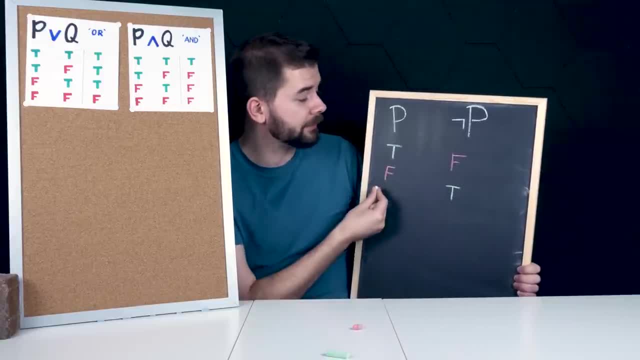 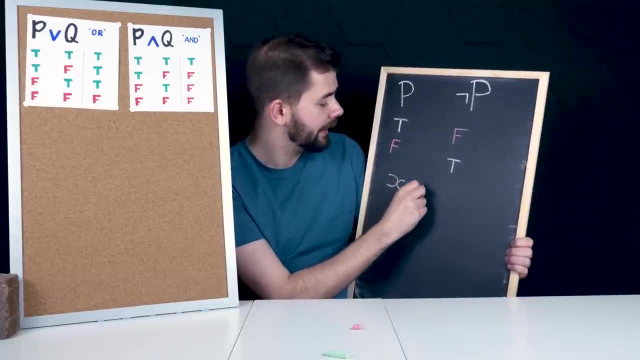 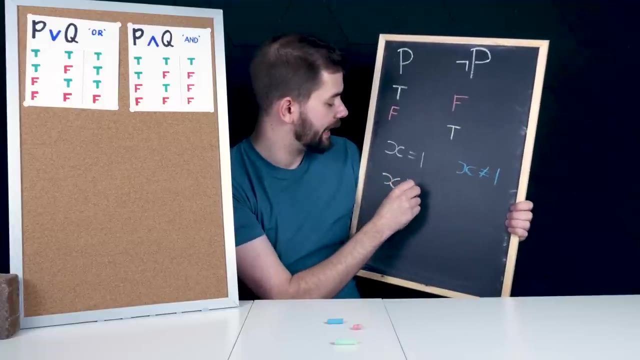 then not p is true exactly when p is false and false exactly when p is true. So, for example, if p is the proposition x is equal to one, then not p would be. the proposition x is not equal to one. If p is the proposition x is greater than one, then not p is the proposition. 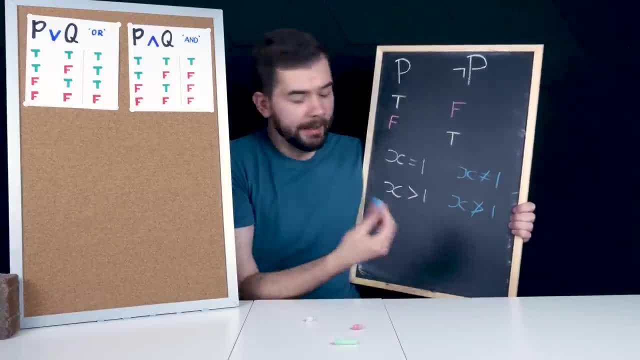 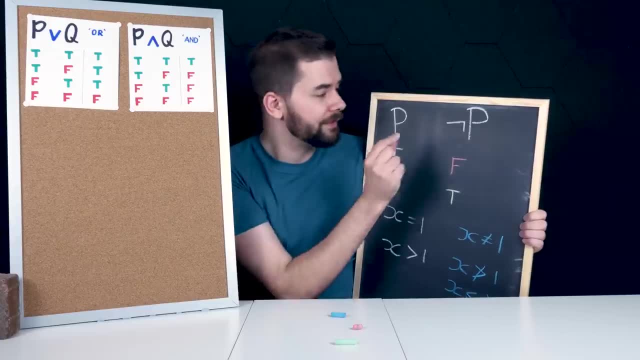 x is not greater than one, And, of course, the usual way to say this is: x is less than or equal to one. Don't forget about the or equal to. We use this symbol for negation and I have no idea why, Maybe. 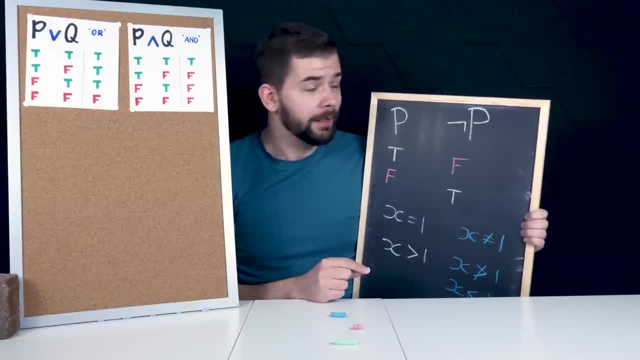 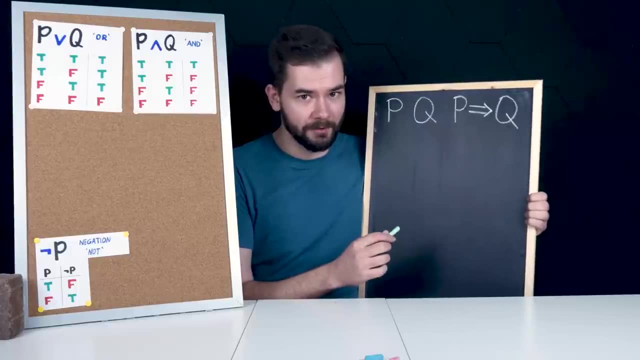 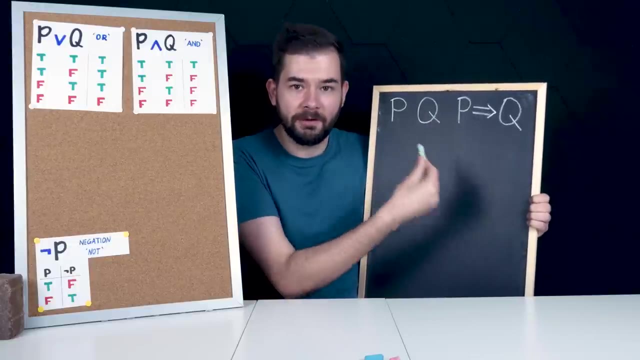 because whoever first used it felt really sorry for that one key on the keyboard that's used for literally nothing else. Okay, final logical connective, and one that's crucial to the study of mathematics, and that is implies: This encodes the notion that one statement follows logically from another. So p implies q. 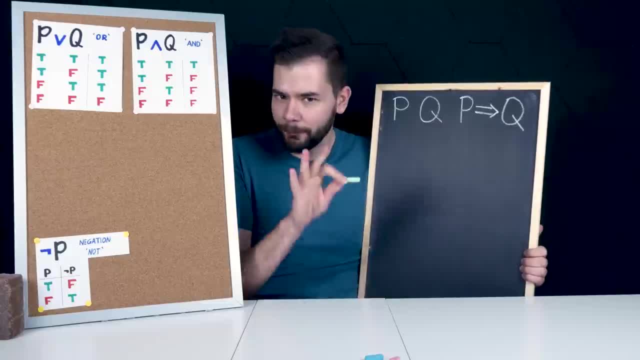 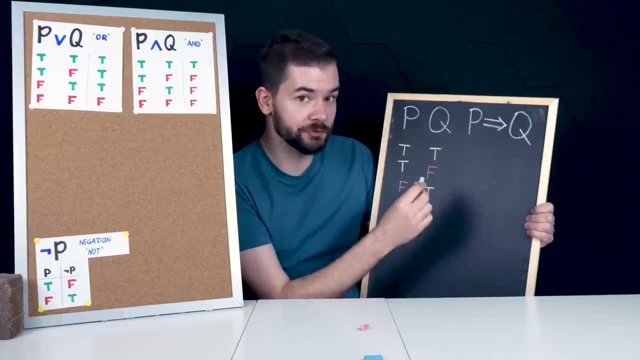 we often read: if p, then q. Now brace yourself, because the first time you see this it might look a bit strange, but it does make sense, I promise. So p implies q is true whenever p and q are both true, or? 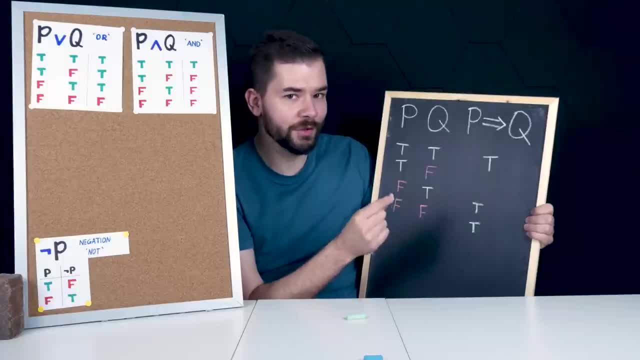 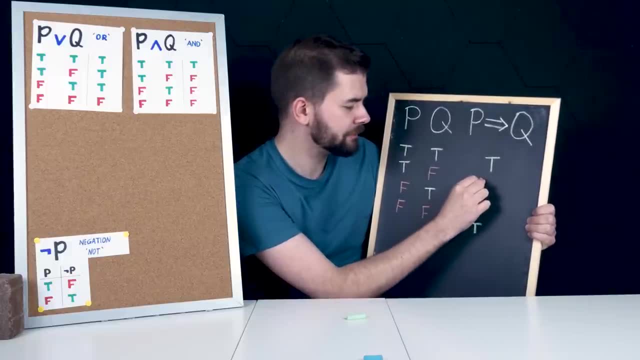 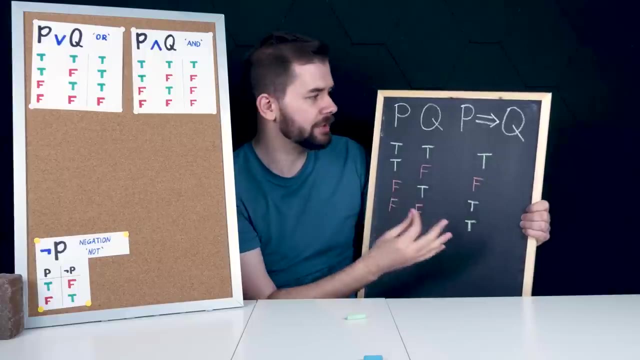 when p is false. The only situation in which p implies q is false is if p is true yet q is false, And hopefully that should feel intuitive, because it doesn't really make sense for q to follow logically from p if we can possibly have a situation in which p is true yet q is still false. Now this might. 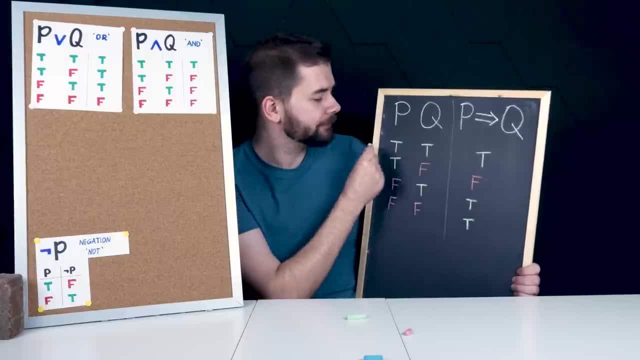 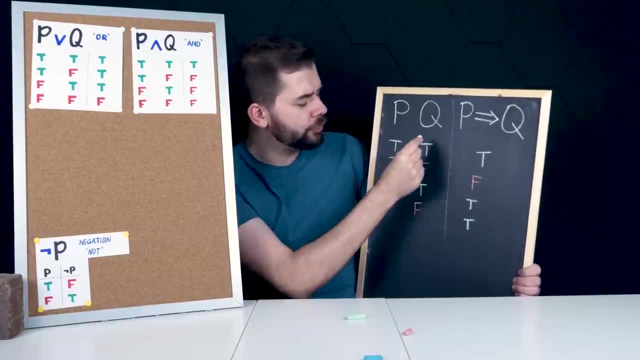 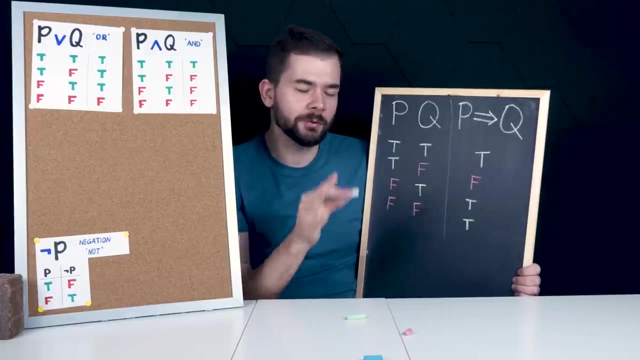 seem a little bit strange. So usually people are comfortable with the idea that if p implies q, then this top row definitely should hold. But surely q couldn't be true even when p is false. you know if this is supposed to be following logically. But let me convince you a few different ways why this is indeed the case. 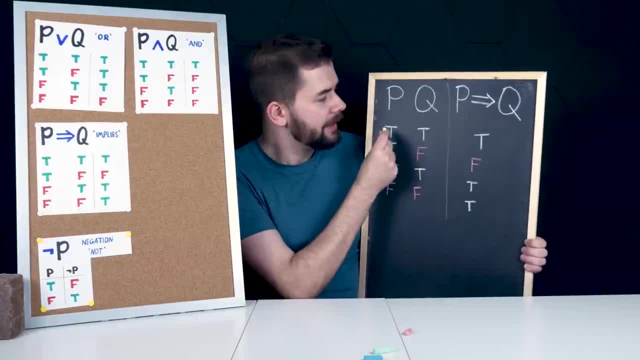 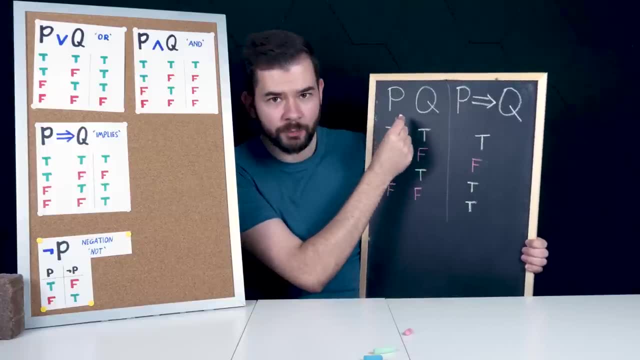 One way to think about it is this: If p is true, then q should automatically be true if q follows logically from p. But in the situations where p is false, we can't conclude anything about q. Let me show you an example. Consider this: Greg is a candidate thatadeshitearscom. 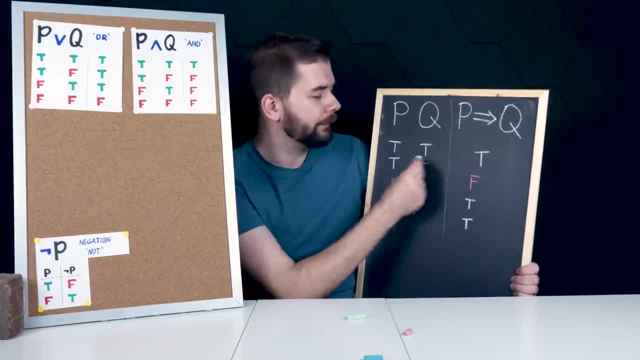 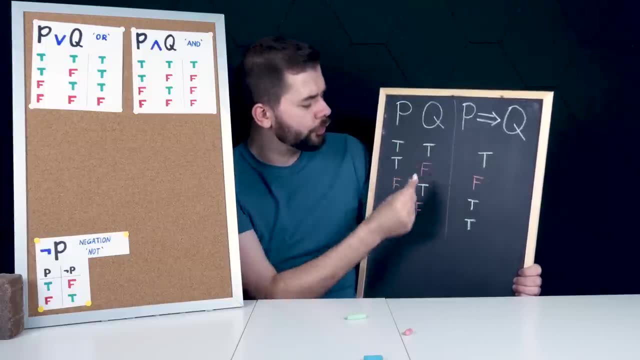 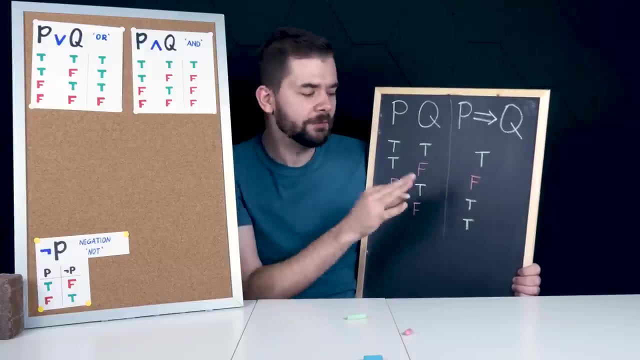 a little bit strange. So usually people are comfortable with the idea that if P implies Q, then this top row definitely should hold. but surely Q couldn't be true even when P is false. You know if this is supposed to be following logically. But let me convince you a few different ways why this is indeed the case. 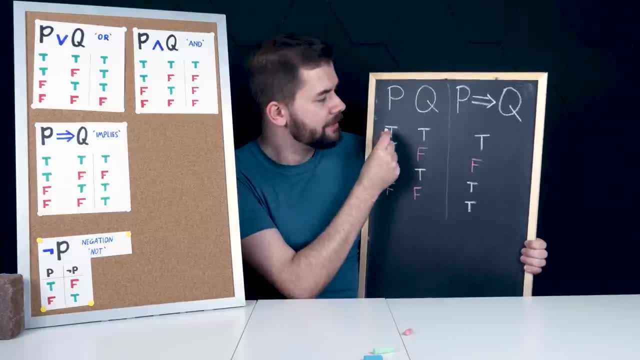 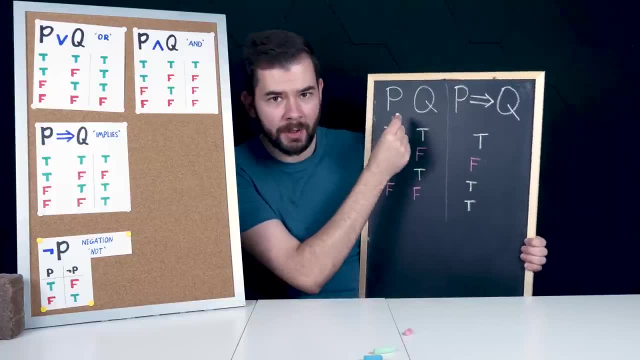 One way to think about it is this: If P is true, then Q should automatically be true if Q follows logically from P. But in the situations where P is false, we can't conclude anything about Q. Let me show you an example. Consider this. 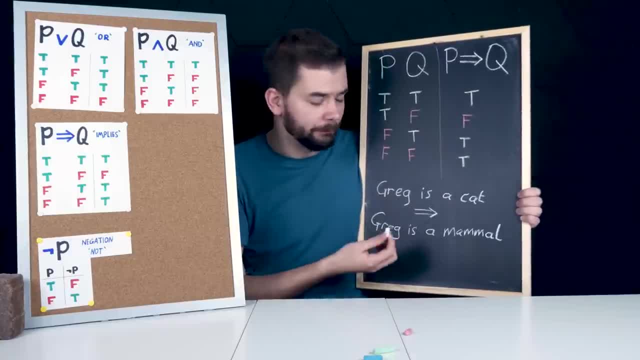 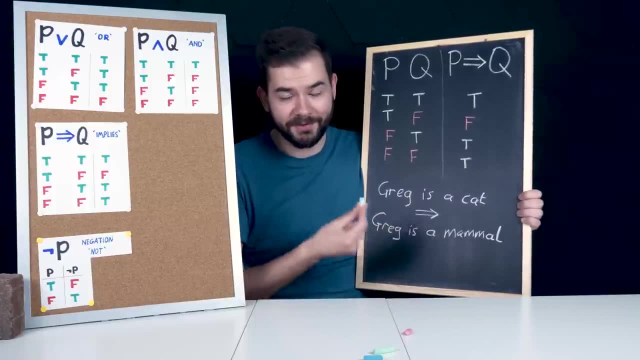 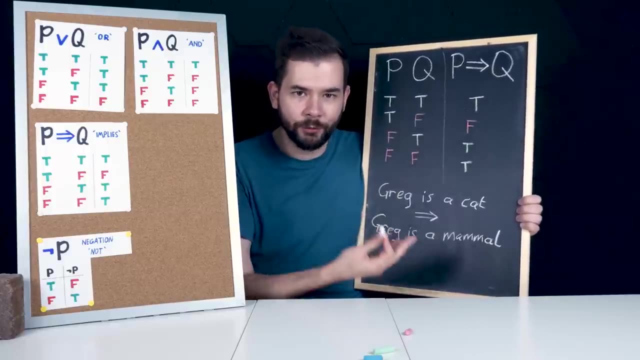 A cat implies Greg is a mammal. That seems to follow, because if this first statement is true and Greg is a cat, then we know it's definitely a mammal, because every cat is a mammal. But think about these situations here. Imagine if Greg is not a cat. Well then we can't conclude anything. 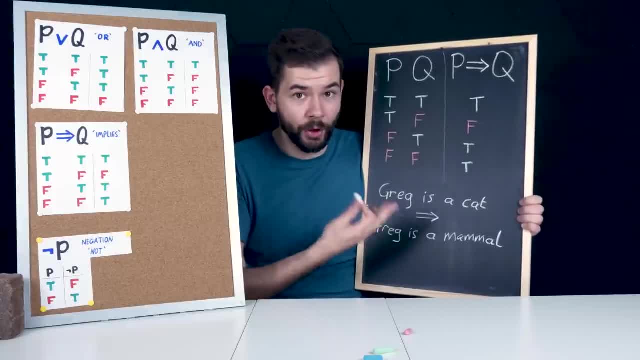 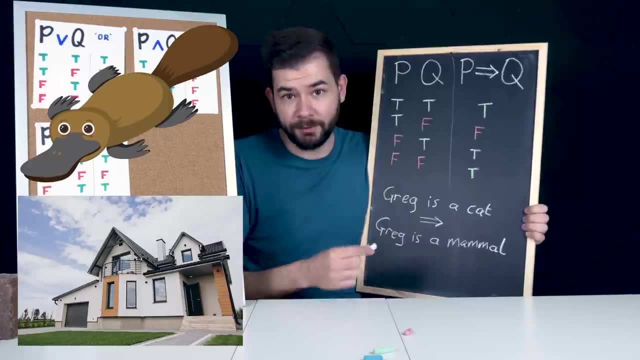 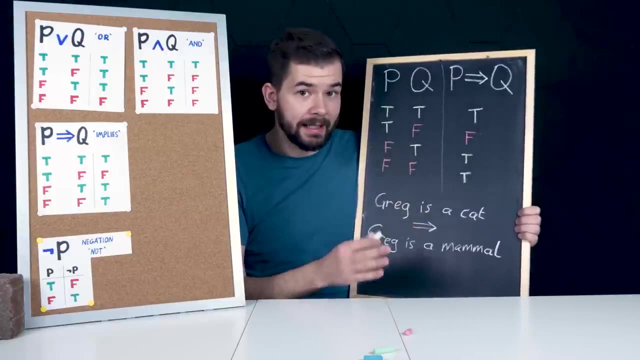 about its nature as a mammal. Greg could be a non-cat non-mammal like an octopus or a house, or Greg could be a non-cat mammal like a platypus or a house. It's a one-way implication. Cat implies mammal, but non-cat doesn't necessarily imply. 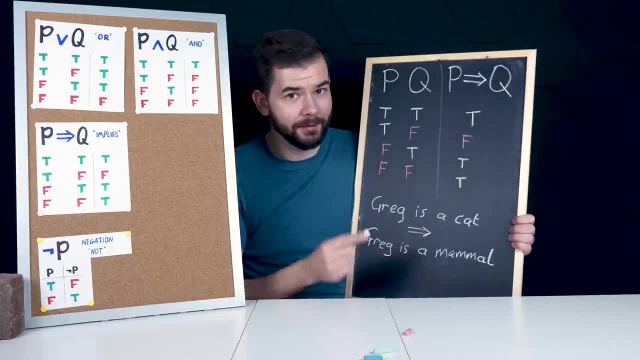 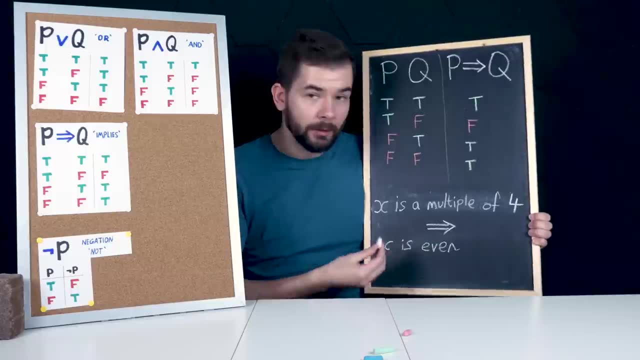 non-mammal. So these second two situations are still valid. A mathematical example might be something like this: X is a multiple of four implies X is even. Well, that definitely follows, because every multiple of four is even. But if X is not a, 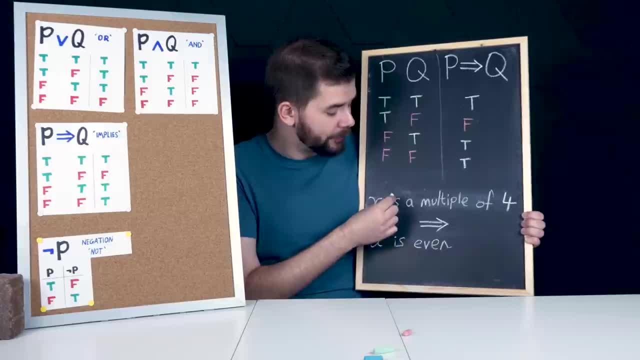 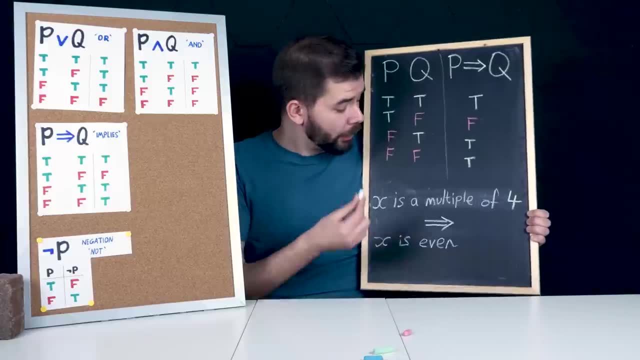 multiple of four. so this first statement is false, then we can't say anything about X's parity. X could be not a multiple of four, but it could be a parity. So if X is not a multiple of four and be odd like five or seven, or it could be not a multiple of four and still even like two, 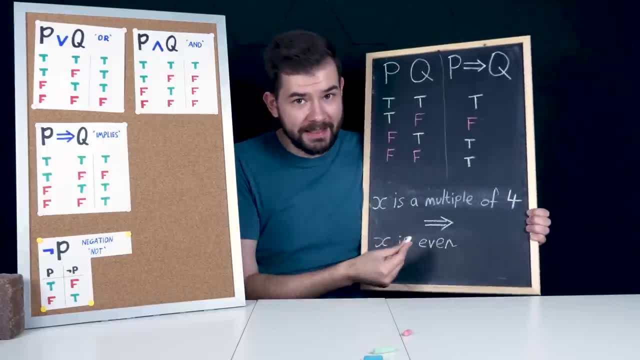 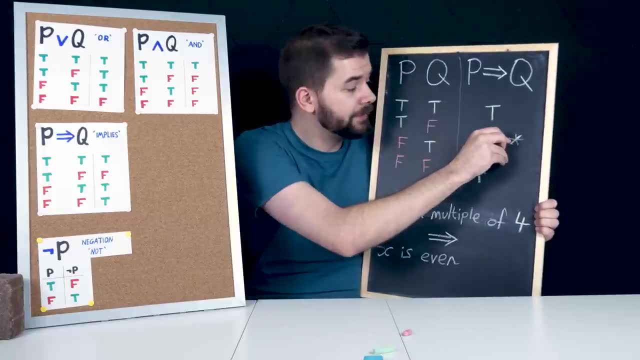 or ten. So multiple of four implies even, but not multiple of four doesn't imply odd or doesn't imply even. Both situations are valid And remember, the only situations in which this implication is false is if the first statement is true and the second statement is false. 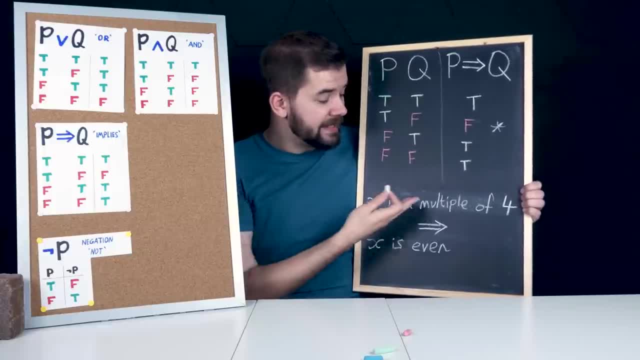 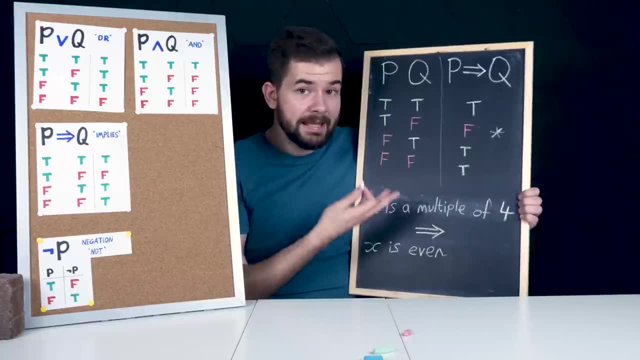 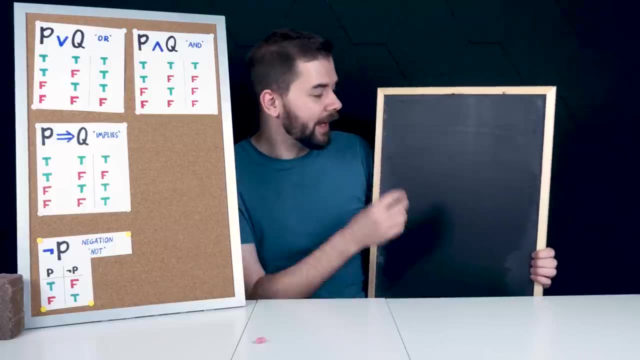 In our examples that would mean something like X is a multiple of four, yet X is not Even Absurd. Or in our earlier example, Greg being a cat, yet not a mammal- Just as absurd. A visual way to think about this implication is like this: Imagine this board represents. 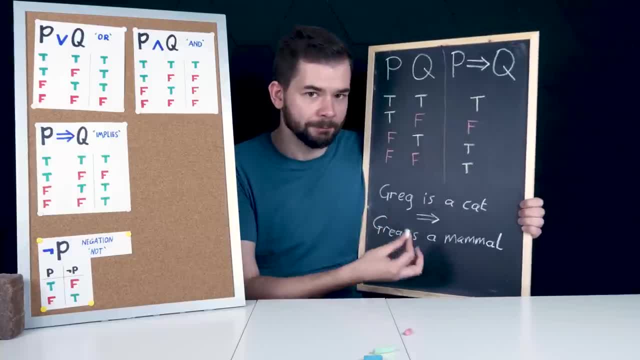 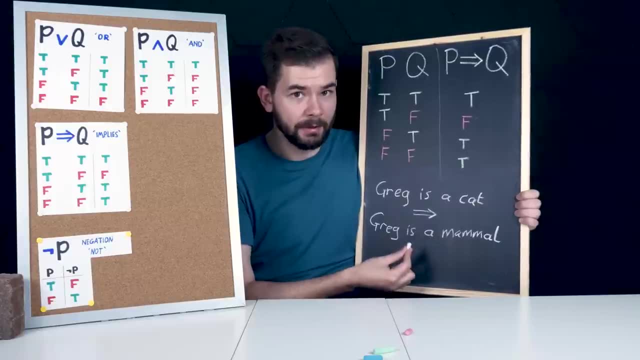 Wahoo, Wahoo, Wahoo, Wahoo, Wahoo, Wahoo is a cat implies greg is a mammal. that seems to follow, because if this first statement is true and greg is a cat, then we know it's definitely a mammal, because every cat is a mammal, but think. 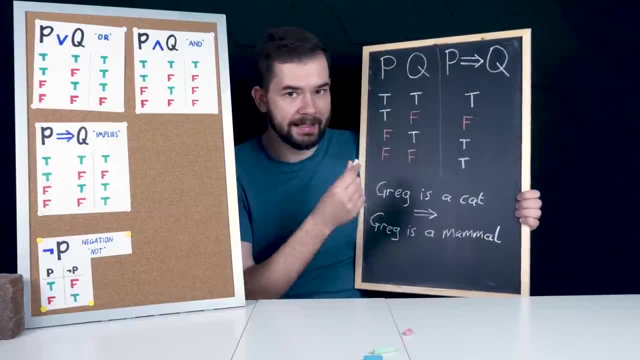 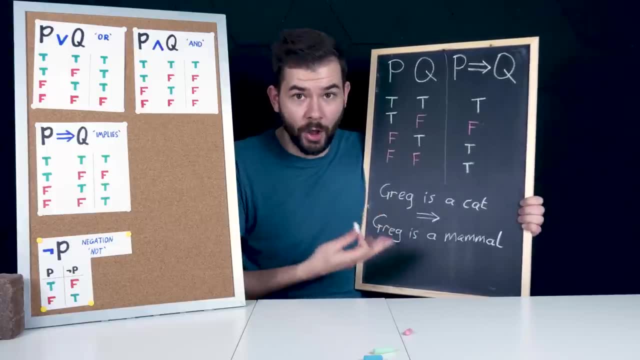 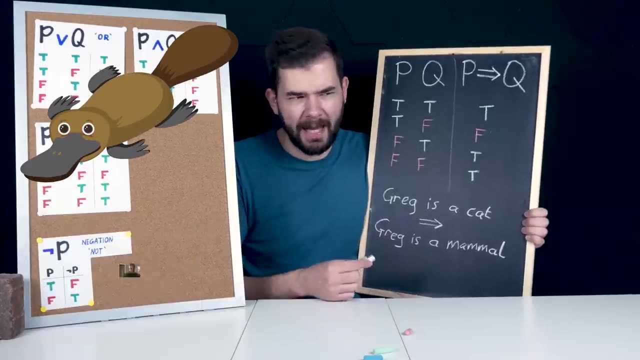 about these situations here. imagine if greg is not a cat. well then we can't conclude anything about its nature as a mammal. greg could be a non-cat, non-mammal like an octopus or a house. or greg could be a non-cat mammal like a platypus or a house. it's a one-way implication. cat implies 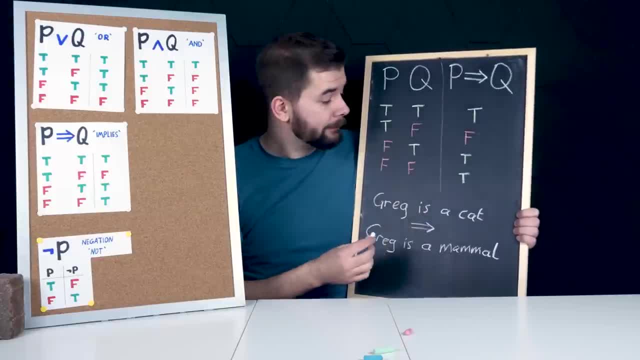 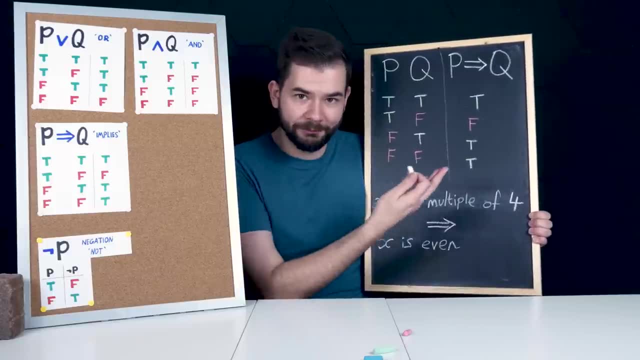 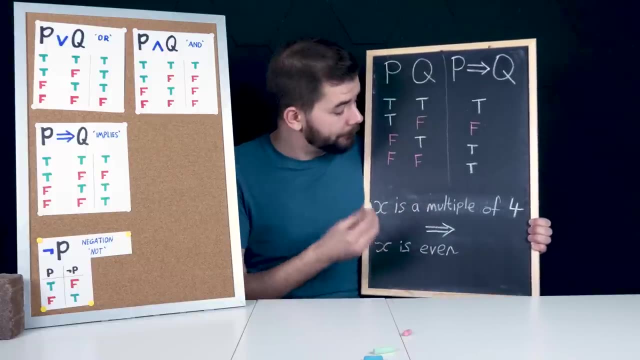 mammal. but non-cat doesn't necessarily imply non-mammal, so these second two situations are still valid. a mathematical example might be something like this: x is a multiple of four implies x is even. well, that definitely follows, because every multiple of four is even. but if x is not a, 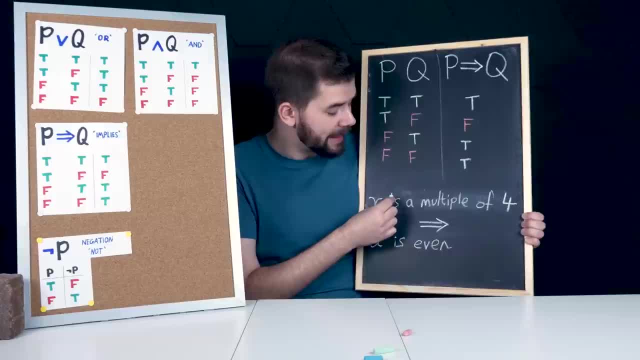 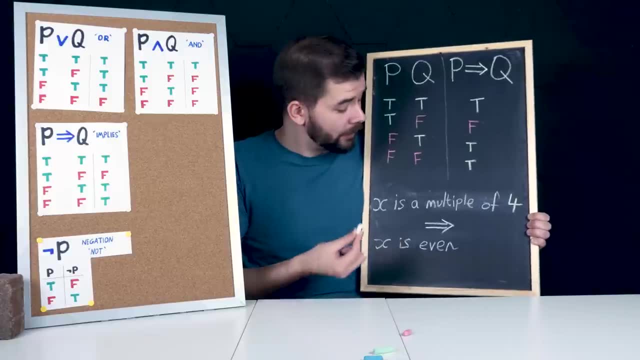 multiple of four. so this first statement is four. then we can't say anything about x's parity. x could be not a multiple of four and be odd like five or seven, or it could be not a multiple of four and still even like two or ten. so 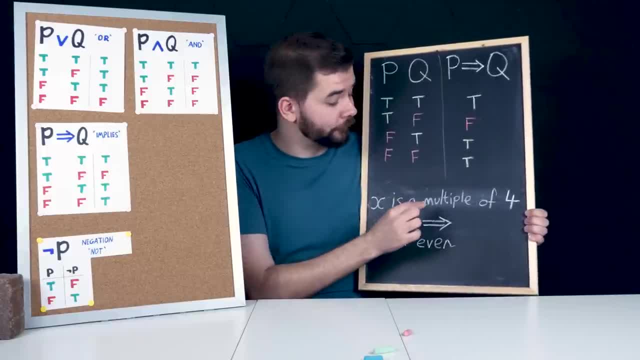 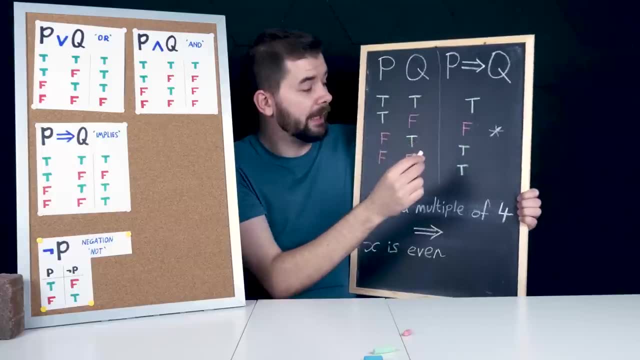 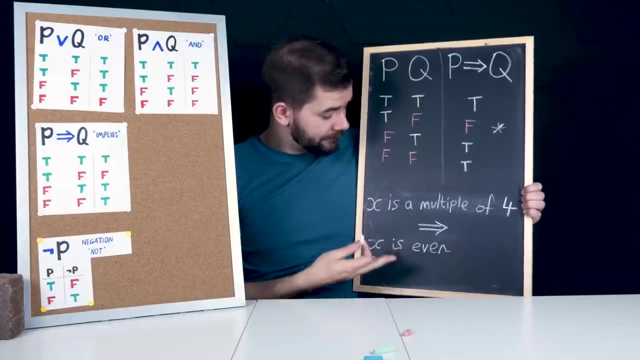 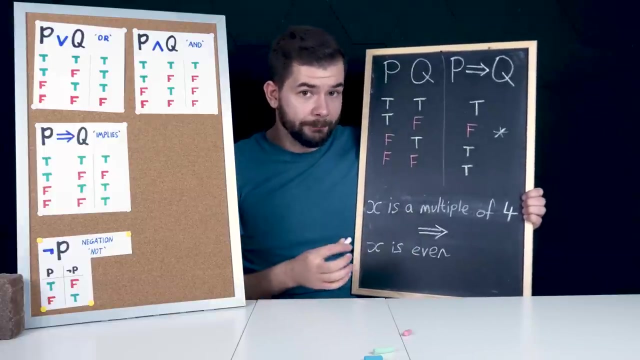 multiple of four implies even, but not multiple of four doesn't imply odd or doesn't imply even. both situations are valid and remember, the only situations in which this implication is false is if the first statement is true and the second statement is false. in our examples would mean something like x is a multiple of four, yet x is not even absurd. or in our earlier example. 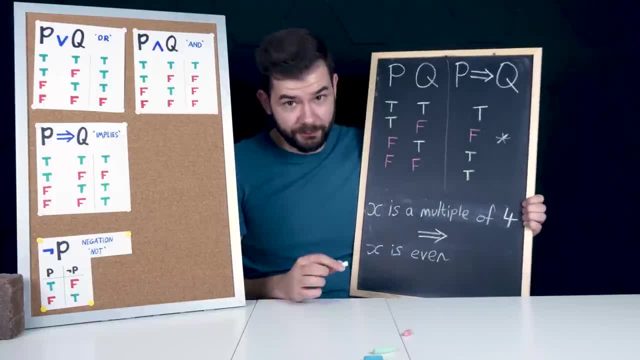 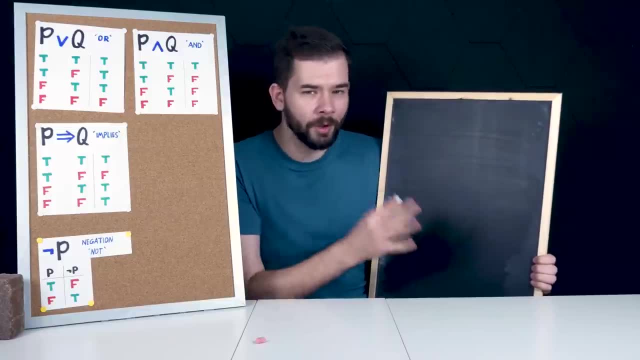 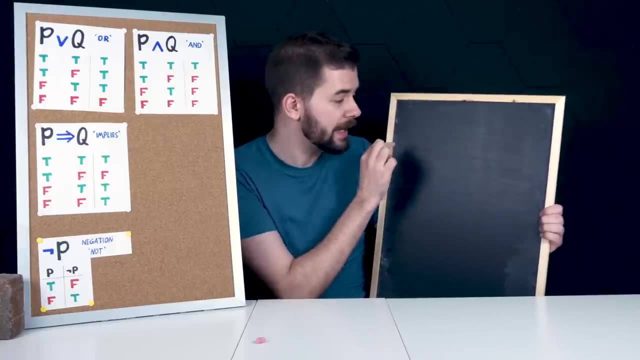 greg being a cat, yet not a mammal. just as absurd a visual way to think about this implication is like this: imagine: this board represents all possible situations, so everything that could possibly happen or ever happen, or will happen or has happened is represented by some position on. 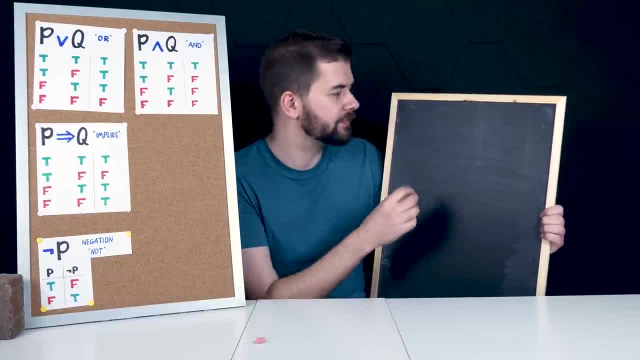 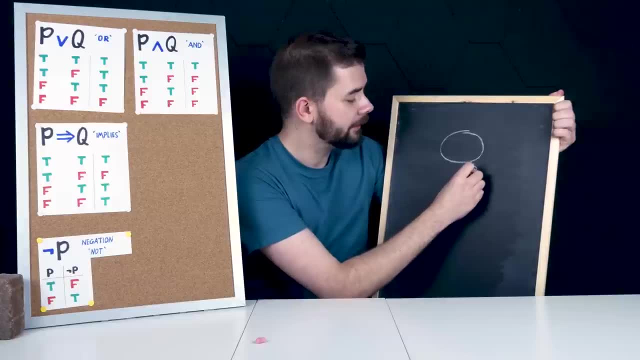 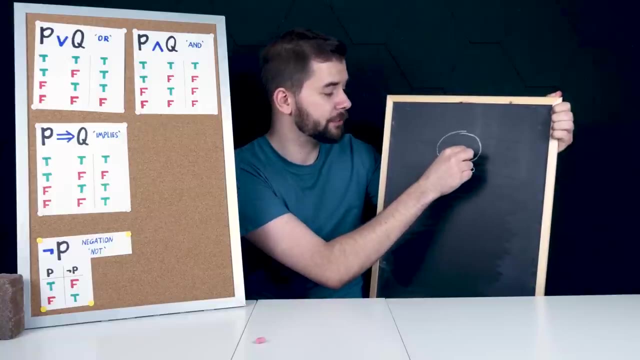 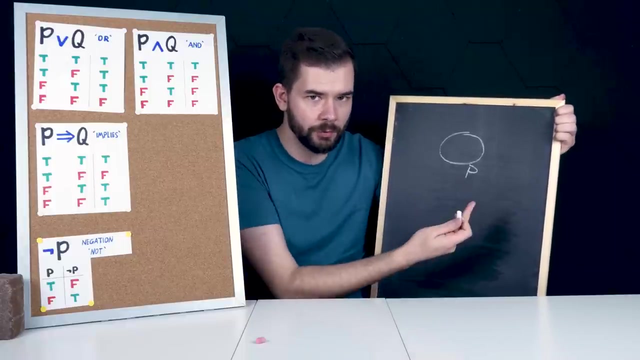 this board. it'll make sense in a minute, trust me. uh, so this board represents all situations, and inside this blob is the situations in which p is true. so if this is a situation out here, p is false. if this is a situation inside this p space, then p is true. now let's think about what it looks like if p implies q. so whenever p is true, 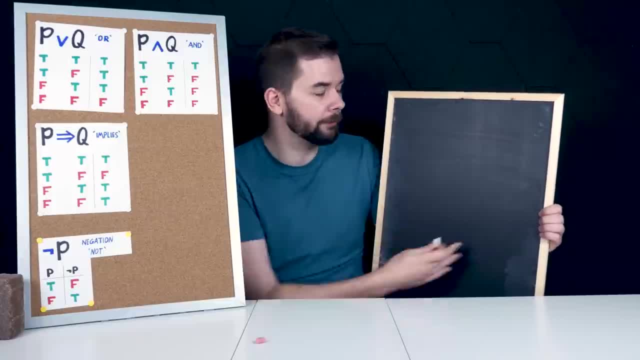 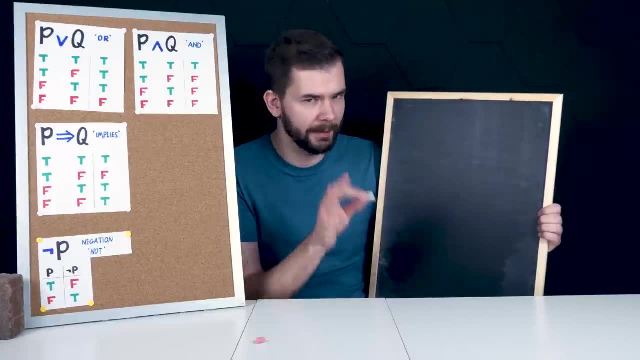 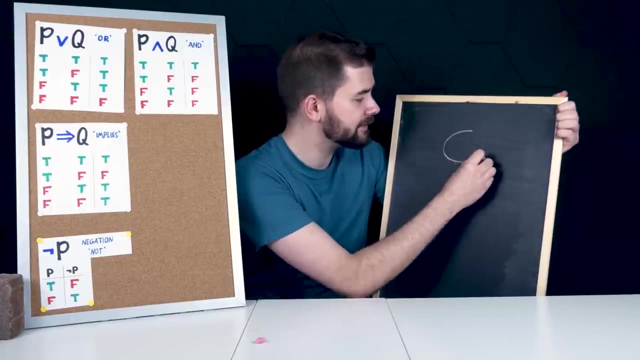 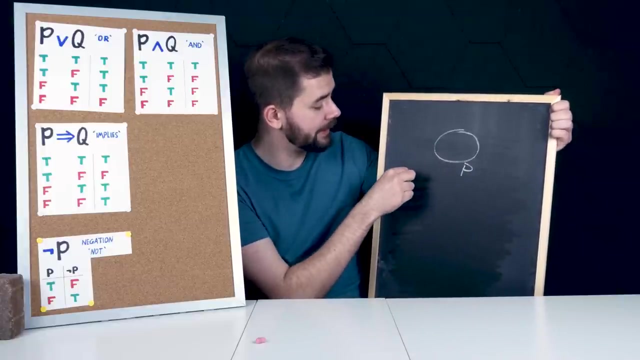 all possible situations. So everything that could possibly happen or ever happen, or will happen or has happened is represented by some position on this board. It'll make sense in a minute, trust me. So this board represents all situations And inside this blob is the situations in which P is true. So if this is a situation, right here. 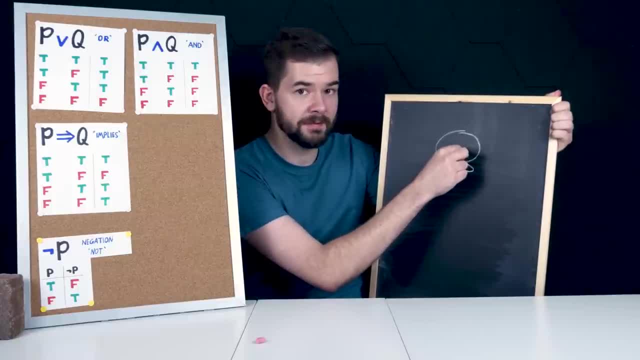 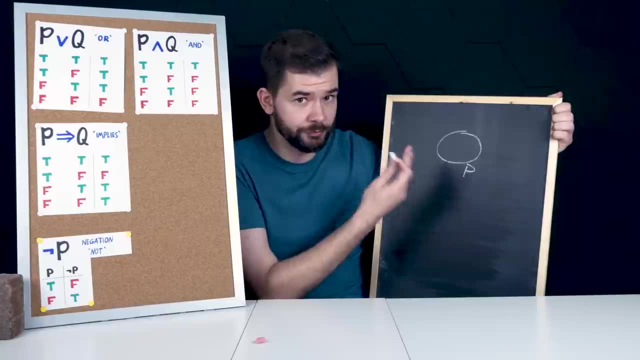 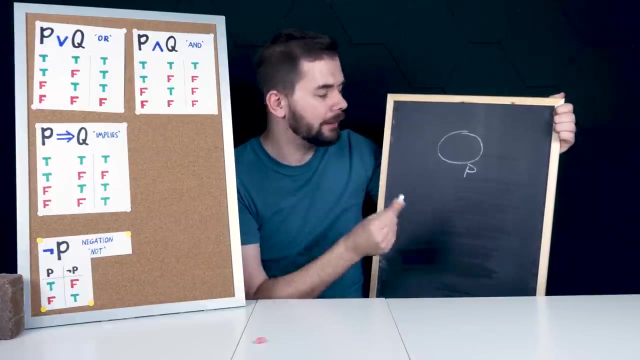 P is false. If this is a situation inside this P space, then P is true. Now let's think about what it looks like if P implies Q. So whenever P is true, Q is automatically true. How are we going to draw the blob representing Q? Well, if you think about it, the only way 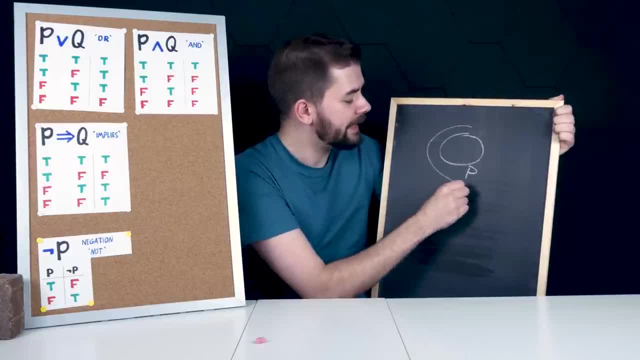 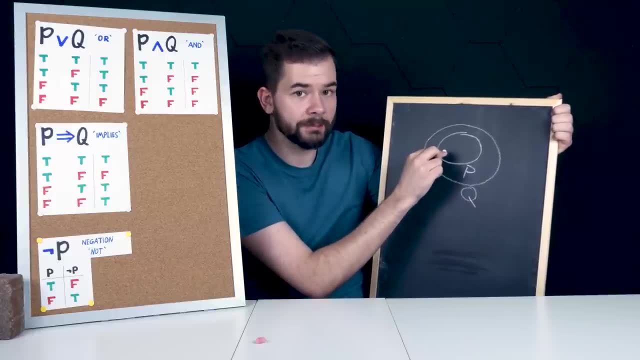 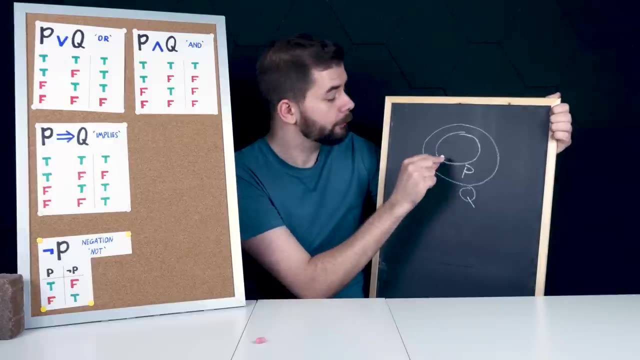 to do? it is to draw a blob where P is nested inside Q. That way, whenever P is true, Q is automatically true. So whenever we're inside the P space, we're automatically inside the Q space. And now look, if P is true, we're inside the P space. 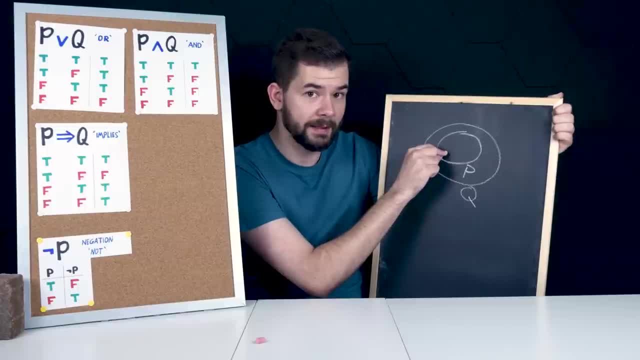 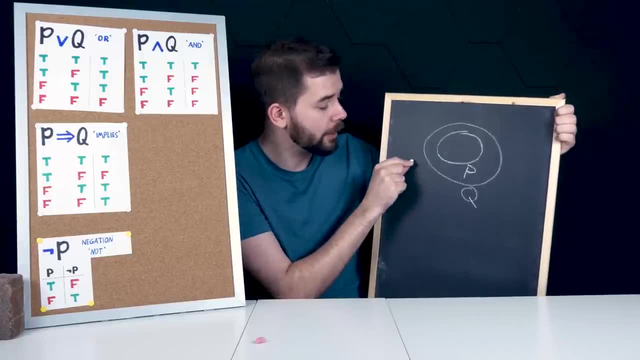 Q is automatically true because we're automatically inside the Q space, But if P is false, then we don't know anything about whether Q is true. If we're outside the P space, we could be inside the Q space or outside the Q space. 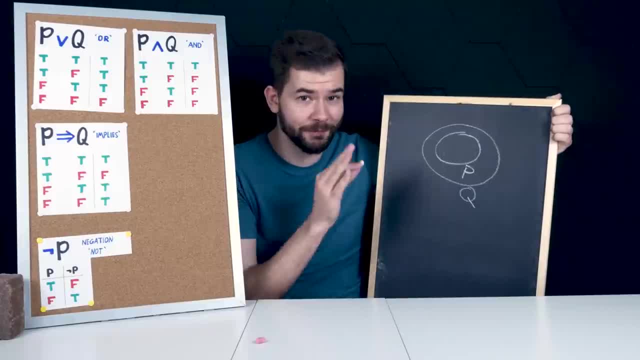 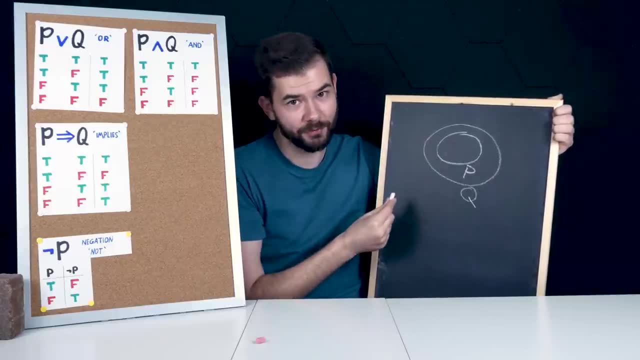 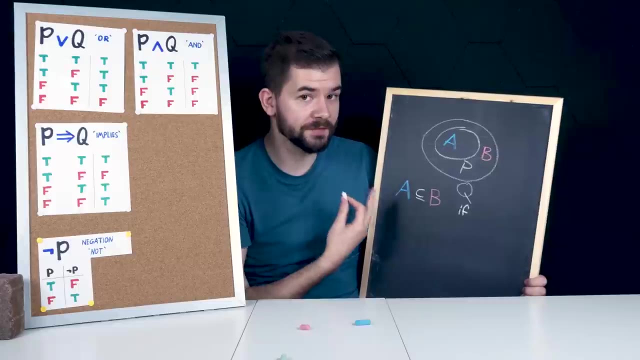 Both situations are perfectly valid. The only situation which is impossible is if P is true yet Q is false, ie we're inside the P space yet outside the Q space. This visual representation is beneficial as well because we also use an implication to describe when one set is a subset of the other. 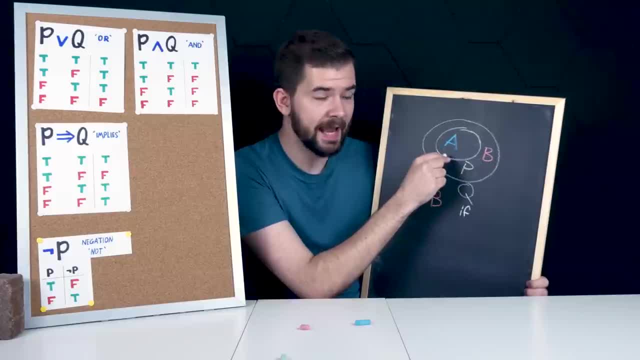 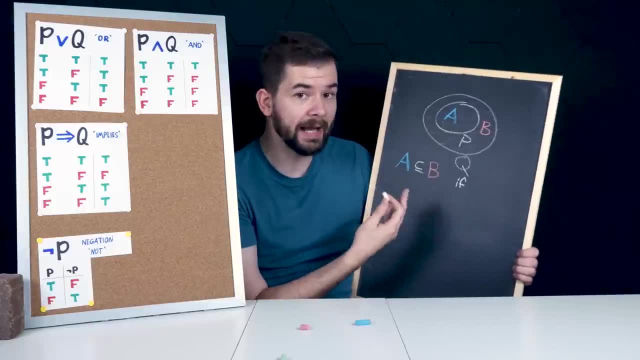 So now let's say that this small circle is the set A and it's contained within the set B. Logically we say A is a subset of B or A is contained in B. If X is in A, implies X is in B. 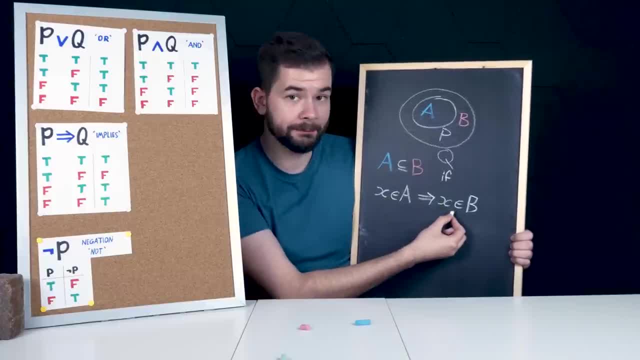 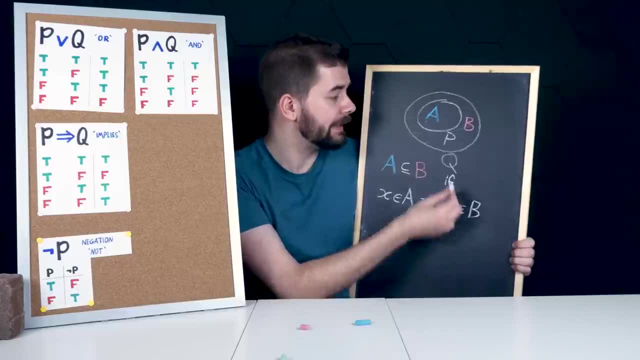 If X is an element of A, it should automatically be an element of B. But if X is not a member of A, we don't really care about whether it's in B. It could be one of the ones that's inside B, or it could be the one of the ones that's outside B. 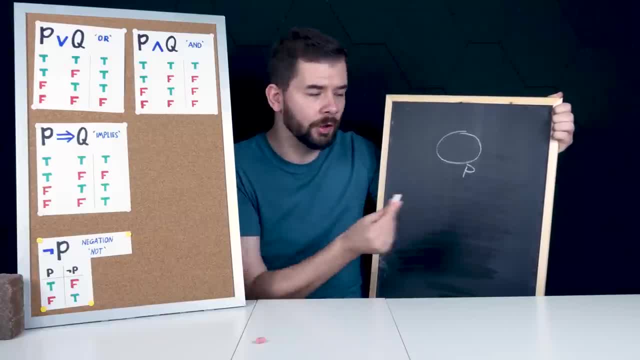 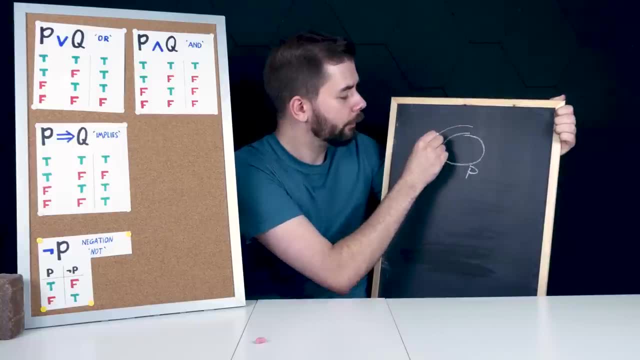 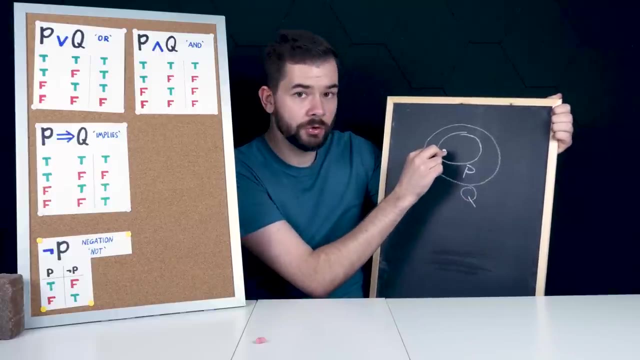 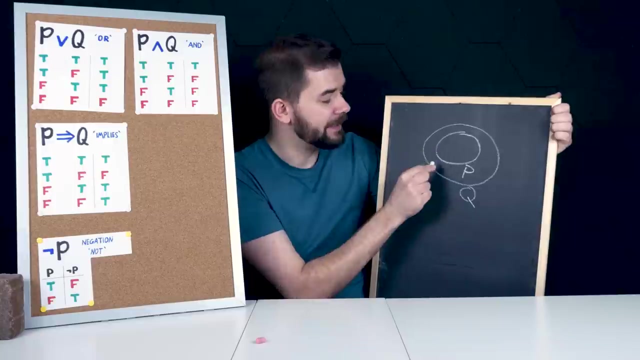 q is automatically true. how are we going to draw the blob representing q? well, if you think about it, the only really way to do it is to draw a blob where p is nested inside q. that way, whenever p is true, q is automatically true. so whenever inside the p space, we're automatically inside the q space. and now look if p is true. 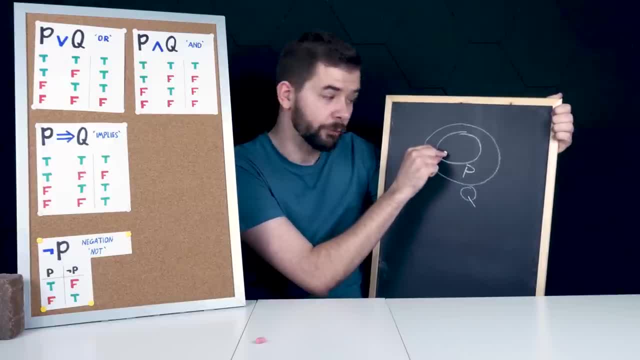 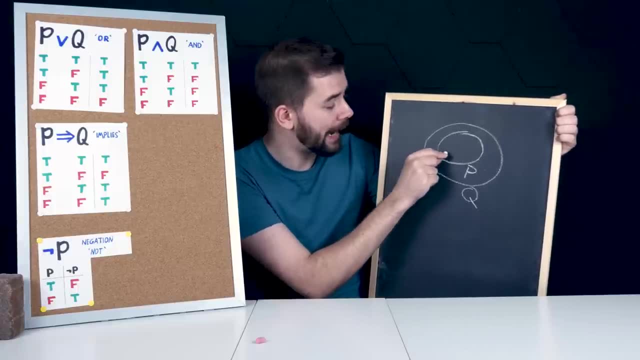 we're inside the p space, q is automatically true because we're automatically inside the q space. but if p is false, then we don't know anything about whether q is true. if we're outside the kenya'tor, the p space, we could be inside the q space or outside the q space. Both situations are perfectly. 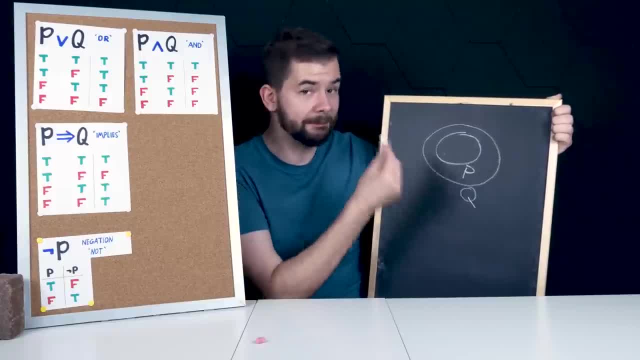 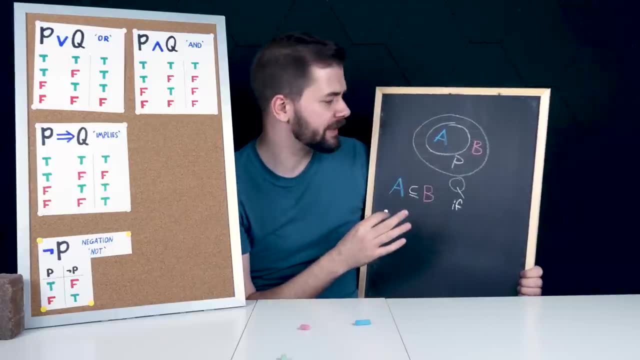 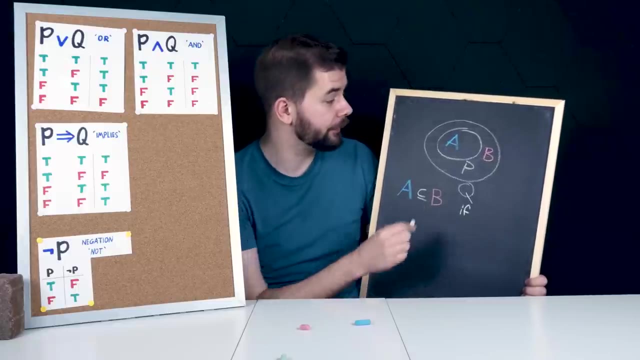 valid. The only situation which is impossible is if p is true yet q is false, ie we're inside the p space yet outside the q space. This visual representation is beneficial as well because we also use an implication to describe when one set is a subset of the other. So now let's say: 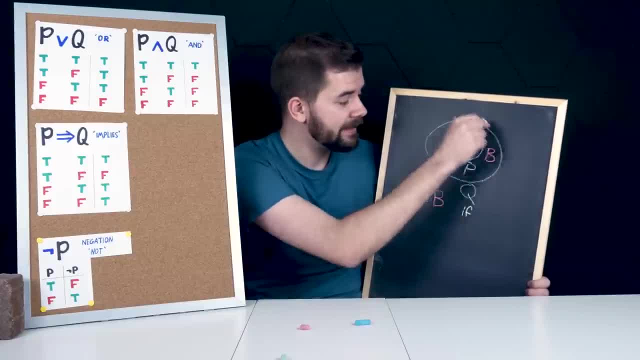 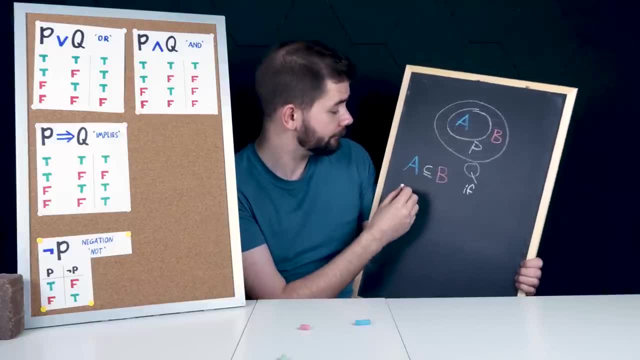 that this small circle is the set a and it's contained within the set b. Logically we say: a is a subset of b or a is contained in b. If x is in a, implies x is in b. If x is an element of a. 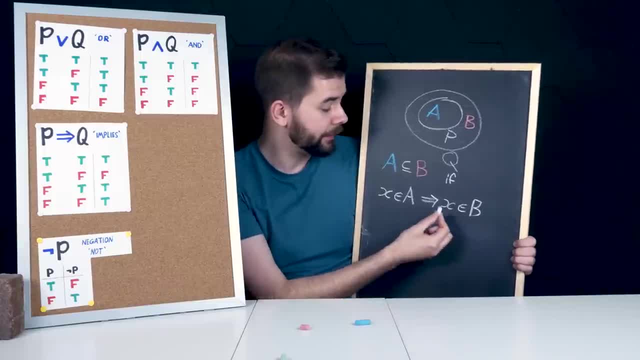 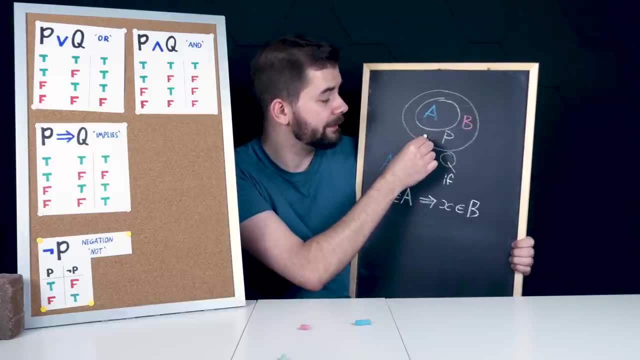 it should automatically be an element of b. But if x is not a member of a, we don't really care about whether it's in b. It could be one of the ones that's inside b, or it could be the one of the ones that's outside b. We don't really care. 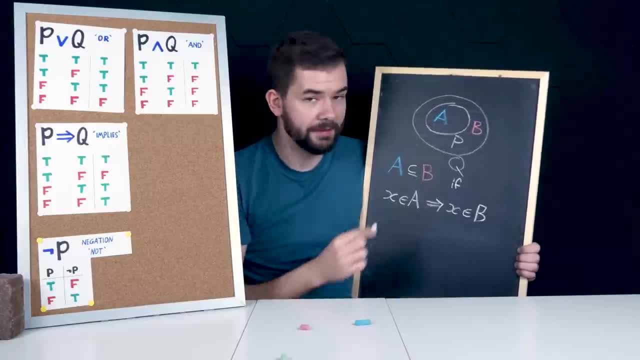 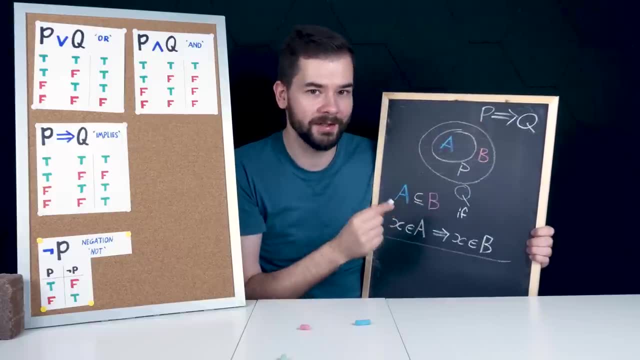 we only care that one set is nested inside the other when thinking about subsets. It's worth noting here that most often in mathematics we're dealing with situations in which we know the first statement is true. So when we're writing a proof, for example, 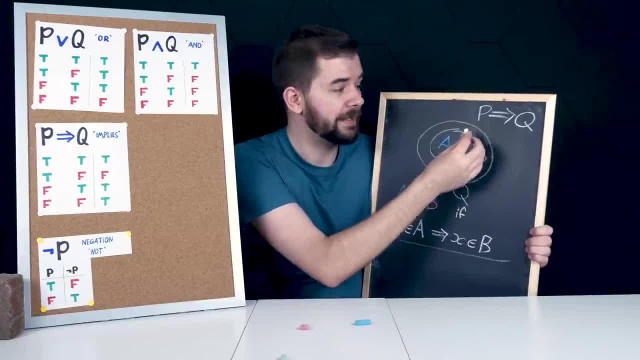 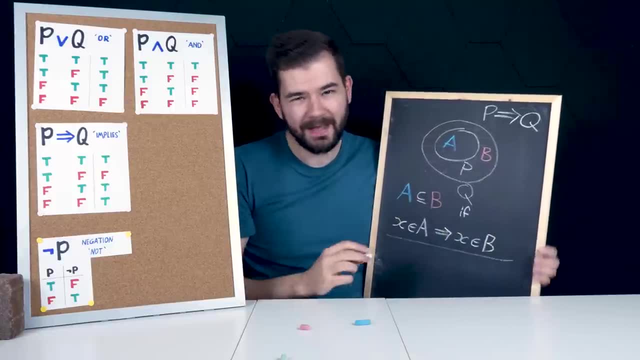 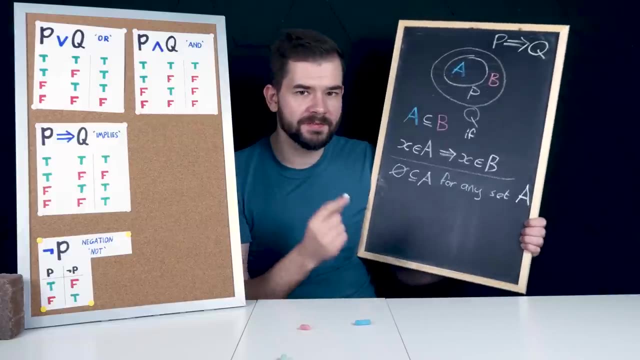 we often either know p is true or we assume p to be true and we string together some implications so we conclude that the consequences are also true. But that's not always the case. Let me show you a classic example in which we know that the first statement is false. So this is in proving. 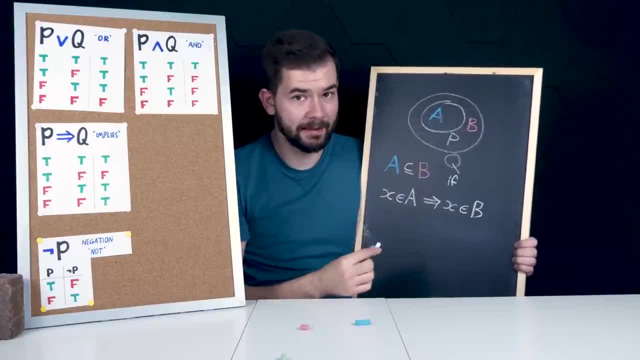 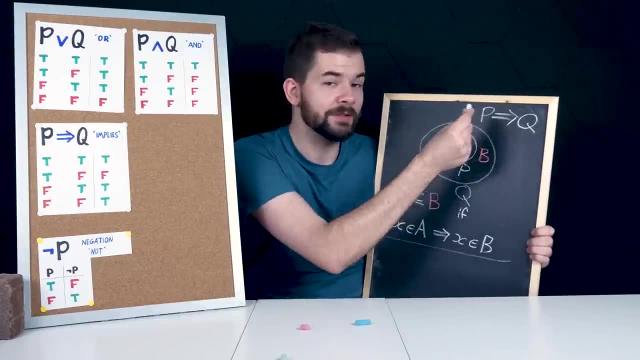 We don't really care. We only care that one set is nested inside the other when thinking about subsets. It's worth noting here that most often in mathematics we're dealing with situations in which we know the first statement is true. So when we're writing a proof, for example, 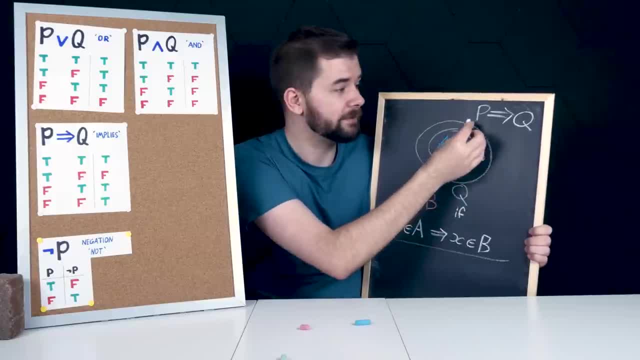 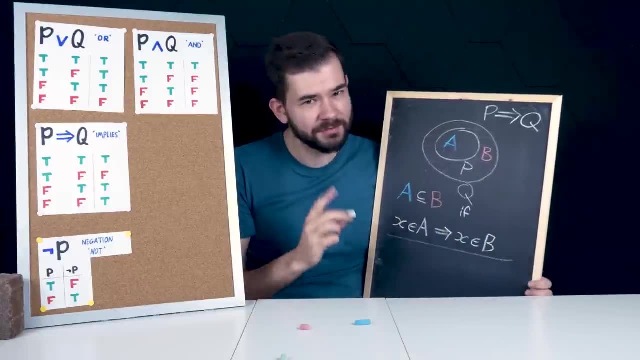 we often either know P is true or we assume P to be true and we string together some implications so we conclude that the consequences are also true. But that's not always the case. Let me show you a classic example in which we know that the first statement is false. 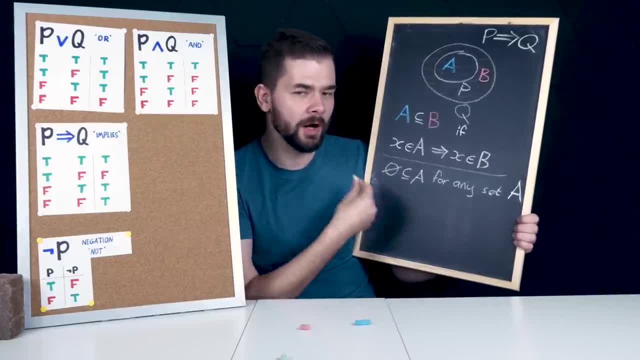 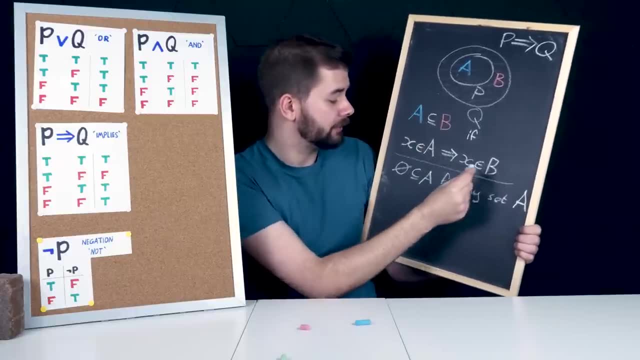 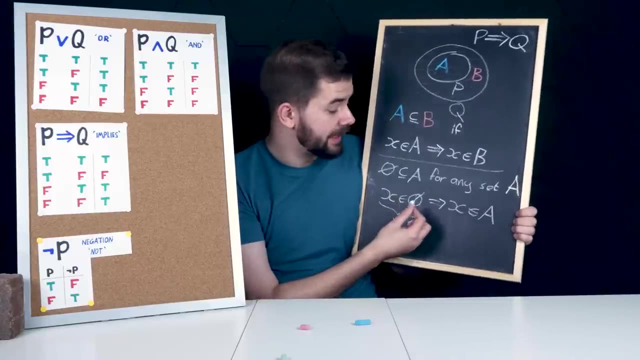 So this is in proving that the empty set is a subset of any set A, And this works because A is a subset of B, if this implication holds. So let's just rewrite this implication but with these terms involved instead. So X is in the empty set implies X is in A. 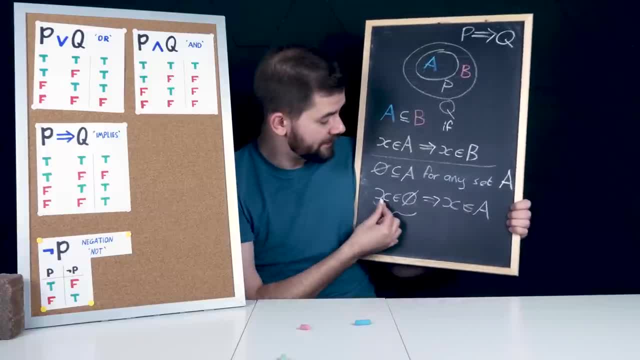 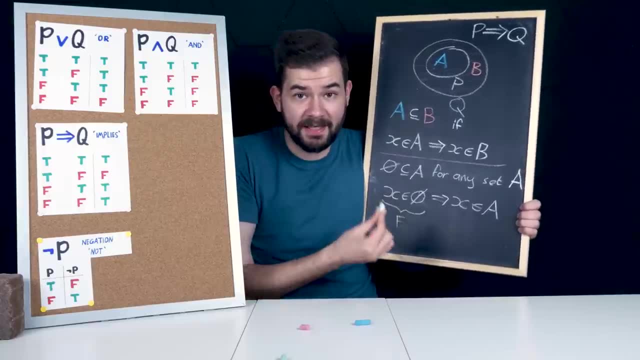 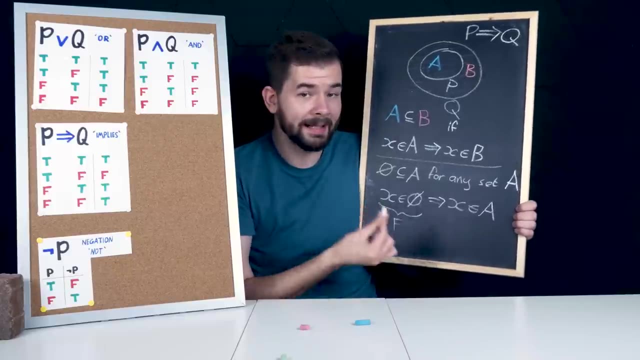 But this implication is always true, because this first statement is always false because X is in the empty set is always false, as the empty set is defined as the set that contains no elements. Since this is always false, this implication is always true. So, by definition, 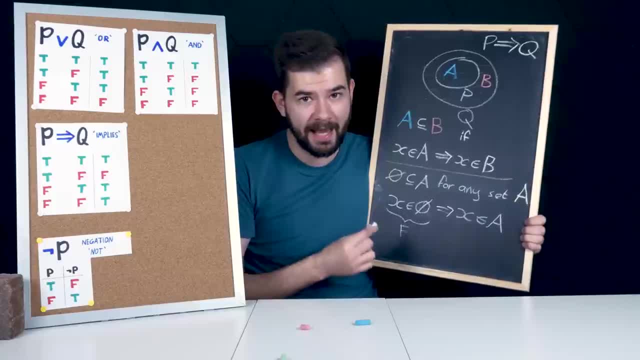 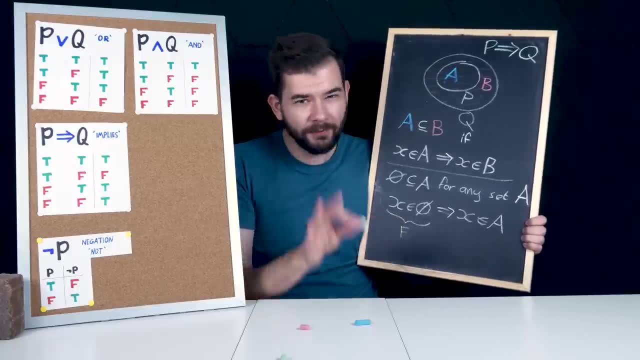 the empty set is always a subset of any given set. A. This kind of implication is known as a vacuous implication, where the first statement is always false. Not often encountered in mathematics, but sometimes. But something magic happens when we're in the situation. 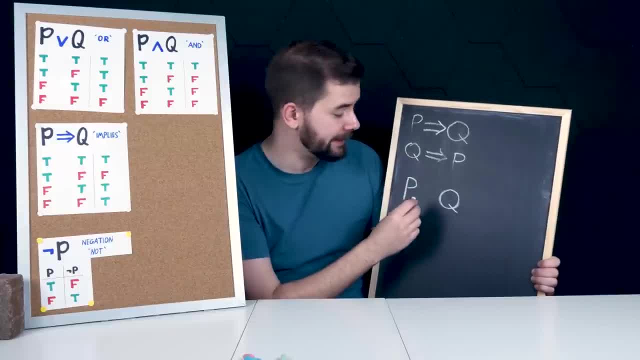 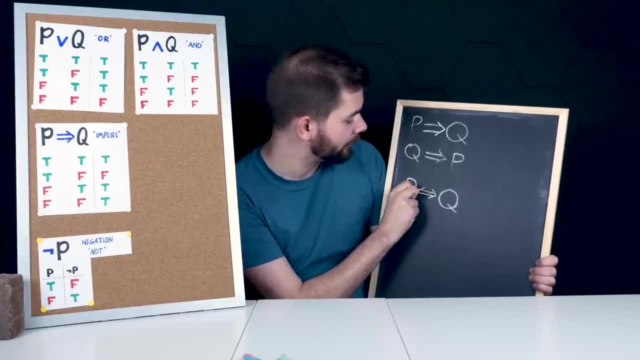 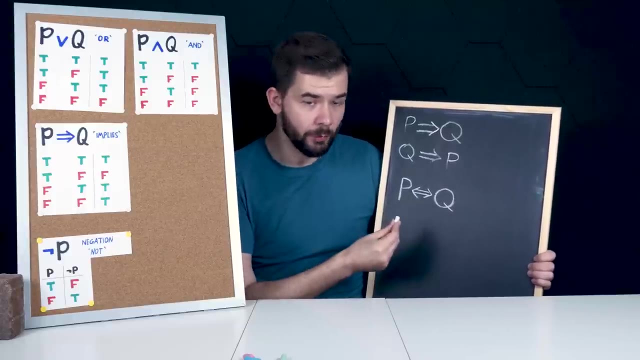 that P implies Q and Q implies P. We often nest these situations together with a special symbol like this: This a double arrow, And we read this: P if, and only if, Q. This is true whenever both of these are true or whenever both are false. 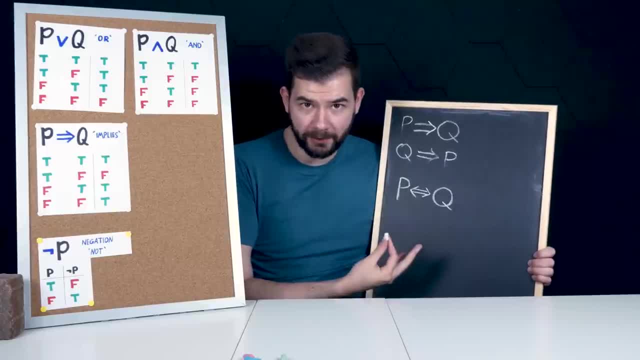 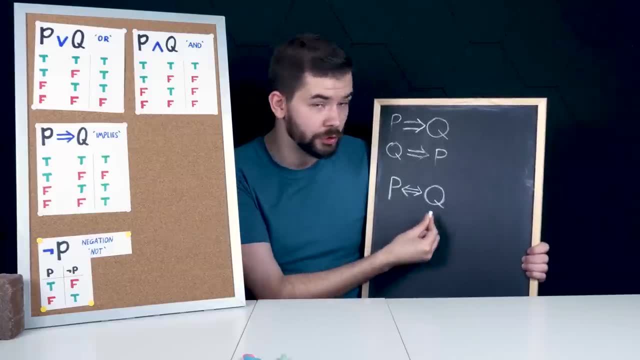 We say that P and Q are logically equivalent because the exact circumstances under which P is true are identical to the circumstances under which Q is true. They're effectively both saying the same thing. Let's look at some examples. So an early mathematical example: 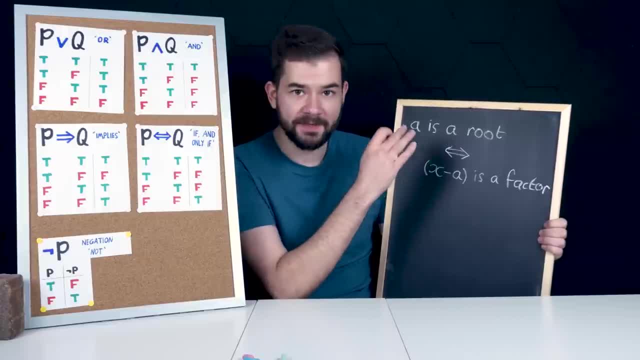 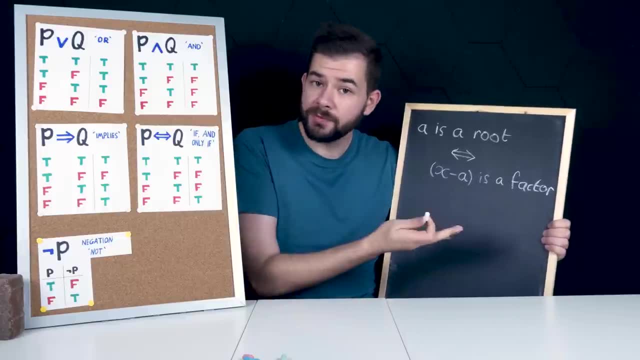 you might come across is the factor theorem. If A is a root of a polynomial, F of X, then X minus A is a factor of that polynomial. To have a root and to have a linear factor are one and the same. If you have a root A. 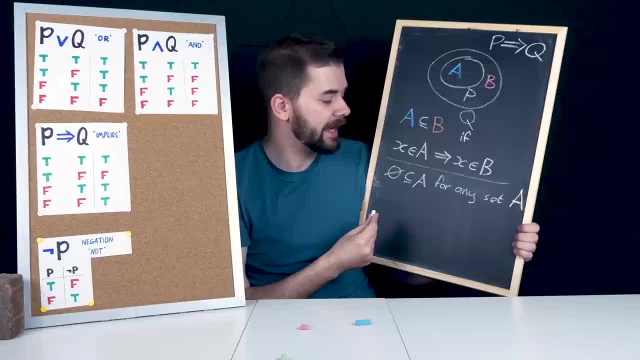 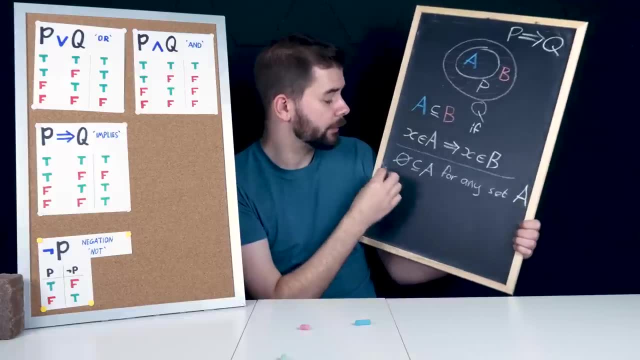 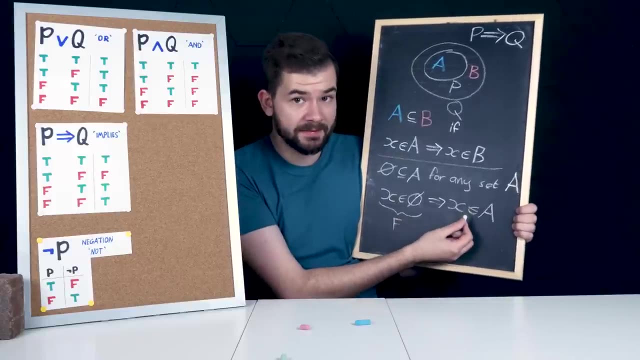 that the empty set is a subset of any set, a, and this works because a is a subset of b, if this implication holds. So let's just rewrite this implication, but with these terms involved instead. So x is in the empty set implies x is in a, but this implication is always true because this: 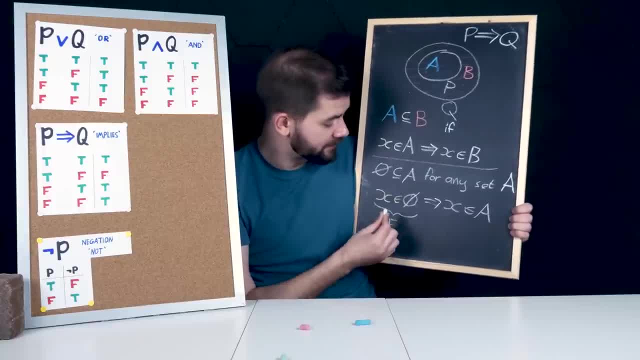 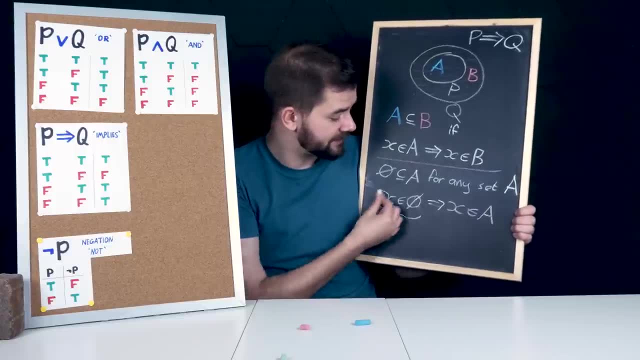 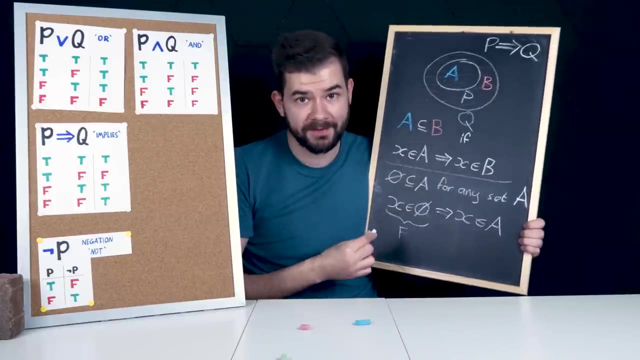 first statement is always true. So this first statement is always false because x is in the empty set is always false as the empty set is defined as the set that contains no elements. Since this is always false, this implication is always true. So, by definition, the empty set is always a subset of any given set, a. 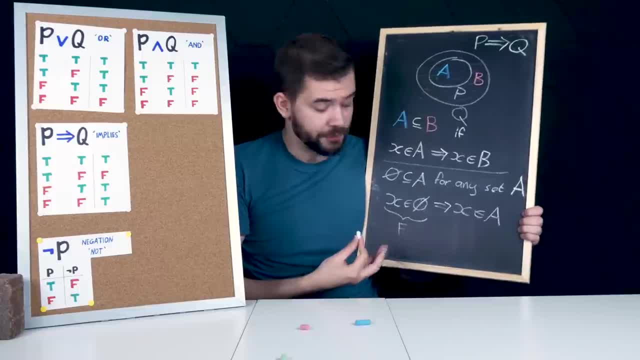 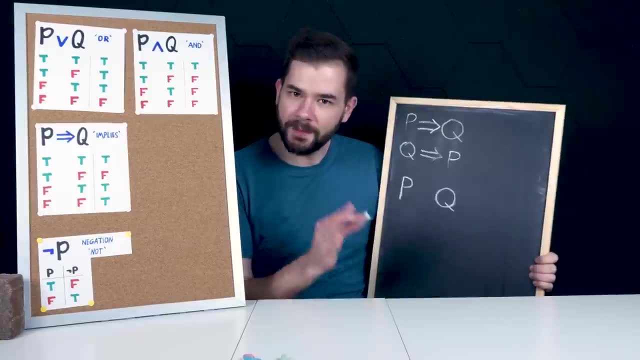 This kind of implication is known as a vacuous implication, where the first statement is always false. Not often encountered in mathematics, but sometimes. But something magic happens when we're in the situation that p is false. So the first statement is always false. So this implication is: 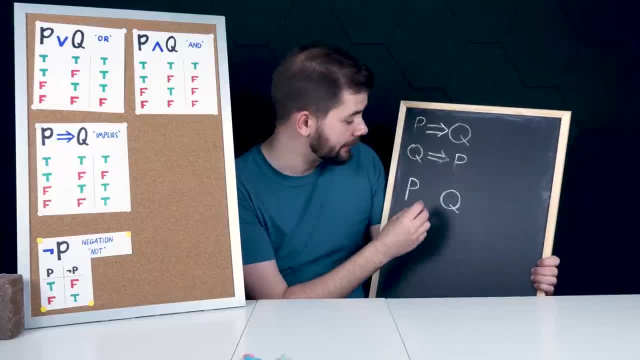 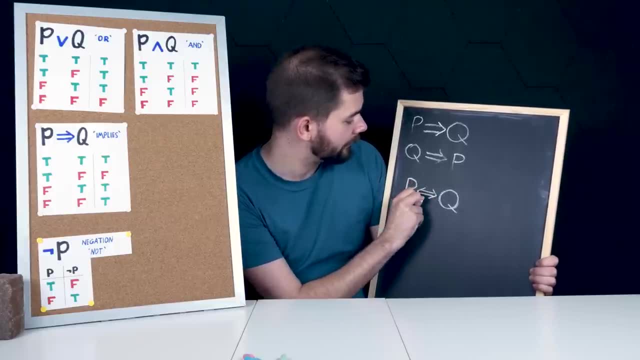 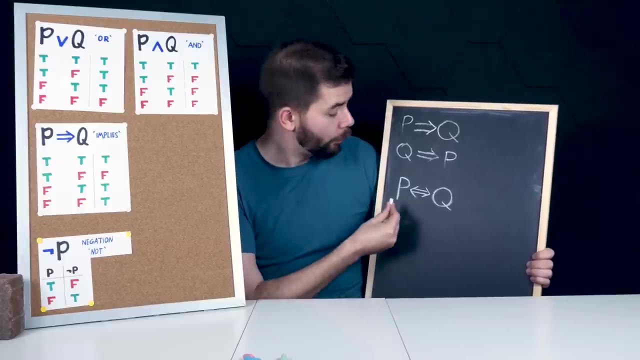 always true. So we say that p implies q and q implies p. We often nest these situations together with a special symbol like this, a double arrow, And we read this: p if, and only if, q. This is true. whenever both of these are true, or whenever both are false, We say that p and q are. 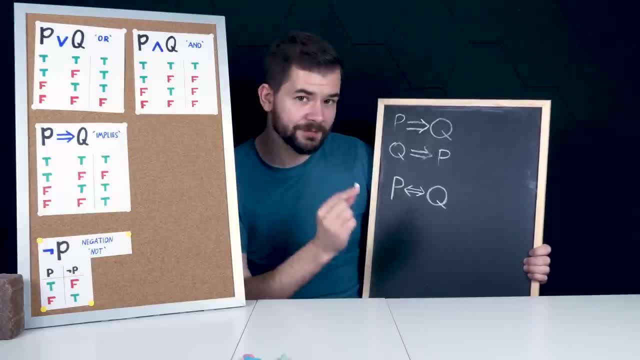 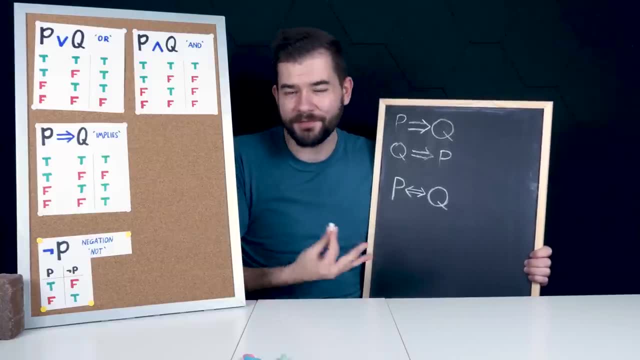 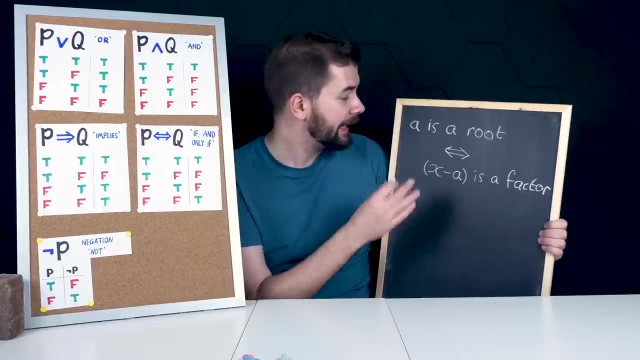 logically equivalent, because the exact circumstances under which p is true are identical to the circumstances under which q is true. They're effectively both saying the same thing. Let's look at some examples. So an early mathematical example you might come across is the factor theorem. If a is a root of a polynomial f of x, then x minus a is a factor of that. 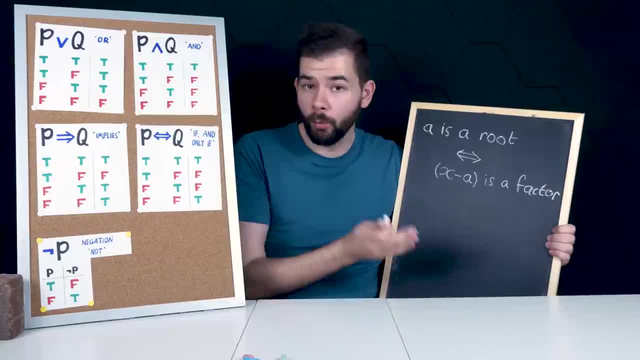 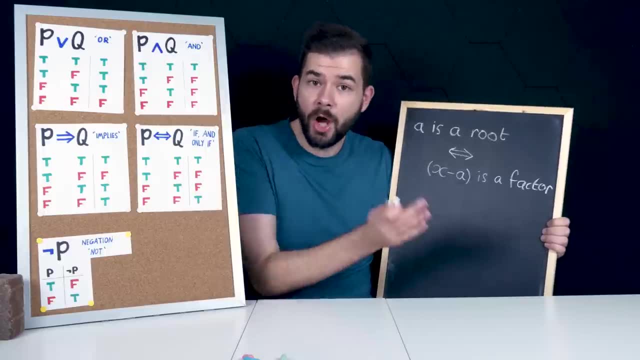 polynomial. To have a root and to have a linear factor are one and the same. If you have a root- a- then you know x minus a is a factor. And if you have a factor- x minus a- then you know that a is a. 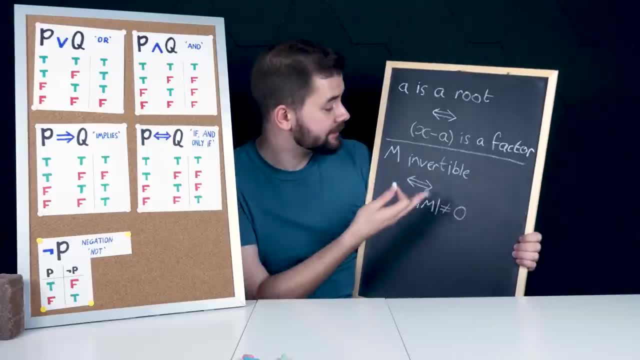 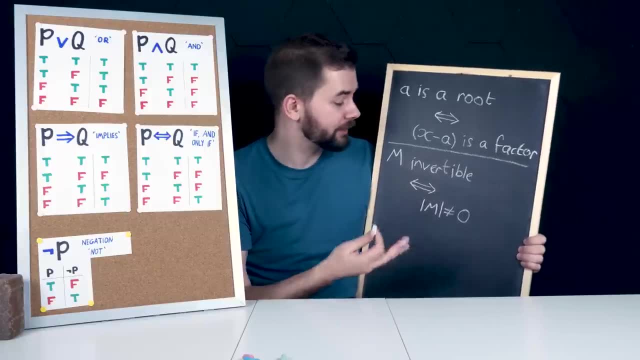 root. Another one you'll come across early in undergraduate study- is that if m is a matrix, m is invertible if, and only if, the determinant of m is not zero. So they mean the same thing: If m is invertible, it will have non-zero determinant, and if it has non-zero determinant, 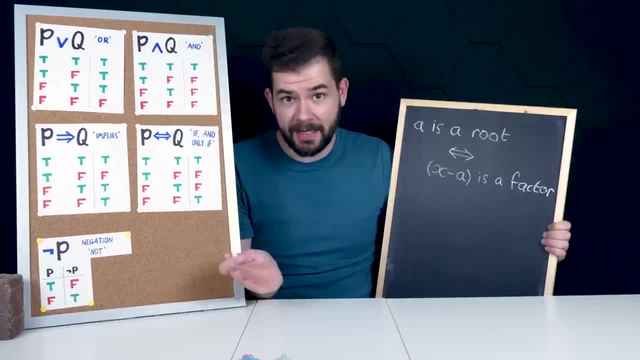 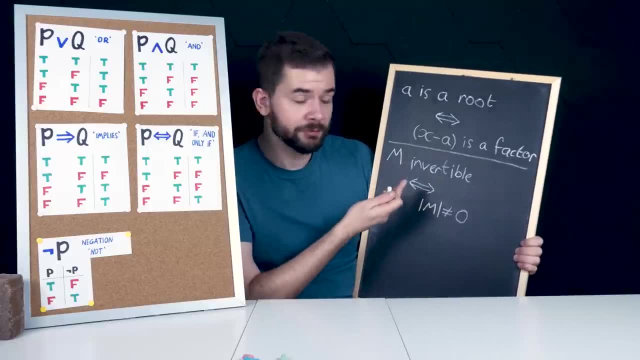 then you know X minus A is a factor. And if you have a factor X minus A, then you know that A is a root. Another one you'll come across early in undergraduate study is that if M is a matrix, M is invertible if, and only if, the determinant of M 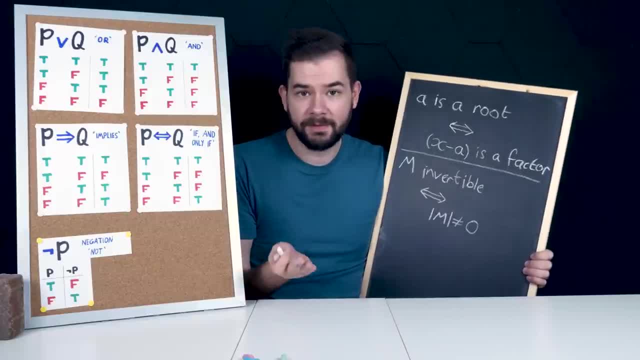 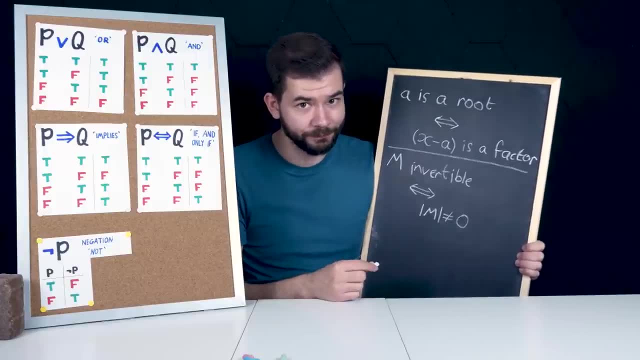 is not X zero. So they mean the same thing: If M is invertible, it will have nonzero determinant, and if it has nonzero determinant, it will be invertible. And finally, another kind of less well-known one is: we all learn at school that if 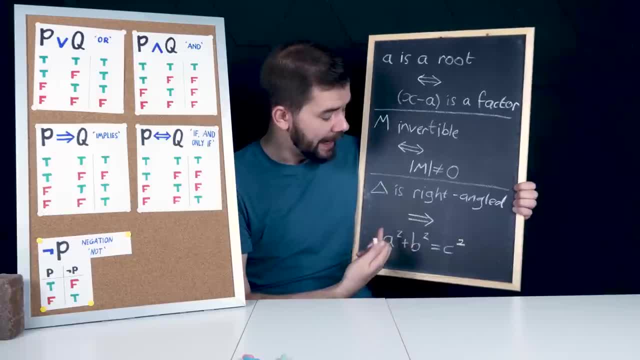 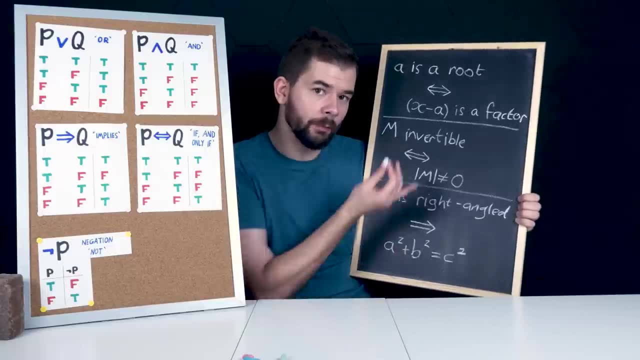 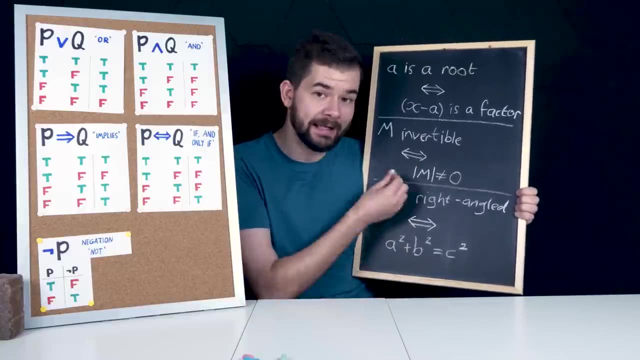 the triangle is right angled, then a squared plus b squared equals c squared will hold true where c is the length of the hypotenuse. But actually the other way around works as well. If you happen to have a triangle in which a squared plus b squared equals c squared, then it must be a right angled triangle. Now a. 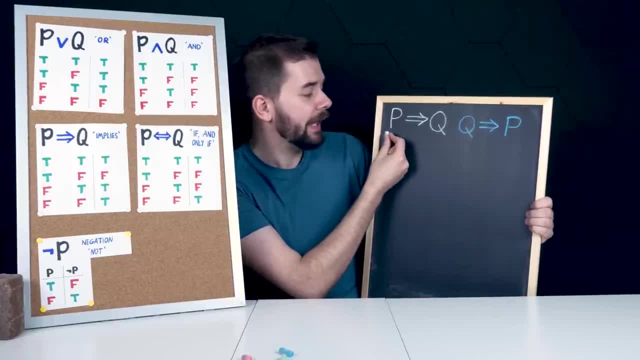 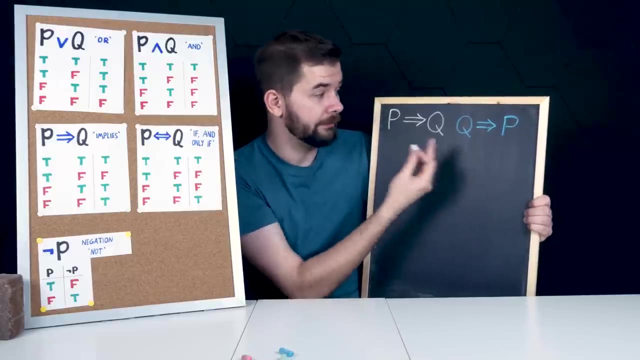 common error that students make is that if an implication holds in one direction, then the implication holds in the other direction. But this isn't true. The statement P implies Q, and this statement here, which has nothing to do with what shoes it's wearing, but it's called the converse of the original statement, are 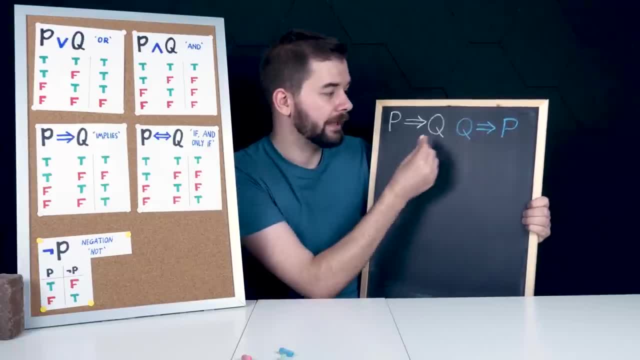 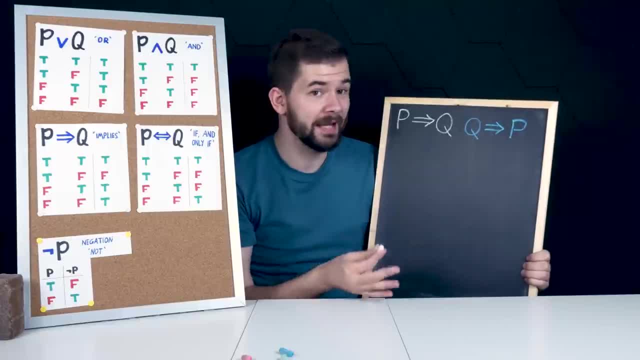 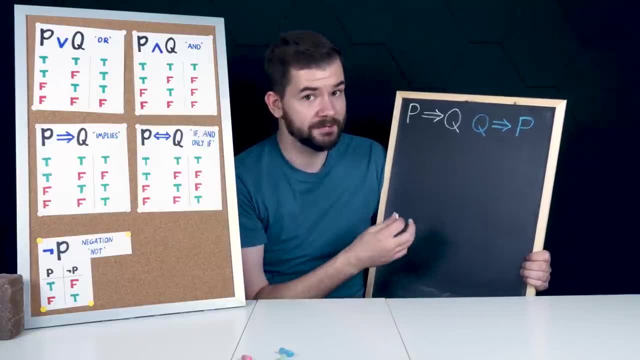 Pythagorean theorem, but it's not always the case. In fact, I would say most of the time it isn't the case. Let's make some basic mathematical statements and see why this. most of the time that this breaks down. We had this example earlier. X is a. 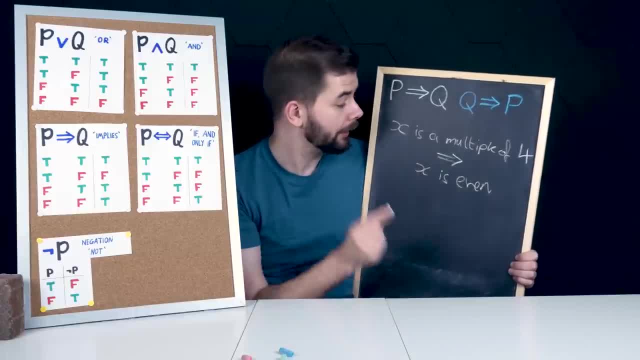 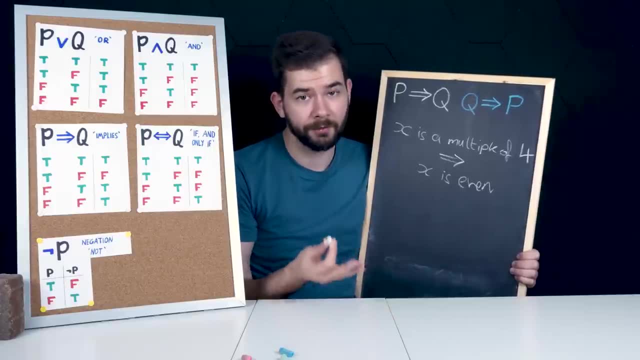 multiple of 4 implies X is even True, But X is even does not imply that X is a multiple of 4, because it could be an even non-multiple of 4, like 6 or something like that. Let's look at another one. 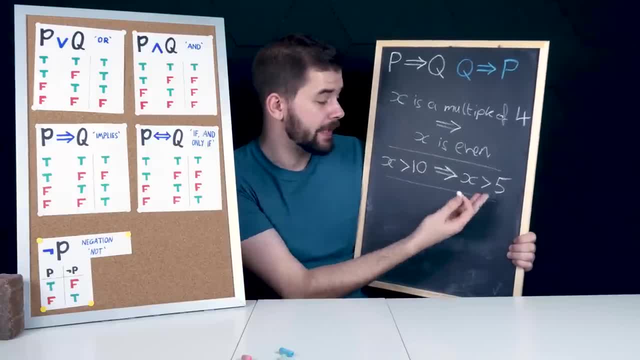 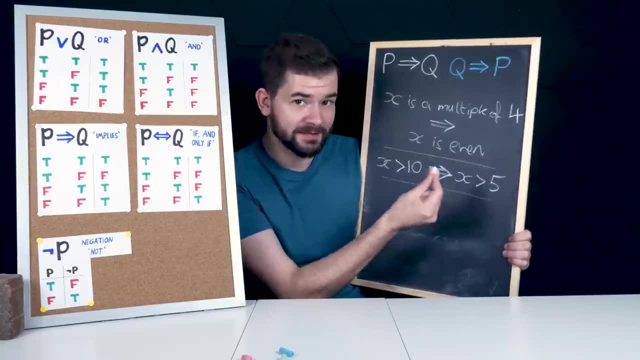 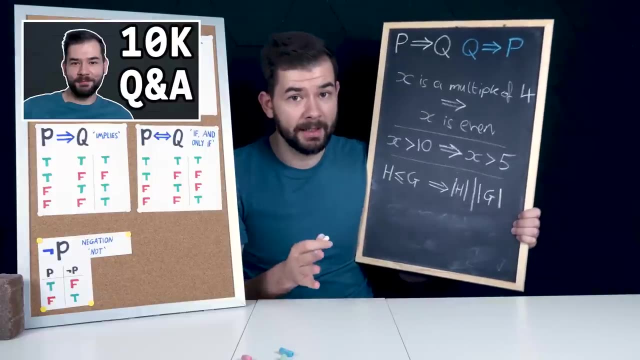 Perhaps an even more basic example: X is greater than 10 does imply that X must be greater than 5.. However, the other direction definitely doesn't hold. X is greater than 5 does not necessarily mean that X is greater than 10, because X could be a number like 6 or 7 or tau. In my 10k Q&A video, I was 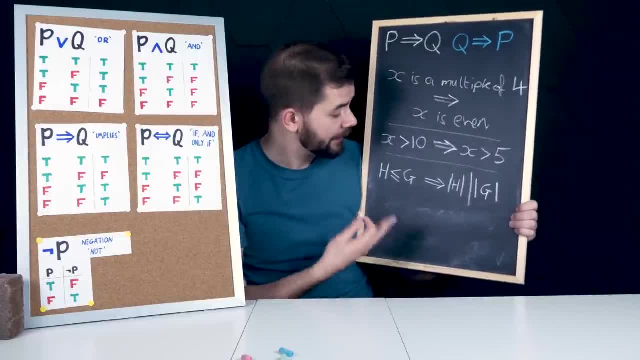 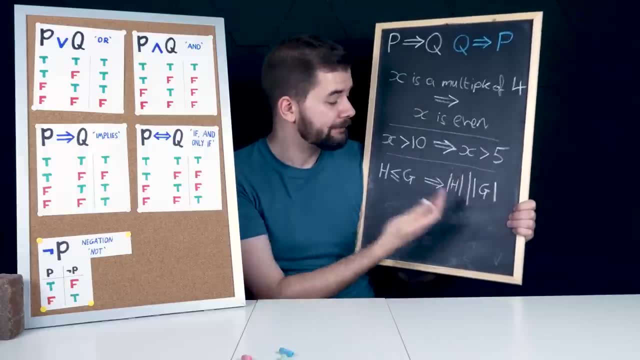 discussing one of my favorite theorems, Lagrange's theorem for groups. This says that if H is a subgroup of G, then the order of H divides the order of G, But not the other way around. If I have a subset H of G, where the 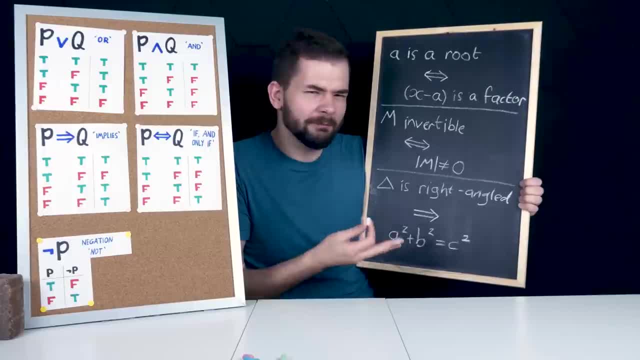 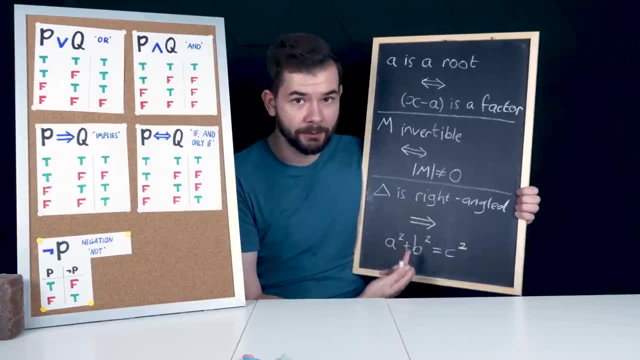 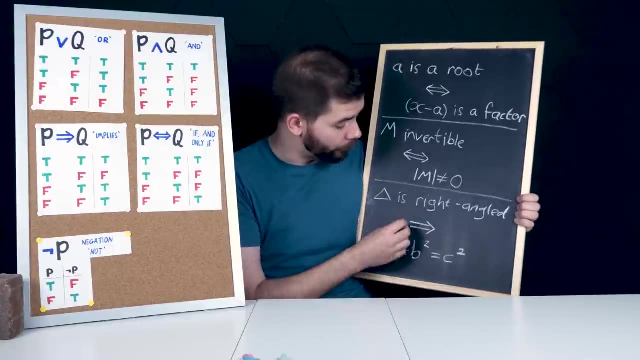 it will be invertible. And finally, another kind of less well-known one is: we all learn at school that if the triangle is right-angled, then a squared plus b squared equals c squared. will hold true where c is the length of the hypotenuse. But actually the other way around works as well. 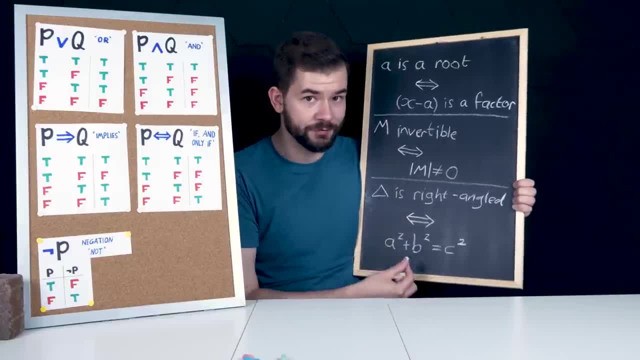 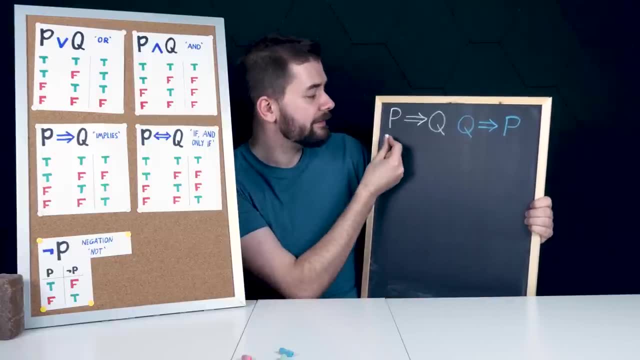 If you happen to have a triangle in which a squared plus b squared equals c squared, then it must be a right-angled triangle. Now, common error that students make is that if an implication holds in one direction, then the implication holds in the other direction. But 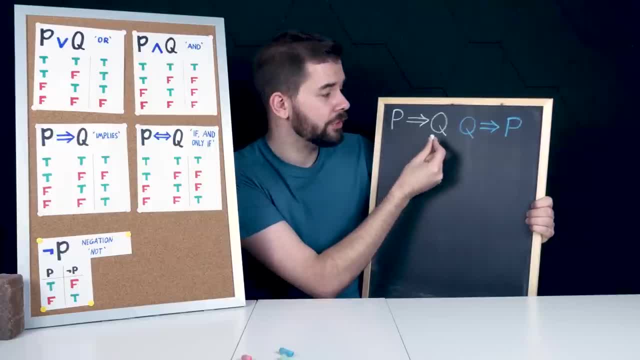 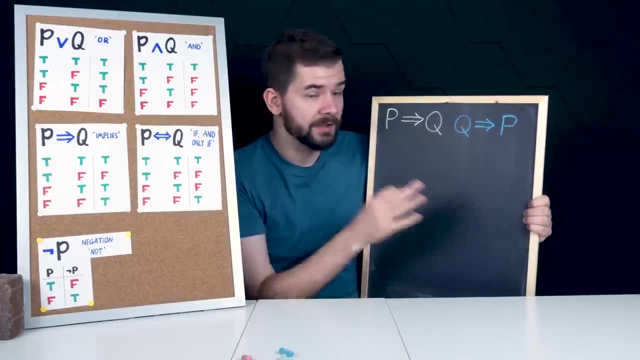 this isn't true. The statement p implies q, and this statement here, which has nothing to do with what shoes it's wearing, but it's called the column, is the inverse of the original statement. They are two different things. Now we've seen some. 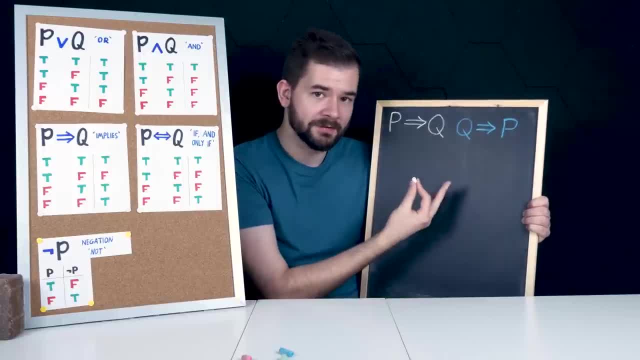 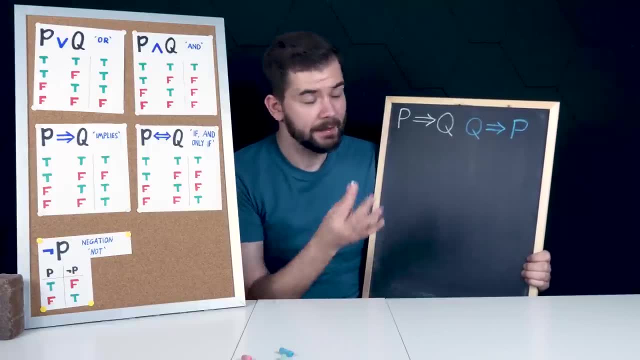 examples of the implication working in both directions, like in the factor theorem or like in the pythagorean theorem. but it's not always the case. In fact I would say most of the time it isn't the case. Let's make some basic mathematical statements and see why this. 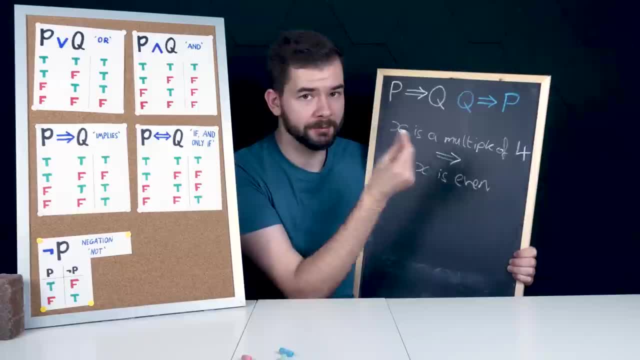 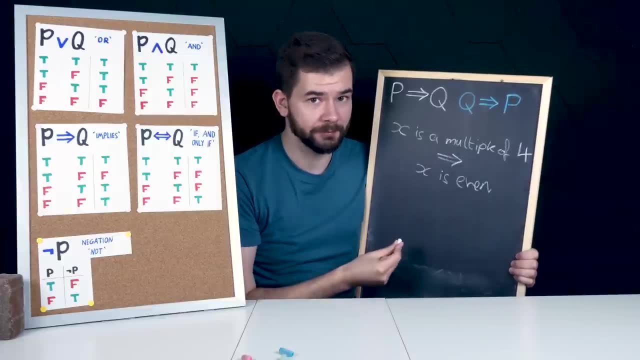 most of the time that this breaks down. We had this example earlier: X is a multiple of four implies x is even True. But x is even does not imply that x is a multiple of four, Because it could be an even non-multiple of four, like six or something like that. 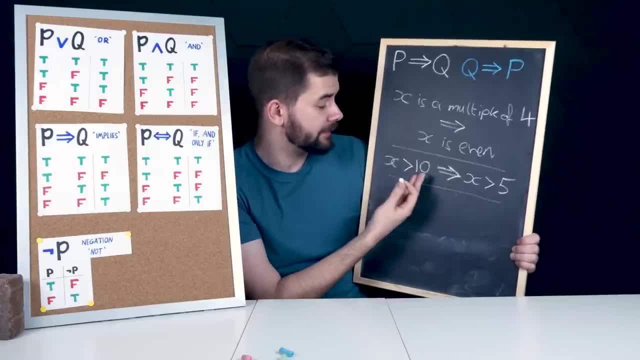 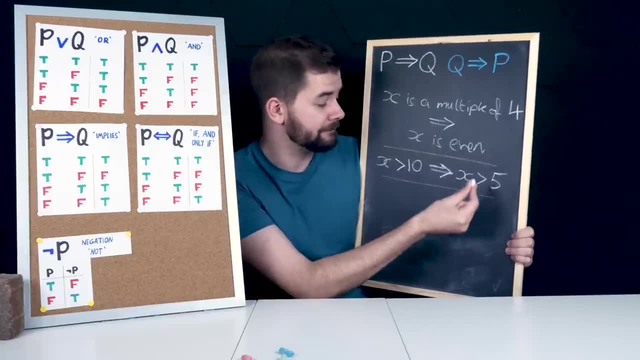 Let's look at another one, Perhaps an even more basic example. X is greater than ten does imply that x must be greater than five. However, the other direction definitely doesn't hold. X is greater than five does not necessarily mean that x is greater than ten, because x could. 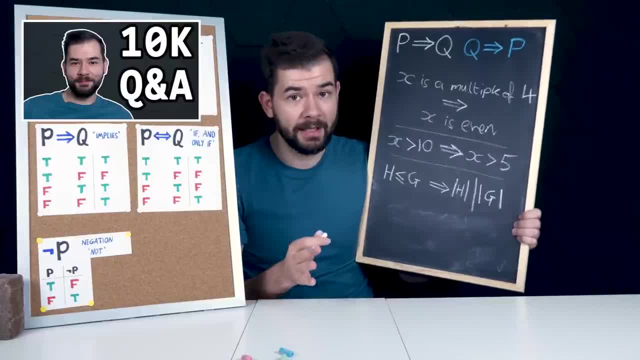 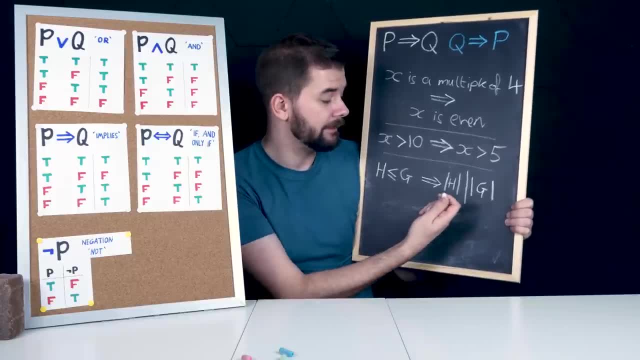 be a number like six or seven or tau. In my 10k Q&A video I was discussing one of my favorite theorems, Lagrange's theorem for groups. This says that if h is a subgroup of g, the order of h divides the order of g, But not the other way around. If I have a subset h of g. 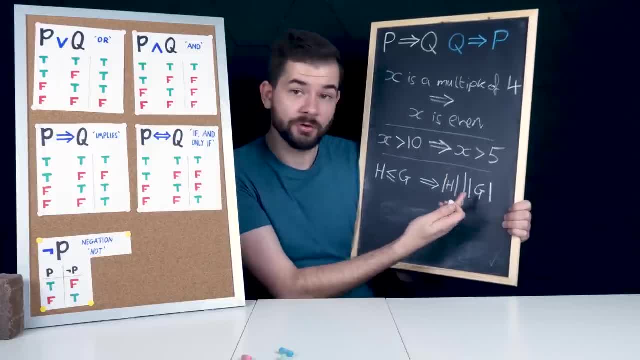 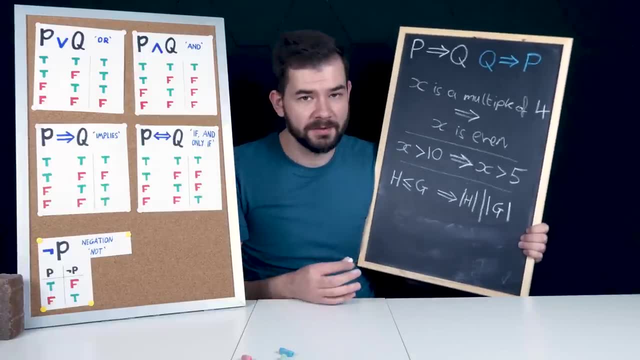 where the cardinality of h happens to divide the cardinality of g, that does not necessarily mean that h is a subset of g, And you find these sort of things all over the place. I don't know. in real analysis, every a function is differentiable implies that it's continuous. 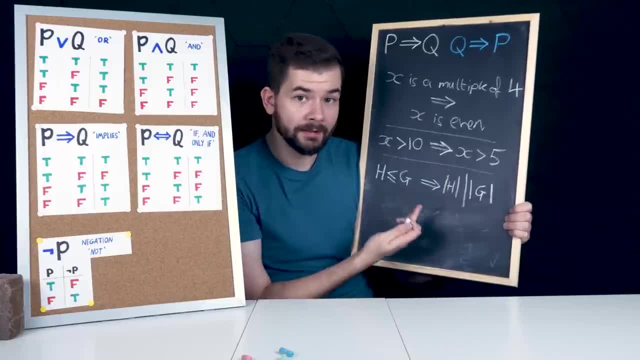 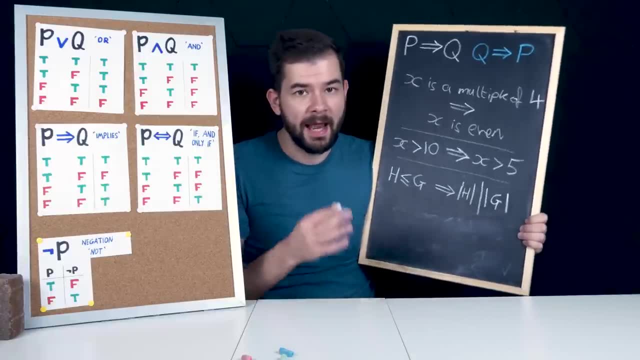 cardinality of H happens to divide the cardinality of G, that does not necessarily mean that H is a subset of G, And you find these sort of things all over the place, I don't know. in in real analysis, every a function is differentiable implies that it's continuous, but not every continuous. 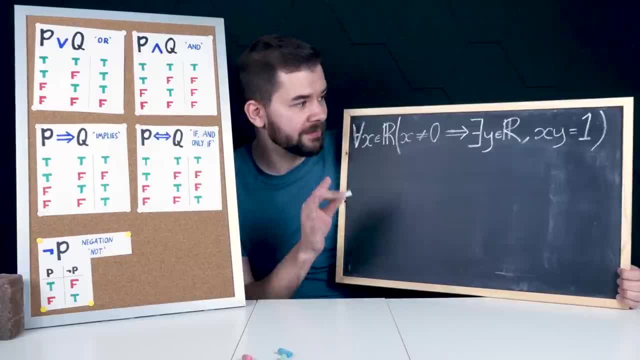 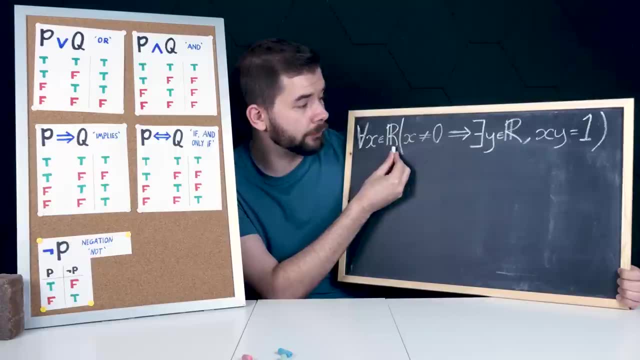 function is differentiable, and so on. All of this is coming together for statements, like we had at the start of the video. Here we're also using this blackboard bold R to represent the set of real numbers and this e-shaped symbol for membership. So this means. 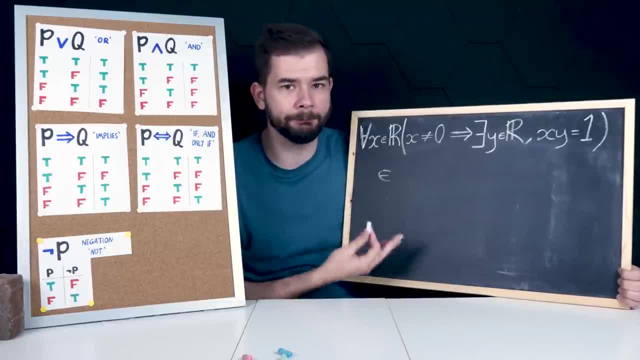 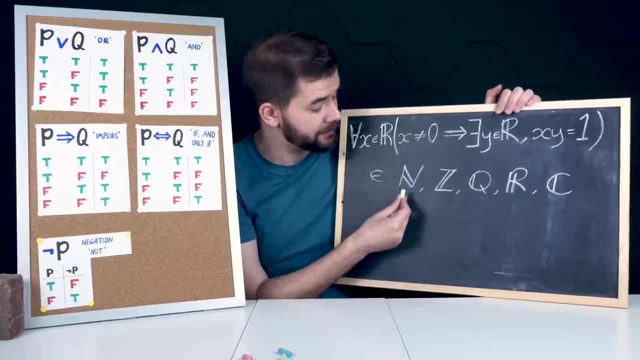 is an element of, and we have a bunch of blackboard bold notations that we use to represent different sets of numbers. The common ones are: N for the natural numbers, that's, positive integers, sometimes including zeros, sometimes not. there's really no consensus. Z for the integers, the whole numbers. Q for the. 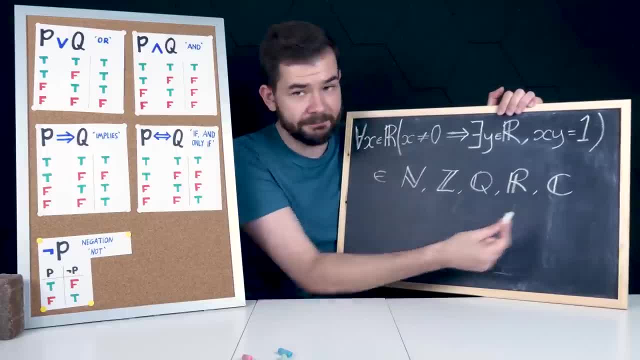 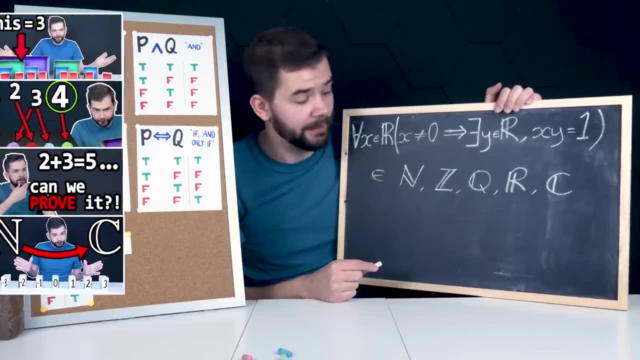 rational numbers, the fractions. R for all the real numbers, C for the complex numbers. How are these sets actually defined? I have a short series of videos about that. you should check it out. By short, I mean there's four videos in the series. It is three and a half hours long, but you know There are other ones as 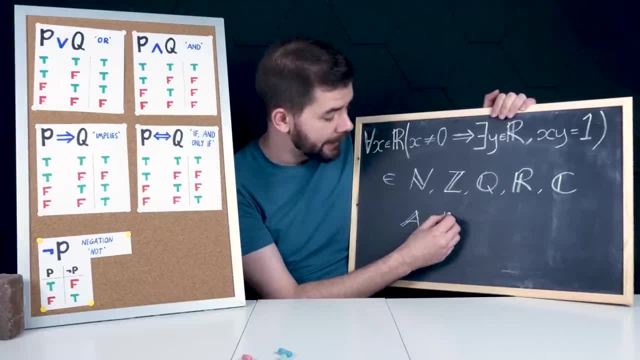 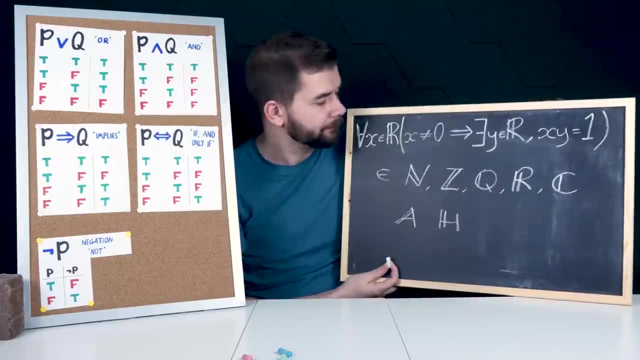 well, but less common. you'll see A maybe for the algebraic numbers and black board bold H for the set of quaternions. But let's not worry about that now, let's just focus on this statement up here. So we have something about a real number X. 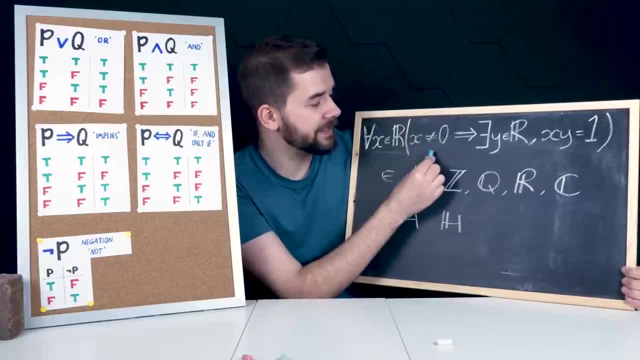 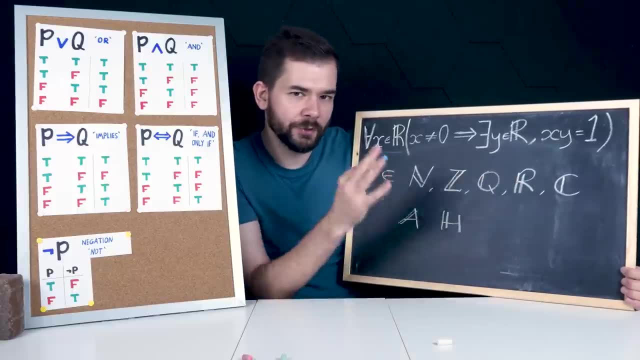 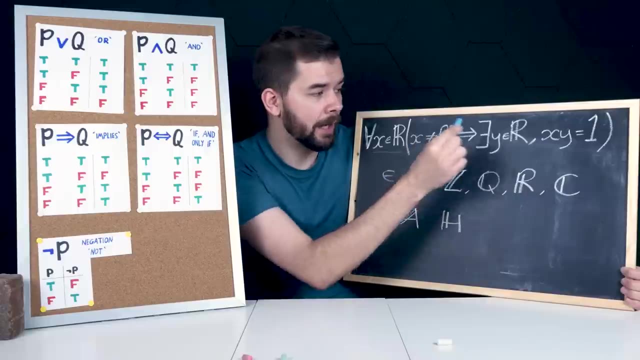 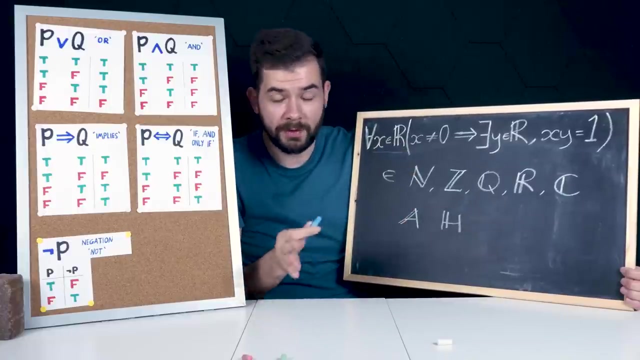 and we are saying: if X is not zero, then something about a real number, Y, such that X times Y equals one. Now we should feel like this is coming together. We know that every non-zero number has a partner number, a reciprocal, which we can multiply by to get to one. So the reciprocal of two is one half the. 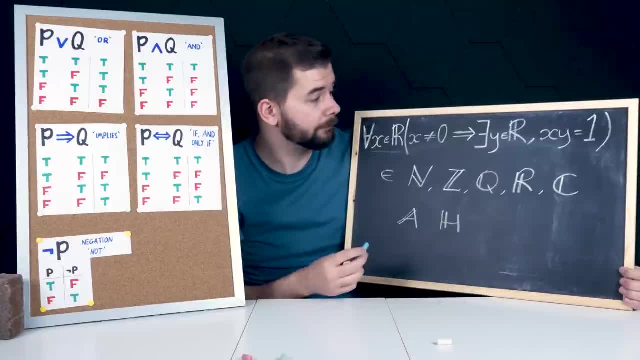 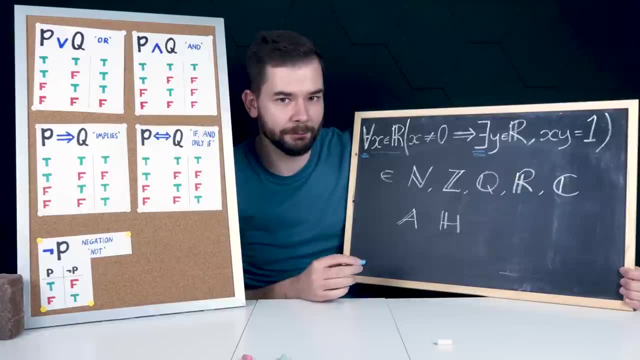 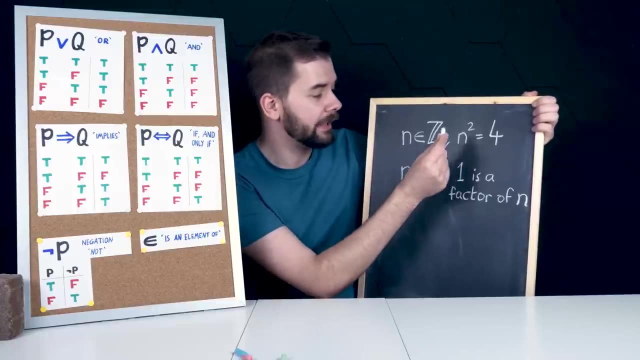 reciprocal of minus three quarters is minus four thirds, and so on. But what do these symbols here mean? Well, that's the final piece of the puzzle, which we will explore now. So consider these two propositions. The first is that N is an integer and N squared is equal to four. The second is that N is an integer and one. 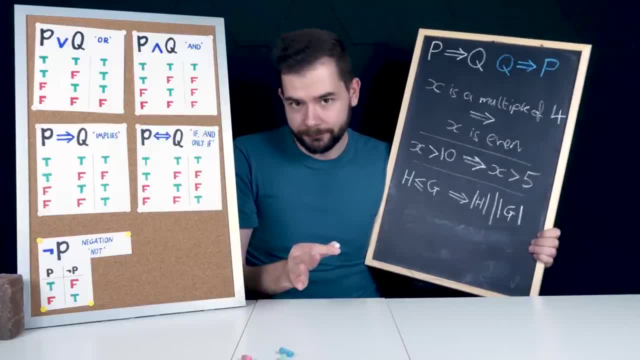 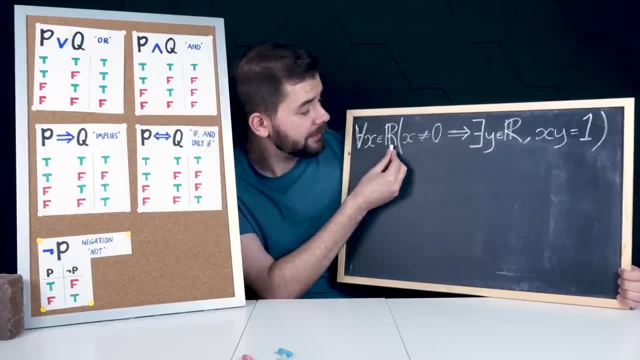 but not. every continuous function is differentiable, and so on. All of this is coming together for statements like we had at the start of the video. Here we're all also using this blackboard bold r to represent the set of real numbers and this e-shaped symbol. 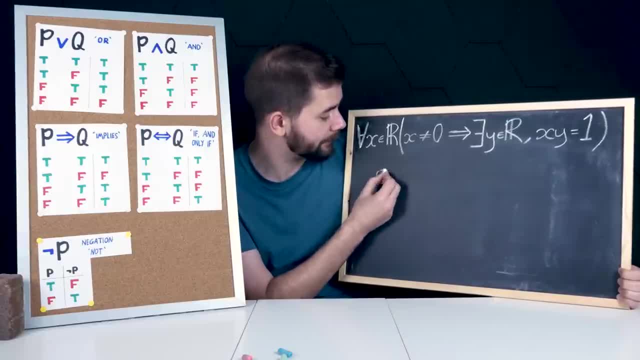 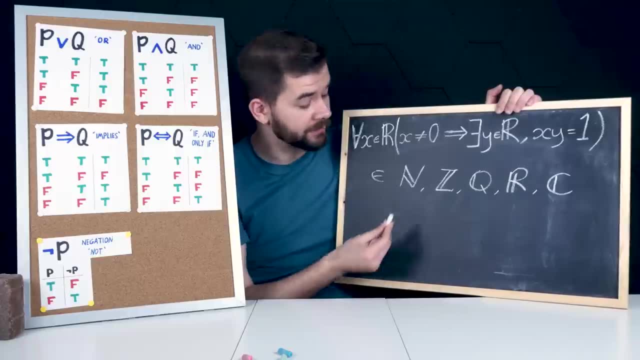 for membership. So this means is an element of, and we have a bunch of blackboard bold notations that we use to represent different sets of numbers. The common ones are: n for the natural numbers, that's positive integers, sometimes including zeros, sometimes not. there's really. 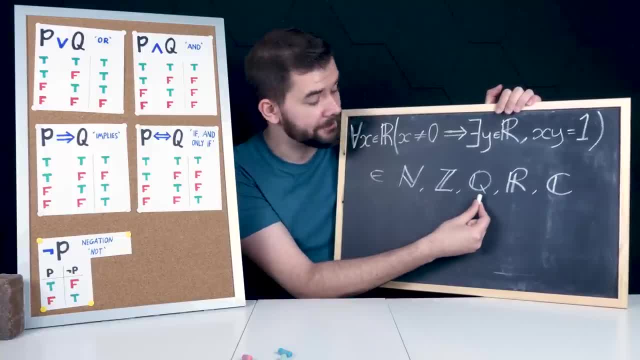 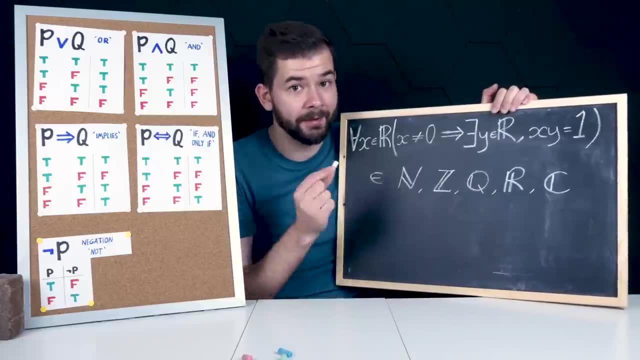 no consensus. z for the integers, the whole numbers. q for the rational numbers, the fractions. r for all the real numbers, c for the complex numbers. How are these sets actually defined? I have a short series of videos about that you should. 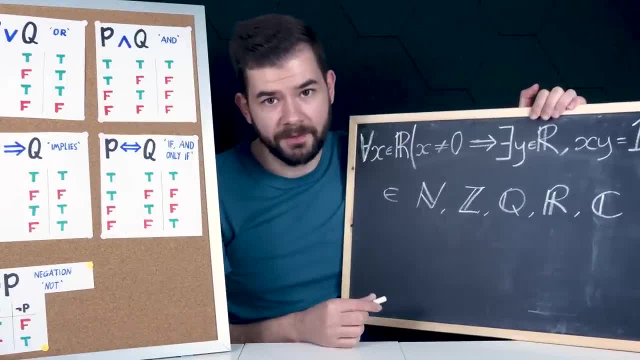 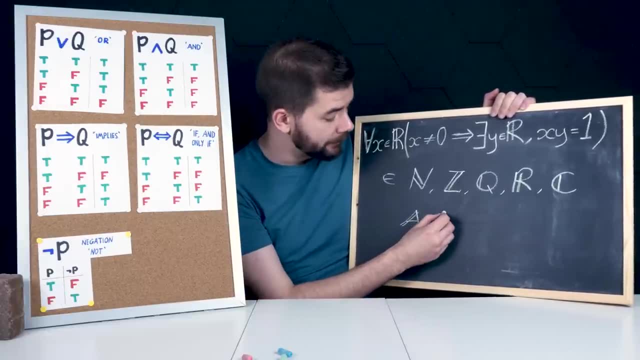 check it out. By short I mean there's four videos in the series. It is three and a half hours long, but you know There are other ones as well, but less common. You'll see a maybe for the algebraic numbers and blackboard bold h for the set of quaternions. But let's not worry about that now. 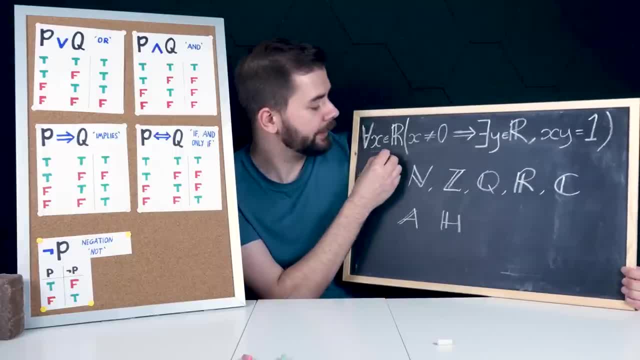 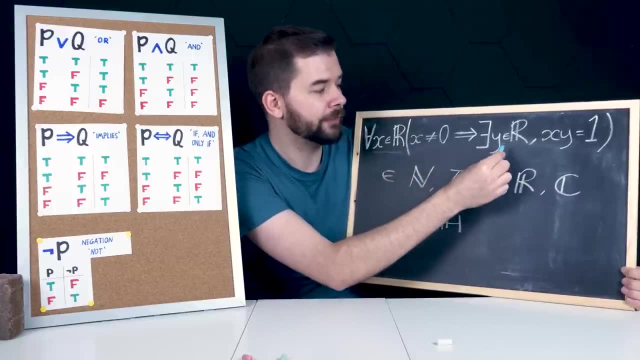 let's just focus on this statement up here. So we have something about a real number x and we are saying, if x is not zero, then something about a real number y, such that x times y equals one. Now we should feel like this: 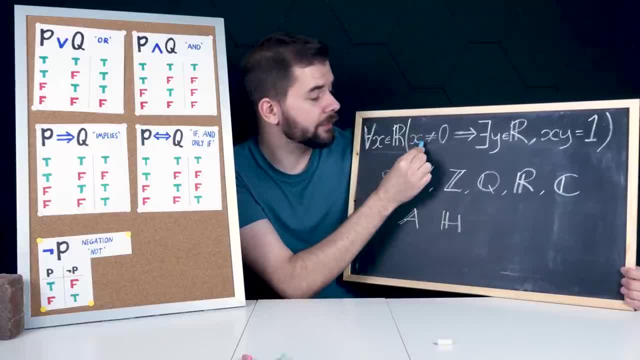 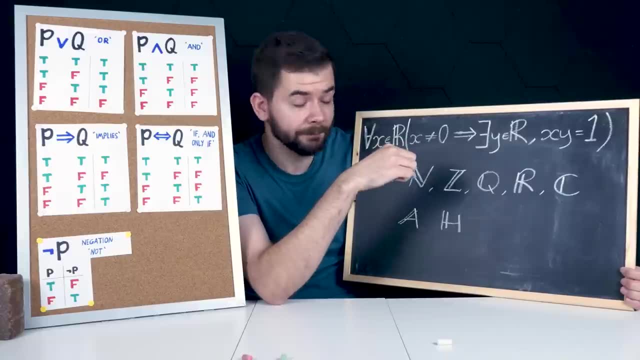 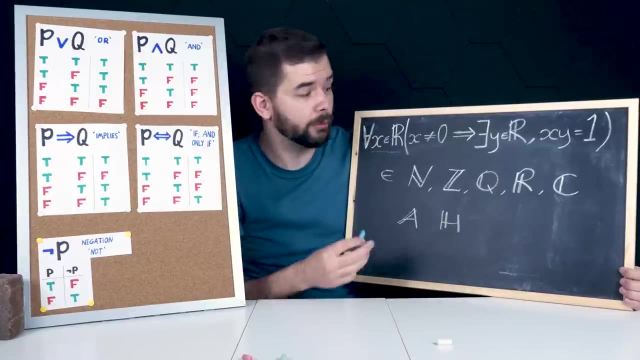 is coming together. We know that every non-zero number has a partner number, a reciprocal, which we can multiply by to get to one. So the reciprocal of two is one half, the reciprocal of minus three quarters is minus four thirds, and so on. But what do these symbols? 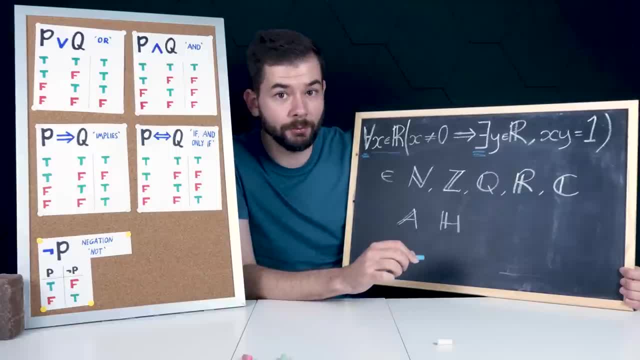 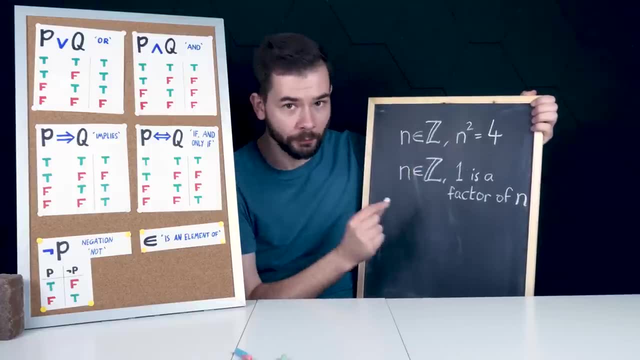 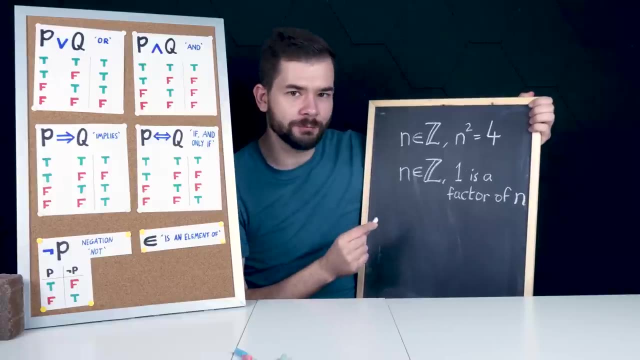 mean? Well, that's the final piece of the puzzle which we will explore now. So consider these two propositions. The first is that n is an integer and n squared is equal to four. The second is that n is an integer and one is a factor of n. What's the key difference between these two? 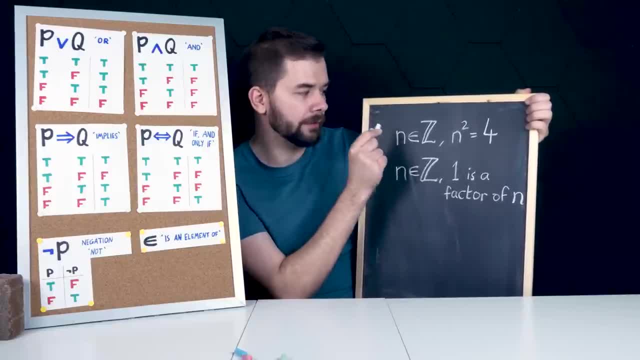 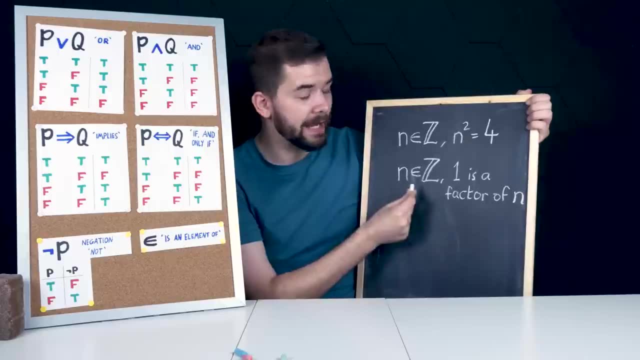 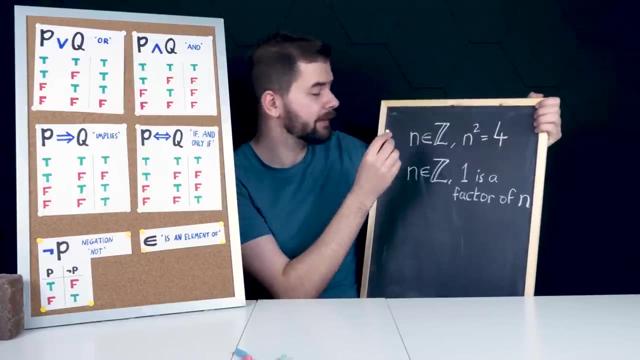 propositions. Well, hopefully we realise the first one is only true for certain values of n, whereas the second one is true regardless of which integer n we choose. Allow me to modify the first statement so that it is always true. So I'm going to add a symbol in. 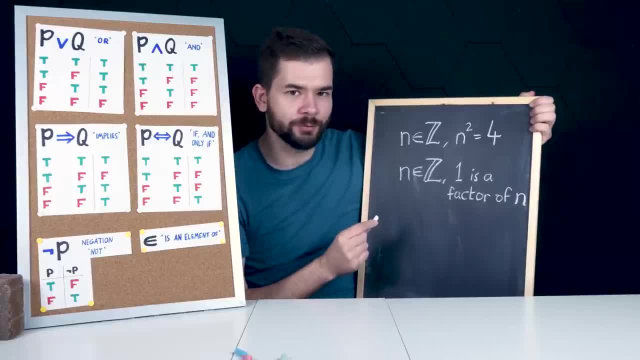 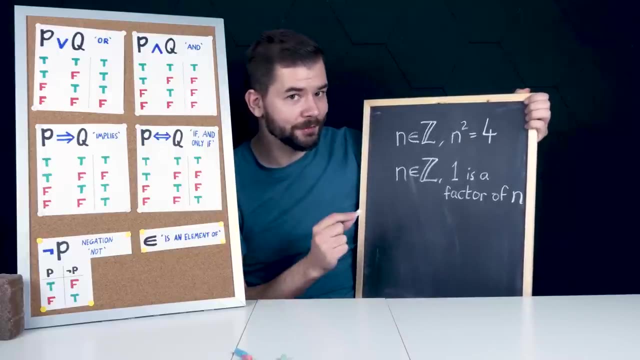 is a factor of N. What's the key difference between these two propositions? Well, hopefully we realize the first one is only true for certain values of N, whereas the second one is true regardless of which integer N we choose. Allow me to modify the first statement so that it is always true So. 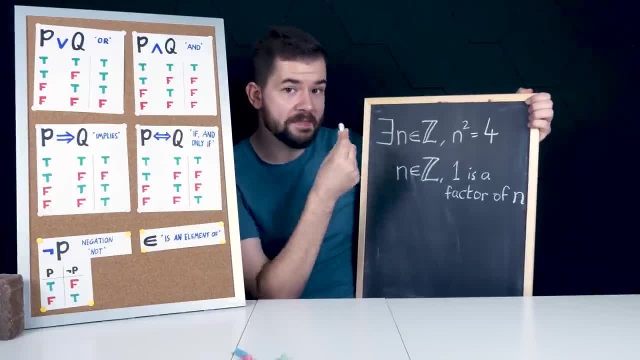 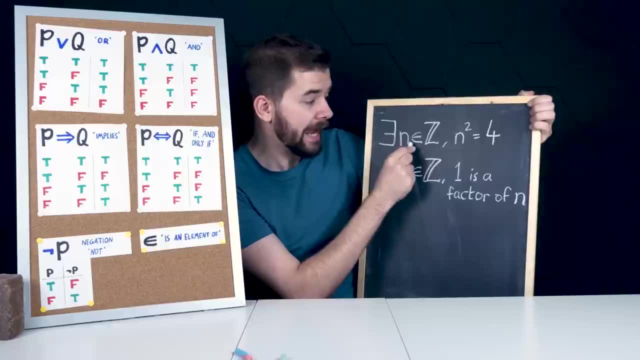 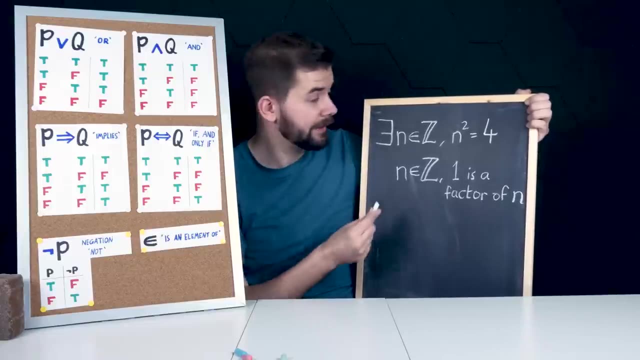 I'm going to add a symbol in here: There exists. So this statement is making the following claim: There exists an integer N with N squared equal to four, and this is a true statement. Such an integer does exist, namely N equals two. There are other examples as well, like: 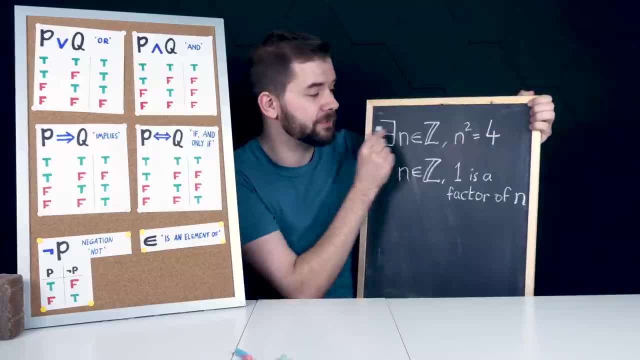 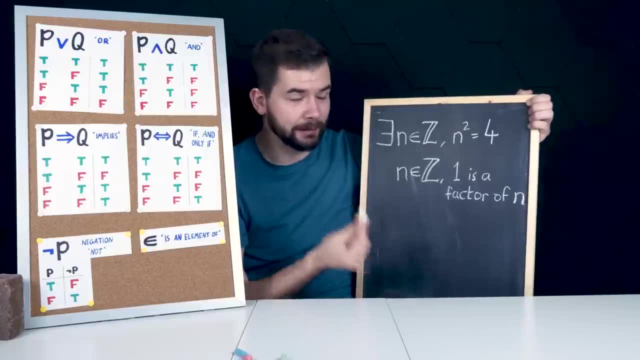 minus two, but I don't really care. In order for this first statement to be true, there just needs to be at least one value of N, for which is true, because this is making an existential claim- There exists an integer N with this property. Now let's modify the second one. 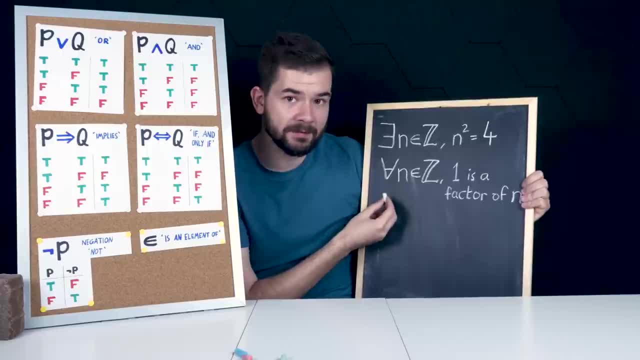 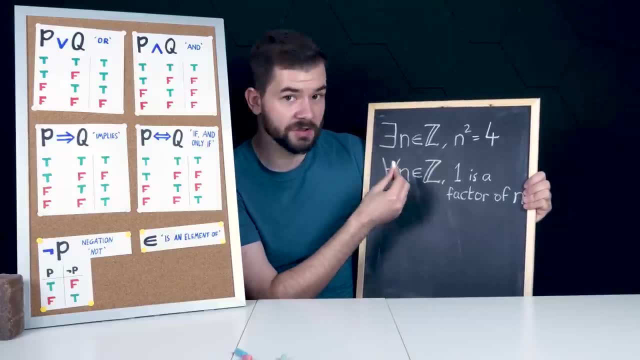 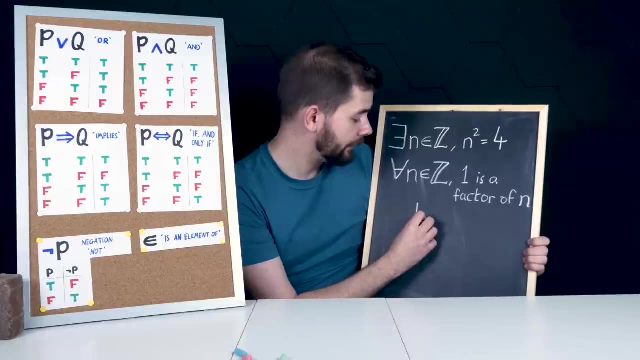 so it looks like how we usually write it. This inverted A means for all or for every. So this now is making the claim for all integers N. One is a factor of N, and we can prove that this one is true by pointing out that one multiplied by N. 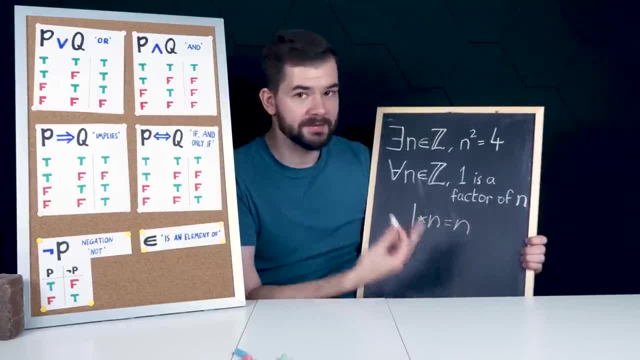 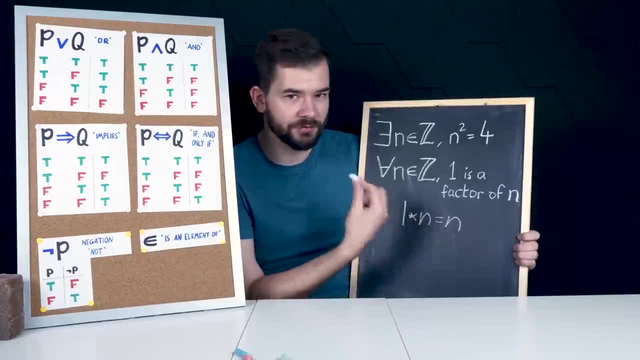 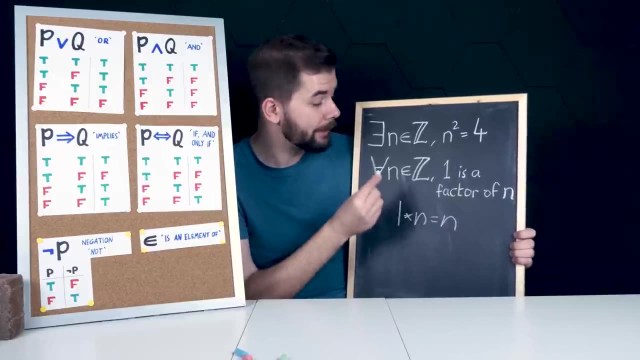 is equal to N, So one divides N. One is a factor of N, regardless of the value of N that we choose, And I need an algebraic proof or something like that in order to prove a statement like this true, because this is a universal claim. It's making a claim about all integers. I can't just list a. 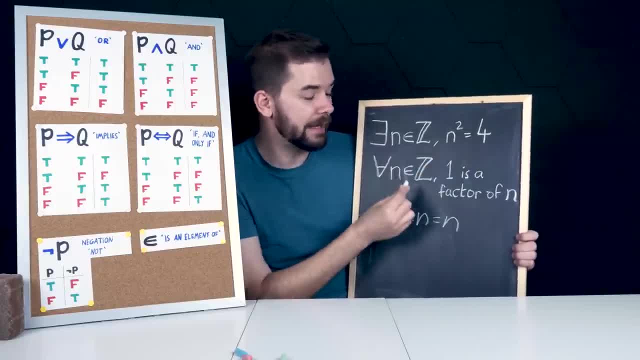 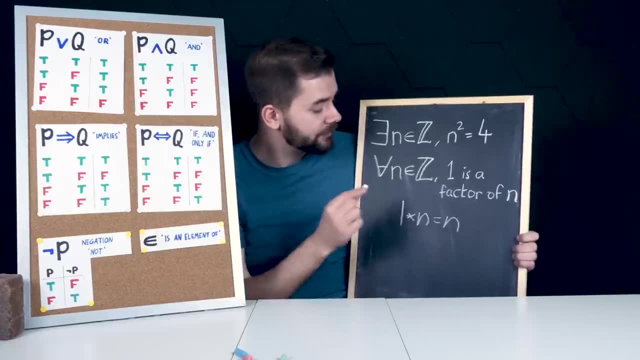 bunch of examples like I can to prove this one true, because it's making a claim about every possible integer. So to list examples would require us to list an infinite amount of examples, So I need an algebraic proof or something along those lines. These are called quantifiers and we 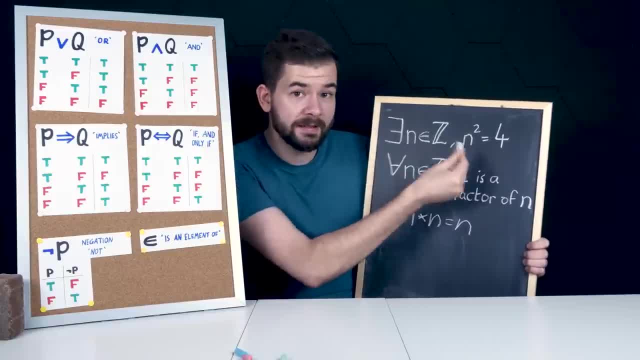 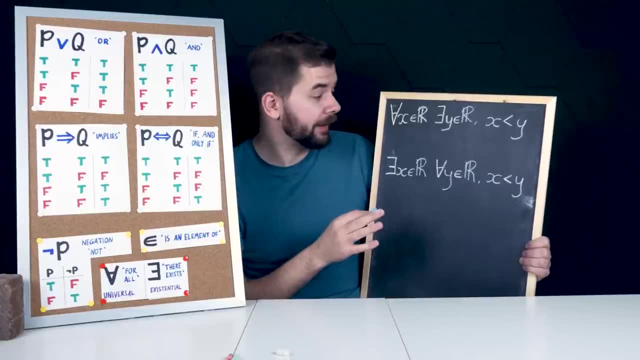 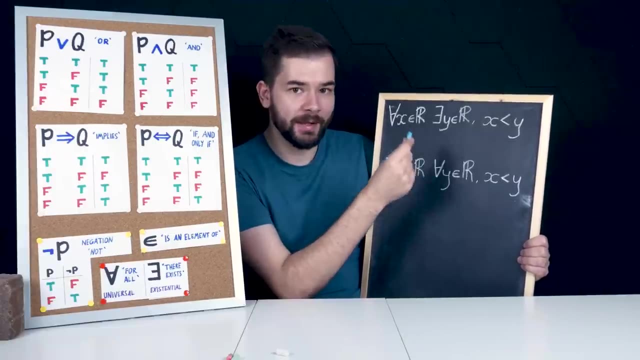 use them to make the distinction between whether we're talking about some of the things or all of the things. Let's see some examples of these in action. Let's look at some examples where we combine these quantifiers, because the order matters. And deep breath, we're almost there. So usually in statements like this, 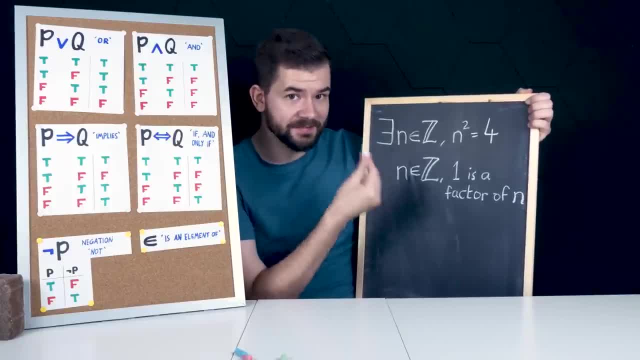 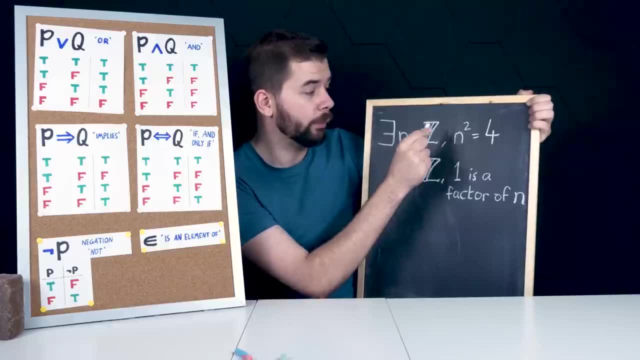 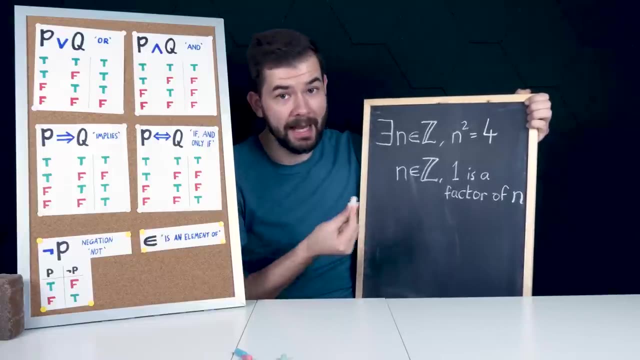 here This backwards e stands for there exists. So this statement is making the following claim: There exists an integer n with n squared equal to four, and this is a true statement. Such an integer does exist, namely n equals two. There are other examples as well, like minus two. 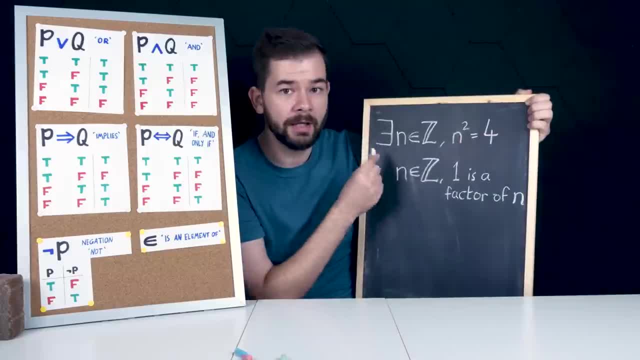 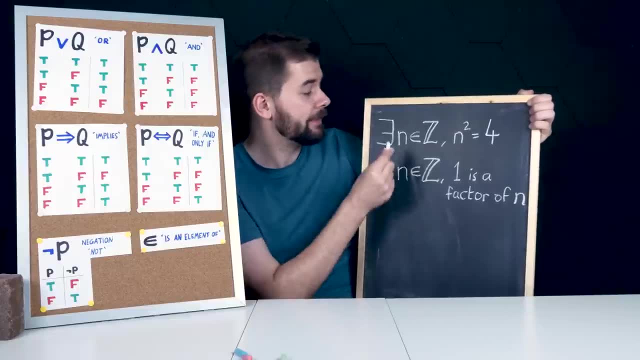 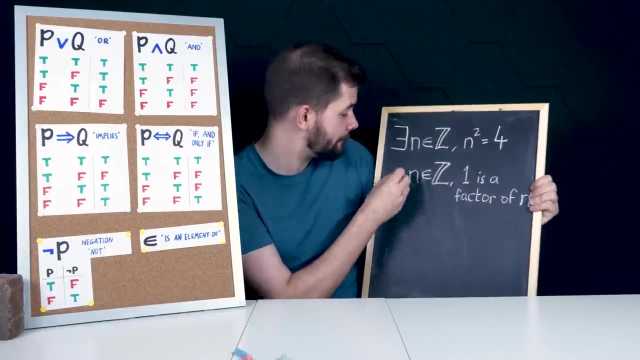 but I don't really care. In order for this first statement to be true, there just needs to be at least one value of n, for which is true, because this is making an existential claim that there exists an integer n with this property. Now let's modify the second one so it looks like how we usually write it. 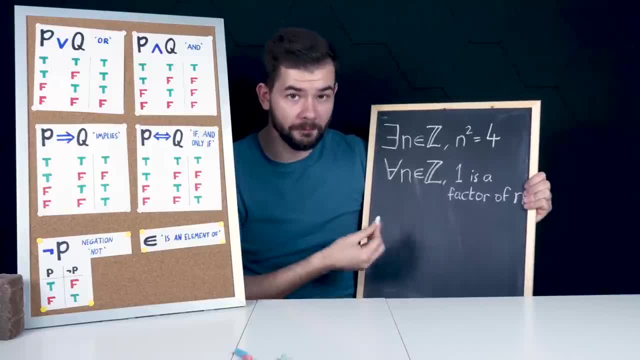 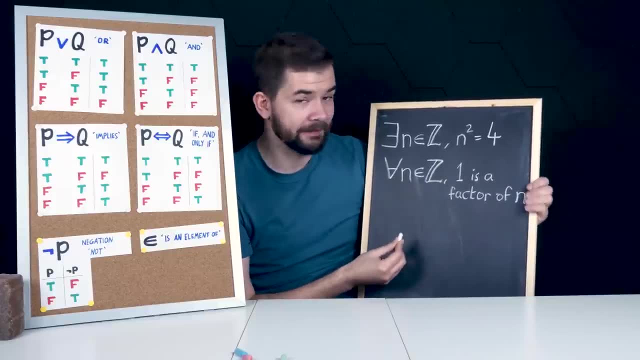 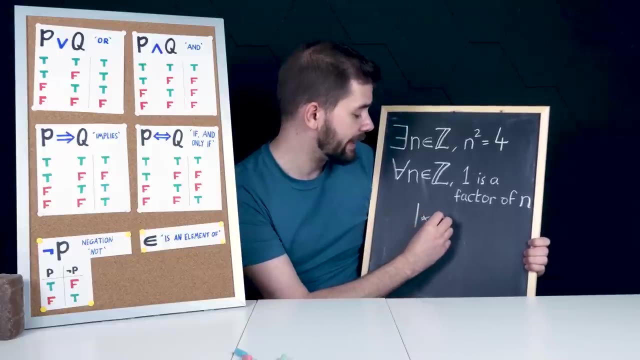 This inverted a means for all or for every. So this now is making the claim for all integers n. one is a factor of n, And we can prove that this one is true by pointing to the value of n. So I'm just pointing out that one multiplied by n is equal to n. So one divides n. 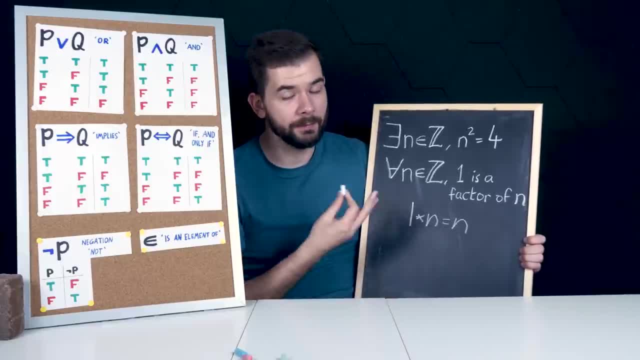 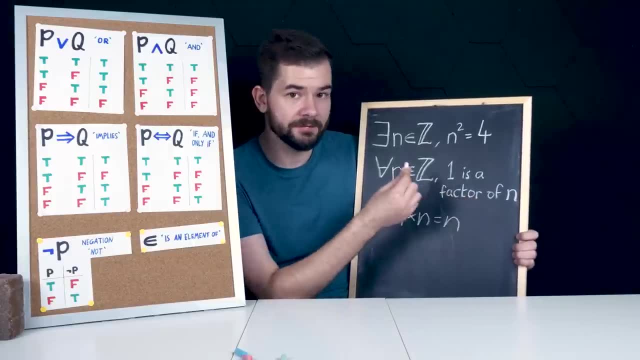 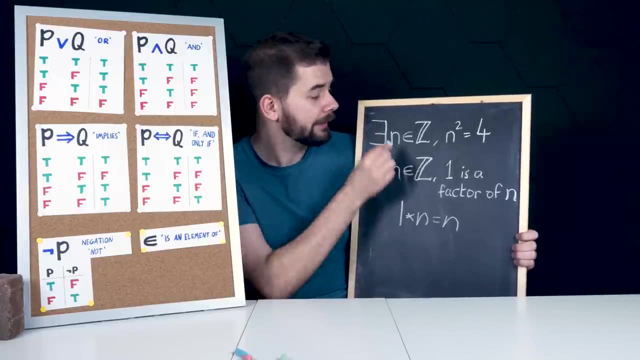 one is a factor of n, regardless of the value of n that we choose, And I need an algebraic proof or something like that in order to prove a statement like this true, because this is a universal claim. It's making a claim about all integers. I can't just list a bunch of examples like I can to prove. 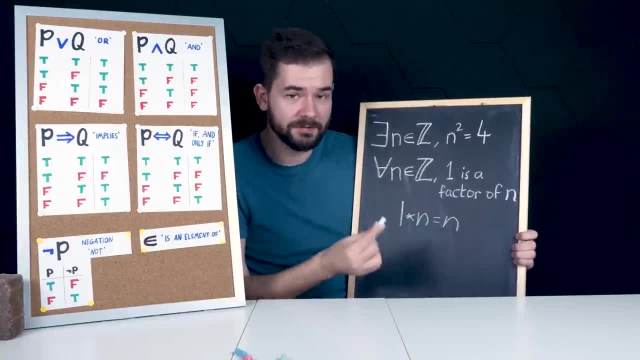 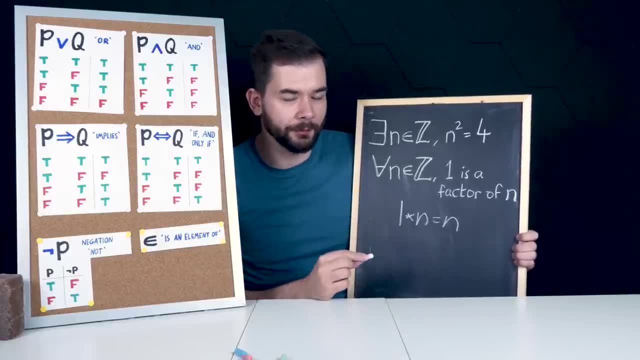 this one true, because it's making a claim about every possible integer. So to list the examples would require us to list an infinite amount of examples, So I need an algebraic proof or something along those lines. These are called quantifiers and we use them to make the 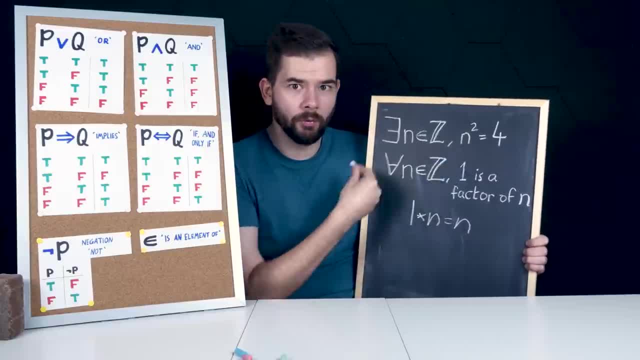 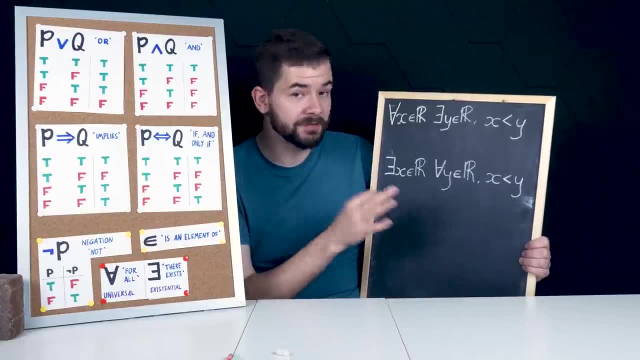 distinction between whether we're talking about some of the things or all of the things. Let's see some examples of these in action. Let's look at some examples where we combine these quantifiers, because the order matters. And deep breath, we're almost there. 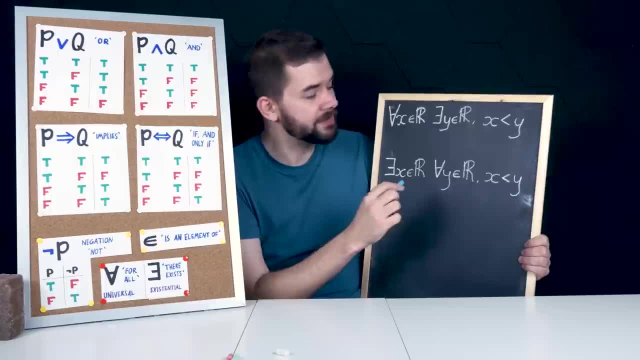 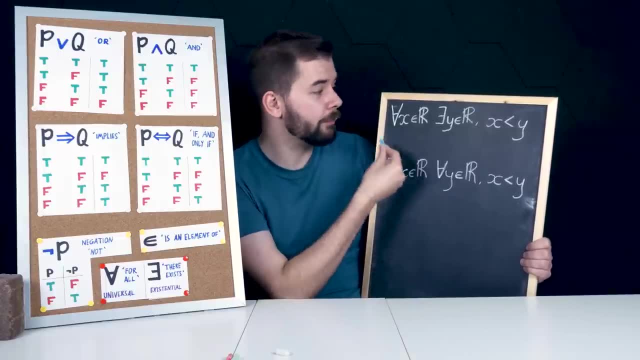 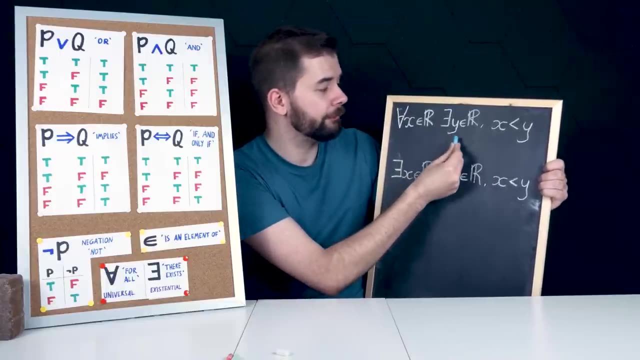 So usually in statements like this we have some brackets, or parentheses, if you call them that, that determine the order of priority, like it does with calculations. But if not, then we read the statement from left to right. So this is saying: for all real numbers x, there exists a real number y. 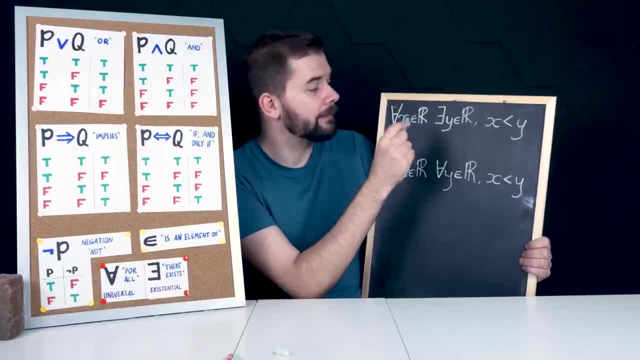 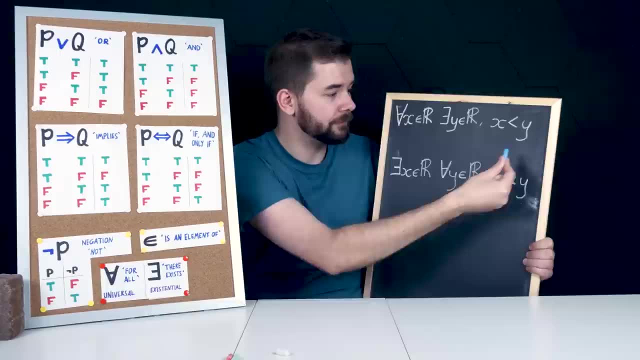 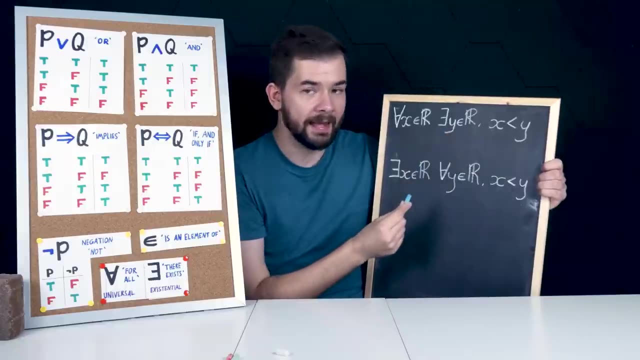 we have some brackets, or parentheses, if you call them that, that determine the order of priority, like it does with calculations. But if not, then we read the statement from left to right. So this is saying: for all real numbers x, there exists a real number y, with x less than y. So 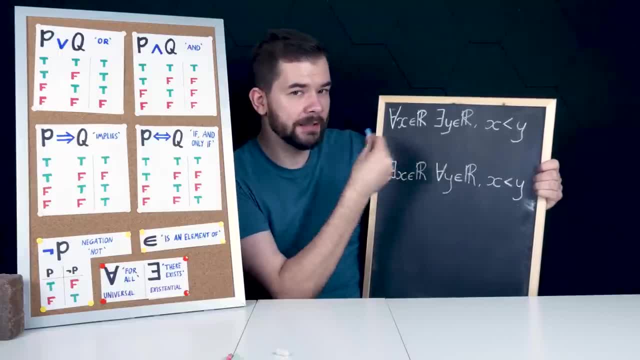 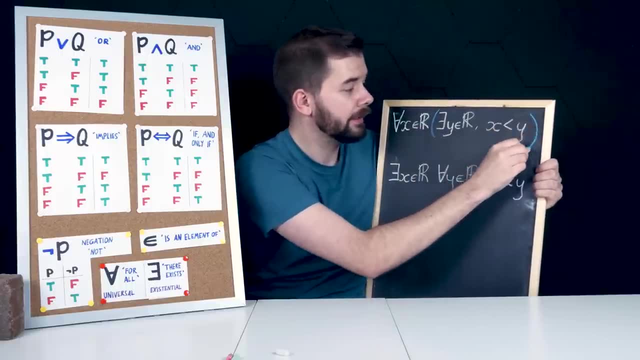 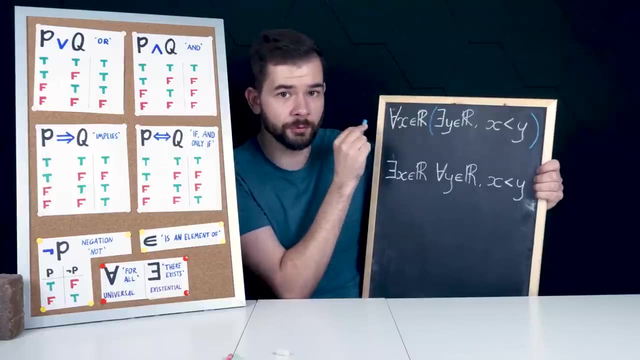 let's just break this down. I'm gonna put some brackets in here to really show exactly what's going on. So for all real numbers, x the proposition. this is true. So this is making a claim about all real numbers. For this statement to be true, it. 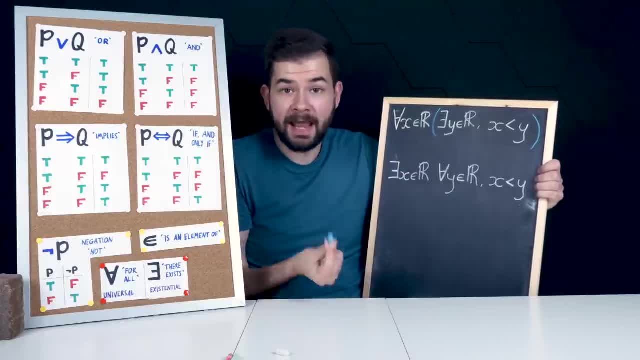 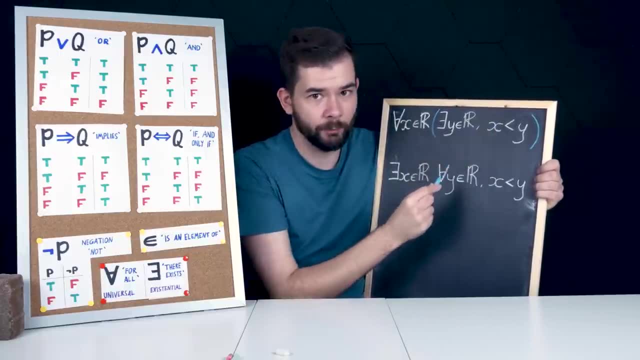 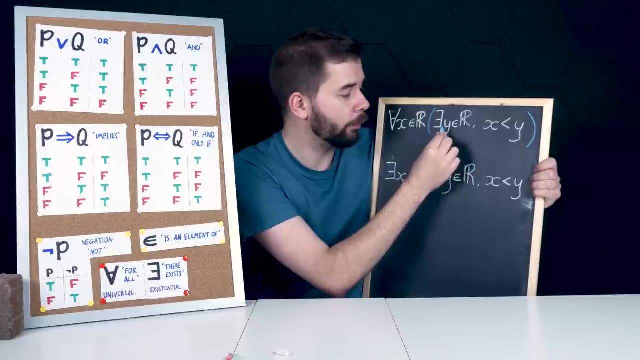 has to be true for every real number x. So for any real number x that we choose, is this proposition true? There exists a real number y, with x less than y. Well, this is true because no matter which x I choose, I can always find a y that is. 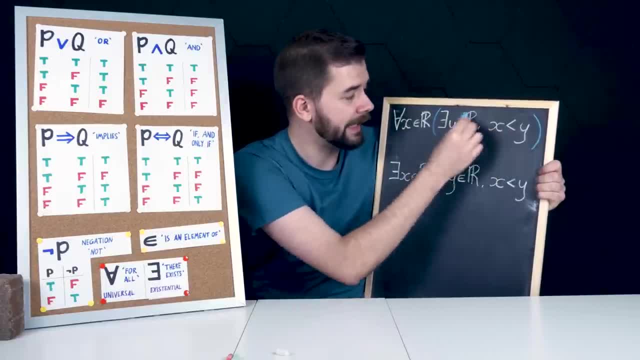 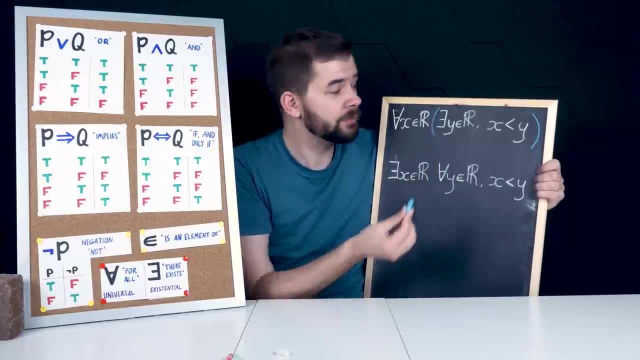 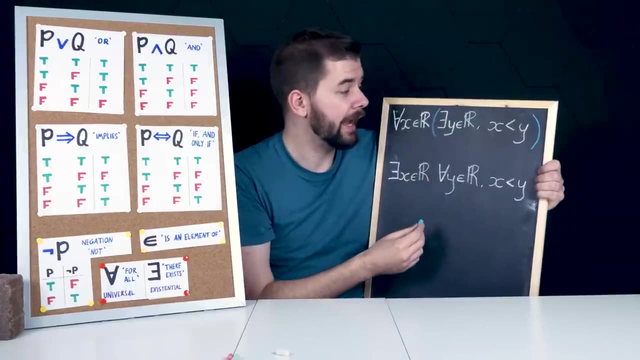 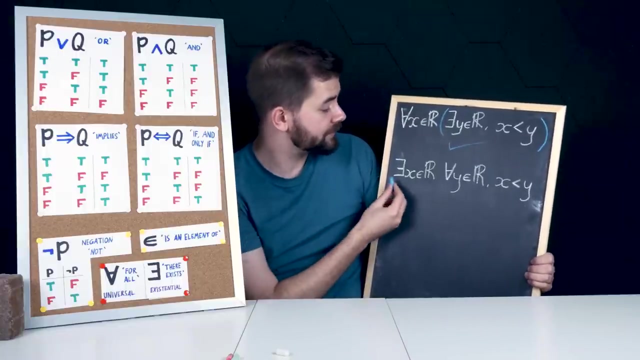 greater than x. and because this is an existential claim, we just have to find one specific example that works for any X. So, regardless of the X I choose, I can find a real number, y, For example, x plus 1, which is greater than than x. So this is a true statement. Contrast it with this one. So this one is saying there exists. 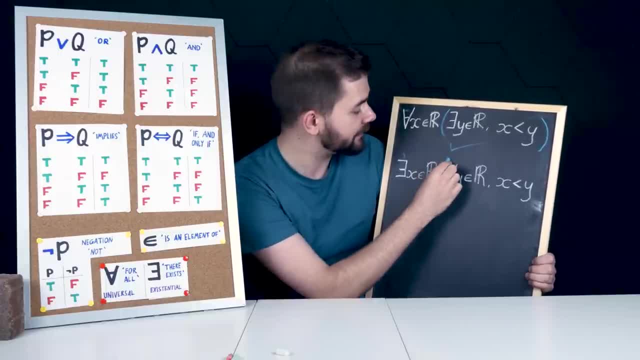 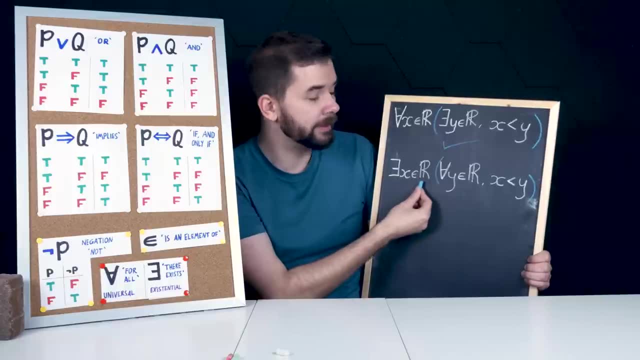 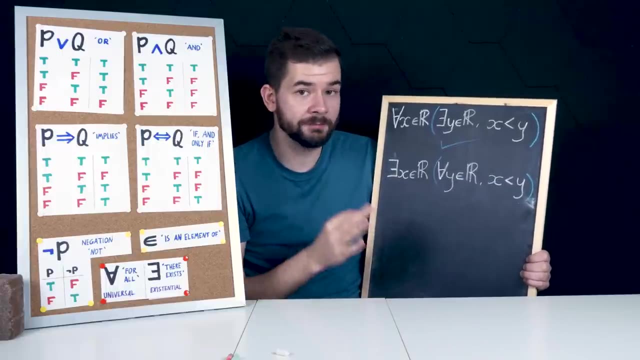 a real number x. So let's just pause here. I'm going to put the brackets in, because then you can really see what's going on. This is making an existential claim. There exists a real number x for which this whole thing here is true. For this statement to be true, it only has to be true. 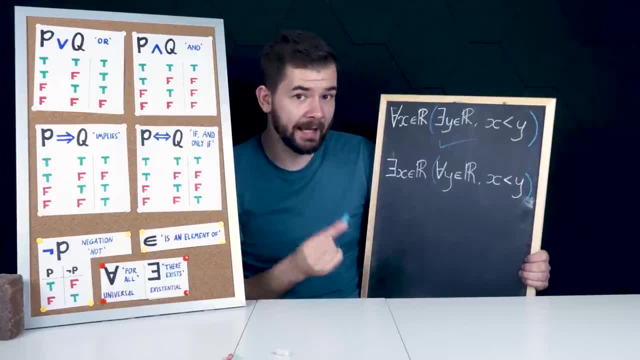 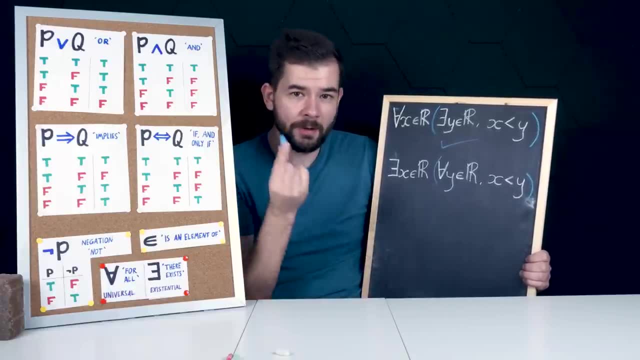 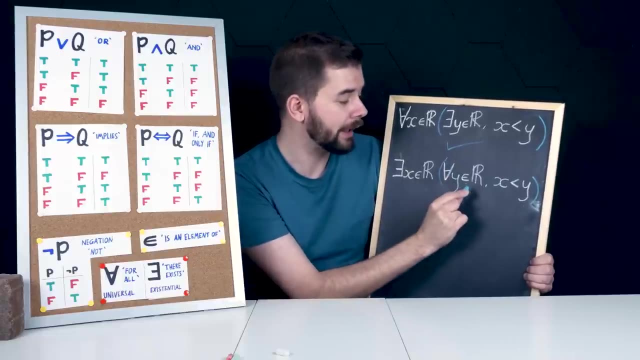 for one real number, for one example of x. So let's see if we can find one particular example of x that makes this statement true. So can we find a specific real number, x, for which the following is true For all real numbers: y, x is less than y, So we need to somehow find a special. 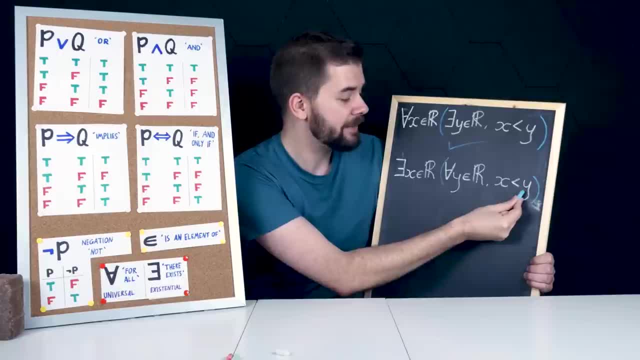 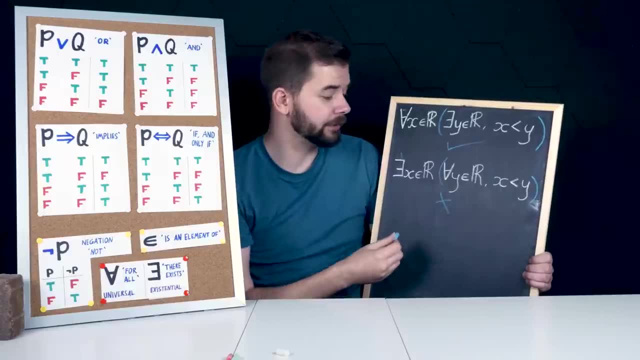 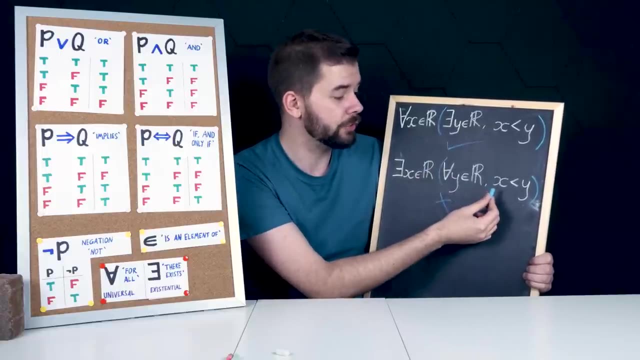 example of a real number, x, which is less than all real numbers, And this, I'm sorry, is false, because no such real number x exists. We can prove it false by a counterexample, Regardless of the x we try to choose, if we choose, y is equal to x minus one, that's always less than. 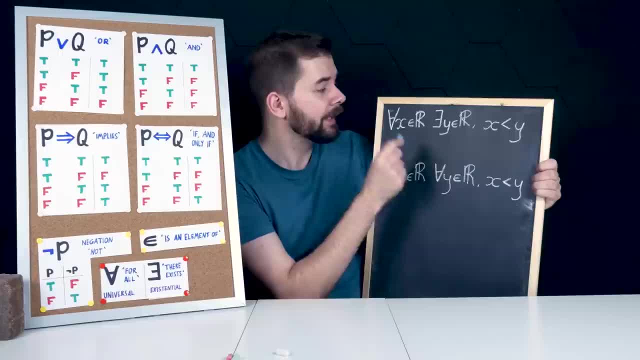 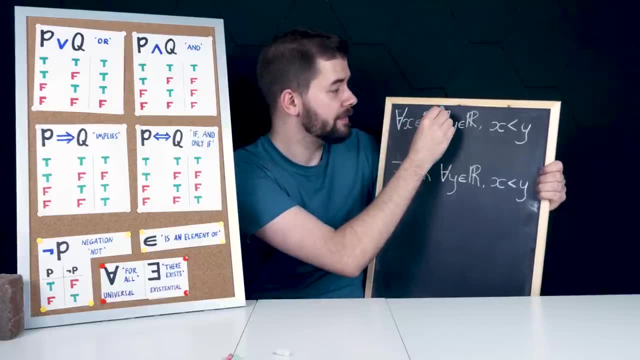 with x less than y. So let's just break this down. I am going to put some brackets in here to really show exactly what's going on. So, for all real numbers x, the proposition. this is true. So this is making a claim about the order of priority. So this is saying: for all real numbers x there exists. 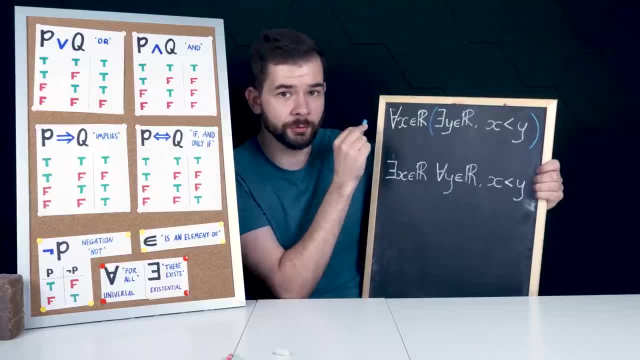 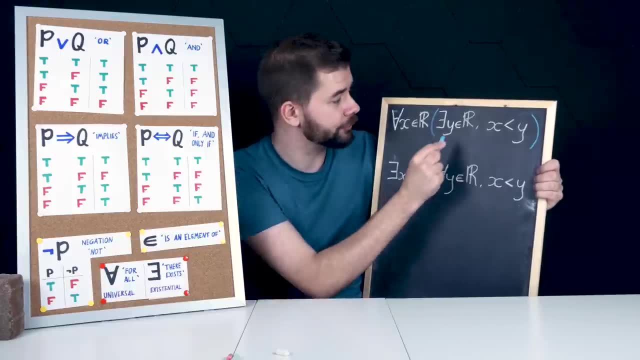 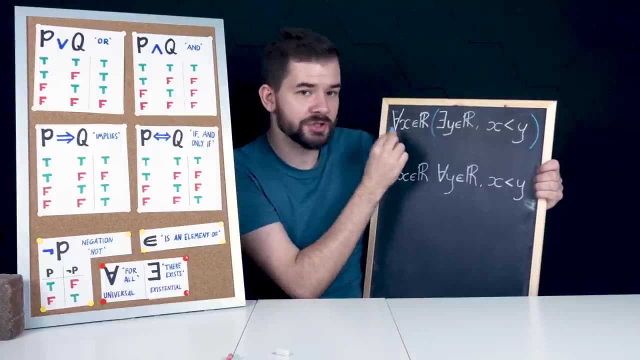 a real number, y with x less than x. Now, when I do this, it's the same thing over and over and over again. So if you look at this before- and this is apparently what I do for all real numbers x- Well, it's also like I've 그렇게. 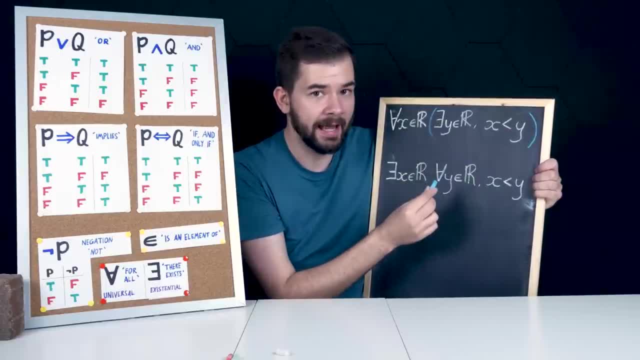 false here for real numbers x, but this is something I always have to do in order to make this statement be true, So I can twist this space down slightly. and this is because for real numbers x, the rule lies in that if i x, that there's no equal to y, so I'm speaking all real numbers by several variables to makes this statement to be true. So, for any number x that we choose, is this proposition true? There exists a real number, y, with x less than y. Well, this is true because no matter which x I choose, i can always find a y that 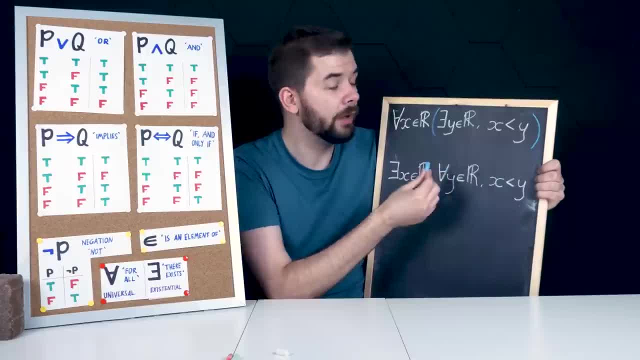 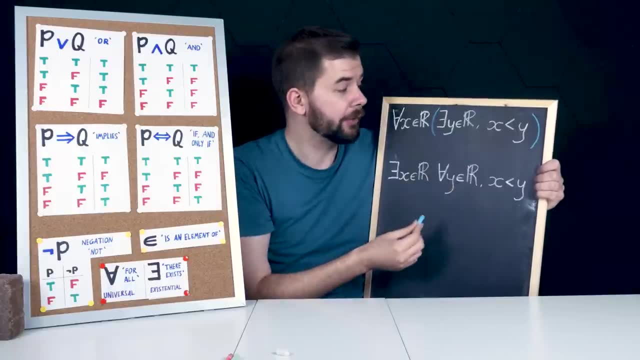 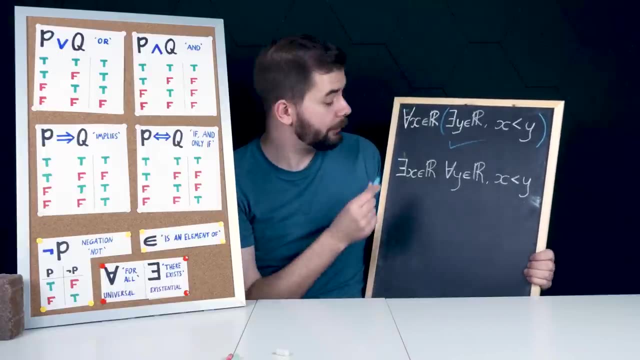 is greater than x. And because this is an existential claim, we just have to find one specific example x. So, regardless of the x I choose, I can find a real number, y, for example, x plus 1, which is greater than x. So this is a true statement. Contrast it with this one. 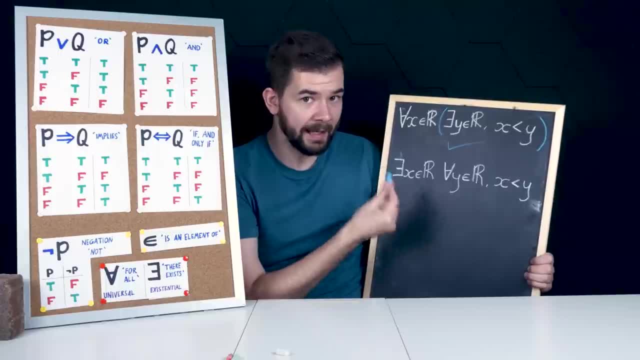 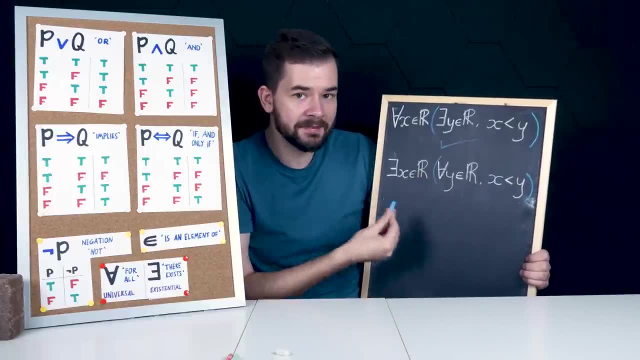 So this one is saying there exists a real number x. So let's just pause here. I'm gonna put the brackets in, because then you can really see what's going on. This is making an existential claim: There exists a real number x, for which 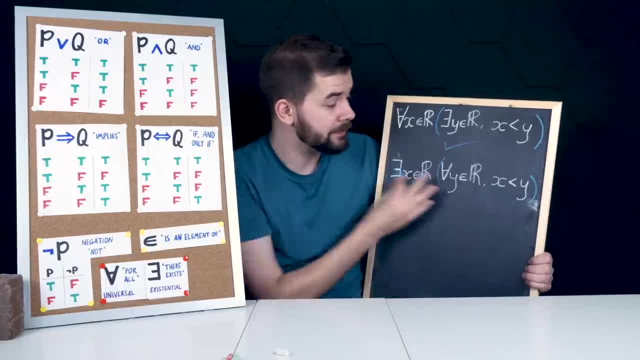 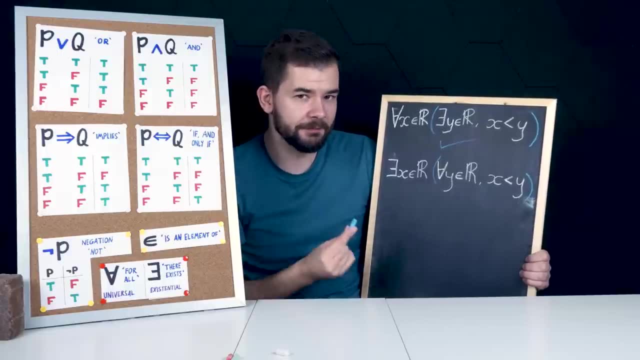 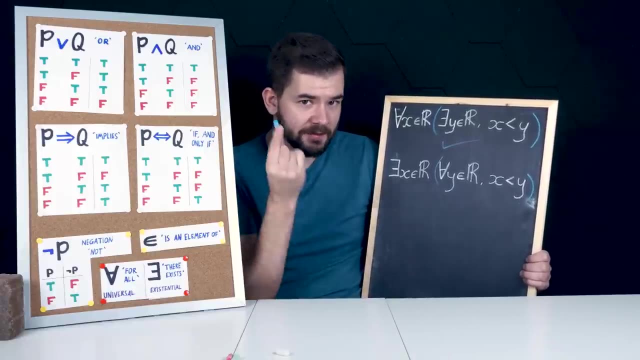 this whole thing here is true. For this statement to be true, it only has to be true for one real number, for one example of X. so let's see if we can find one particular example of X that makes this statement true. So can we find a specific? 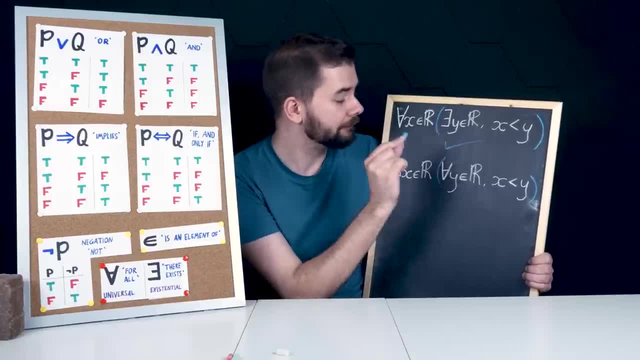 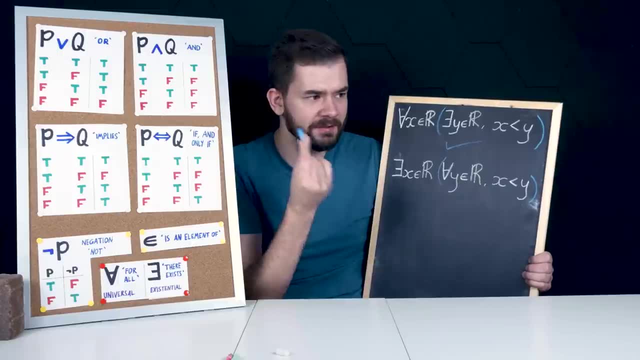 real number x, for which the following is true: For all real numbers y: x used is only one number. For all real numbers z, an existential claim. w is a true statement- is less than y, So we need to somehow find a special example of a real number x which is less. 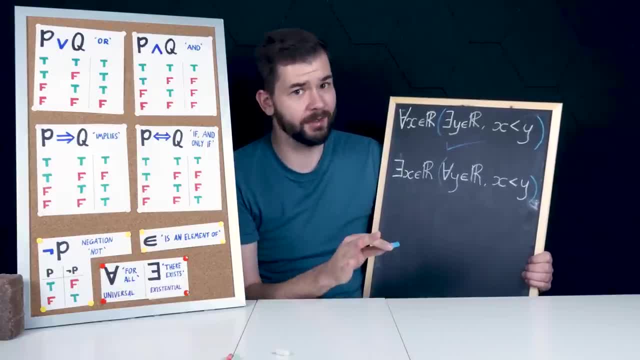 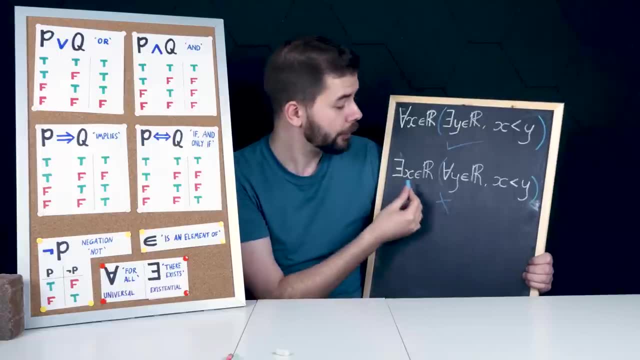 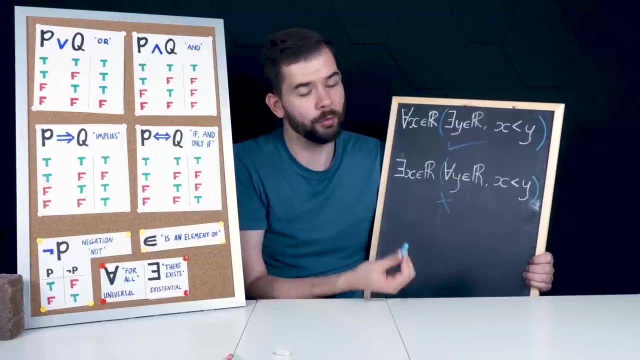 than all real numbers, And this, I'm sorry, is false, because no such real number, x, exists. We can prove it false by a counterexample: Regardless of the x we try to choose, if we choose y is equal to x minus 1, that's always less than x. So we can always find a real number that breaks this. 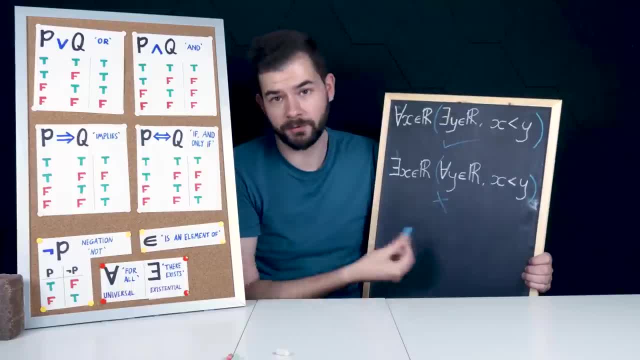 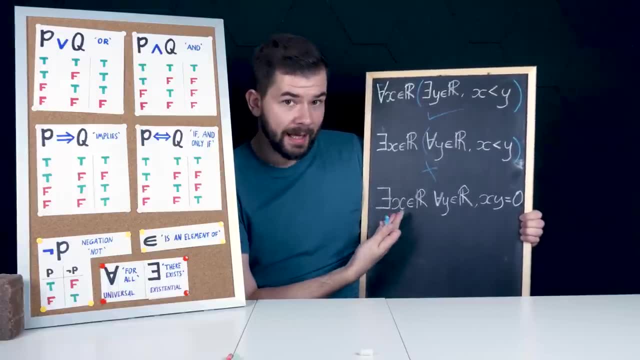 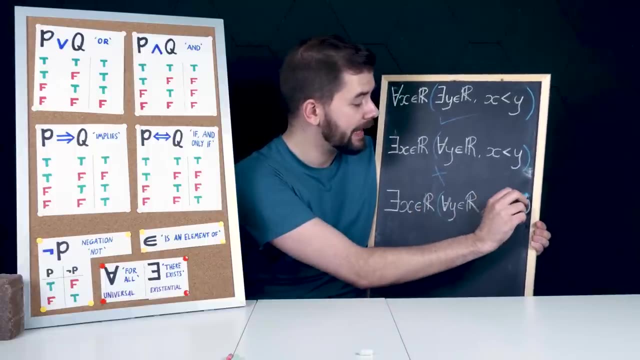 condition here. So it's not true for all real numbers y, and so the entire proposition is false. And let's contrast it with this statement: here There exists a real number x, such that for all real numbers y, x times y equals 0. So once again, this is making an existential claim. 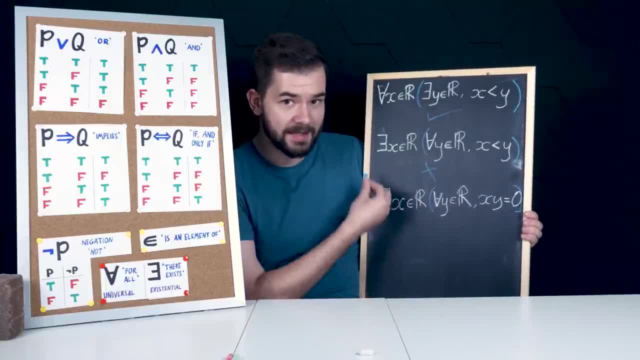 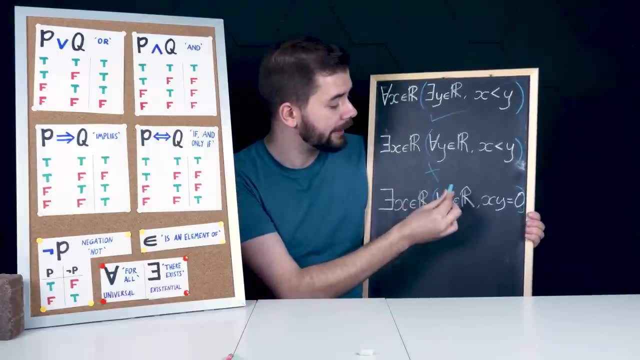 if I could draw that bracket in. There exists a special real number, x, so we just need to find one specific value of x for which the following holds: For all y real numbers: x times y equals 0. And we can find a specific value of x. 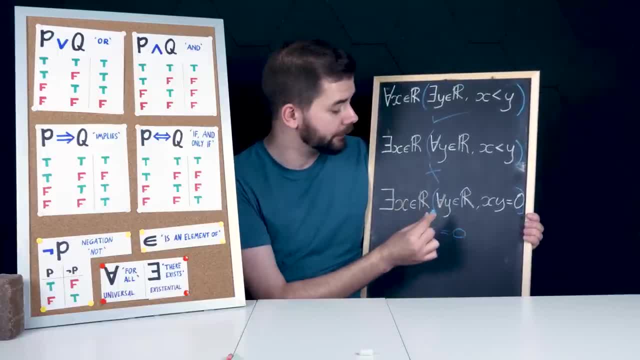 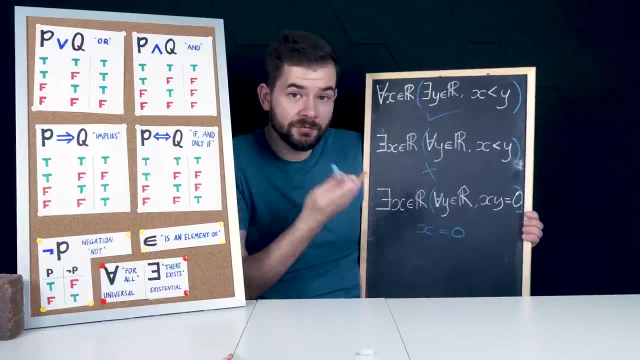 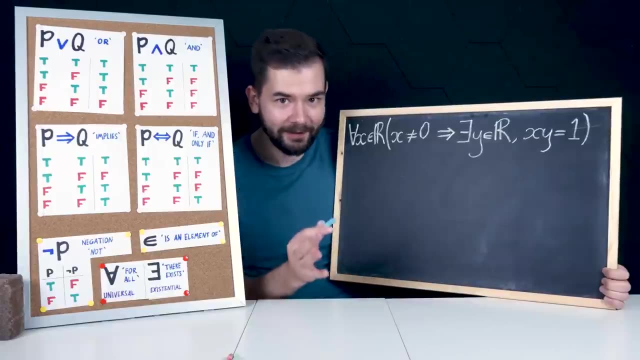 x equals 0.. For all y- that's a real number- x times y will be 0 in the case that x equals 0. This is an existential claim. It is only claiming that such a real number exists. So by finding one example, we prove the proposition is true. Now let's finally examine the claim from the start. 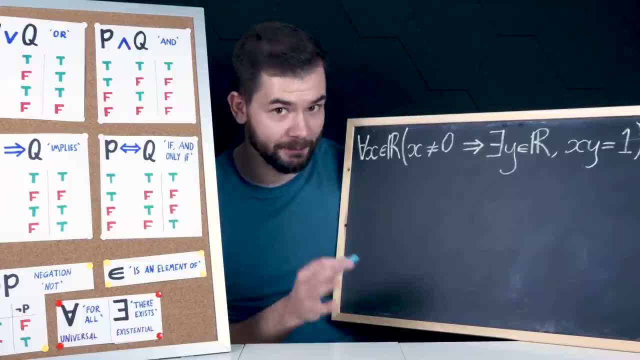 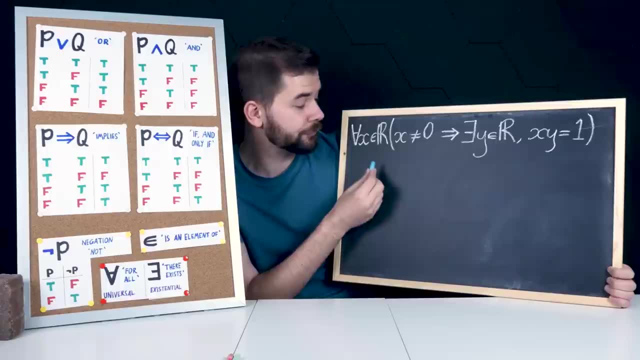 of the video. Are you ready? I'm ready. I've been filming a long time and I'm quite hungry. So this says for all real numbers: x. so for this to be true, it has to be true for every real number. 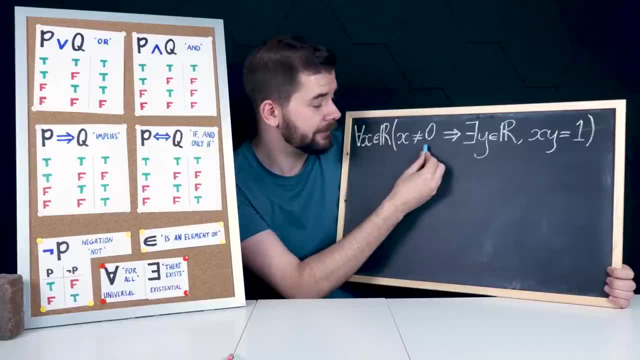 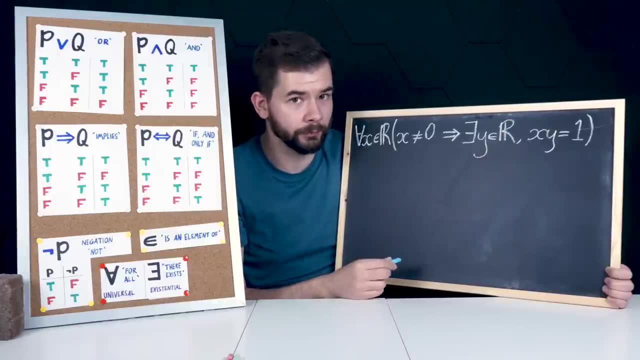 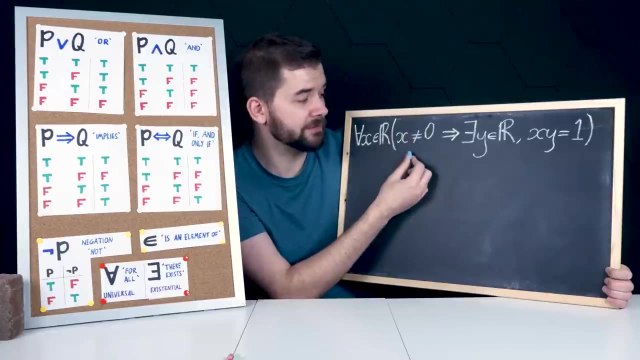 So, for every real number x, if x is not 0, then there exists a real number, y, with x, y equal to one. So in order to prove this true, we have to say that whenever it is the case that x is not 0,. 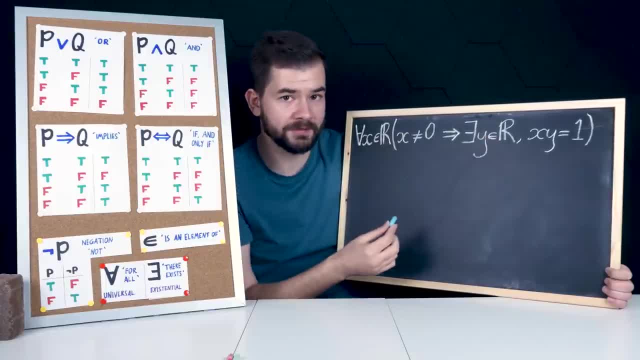 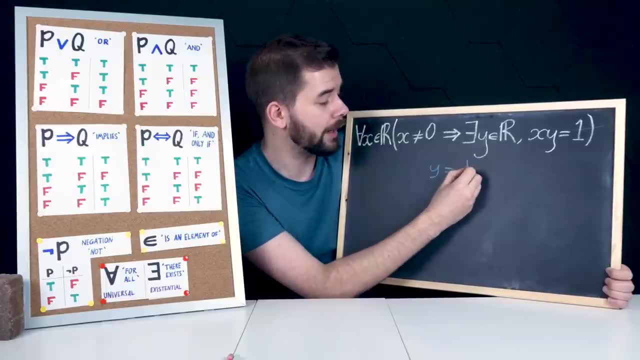 then it是 that the case that we can find a y with the property that x times y is 1, and this is true because whenever x is 0, we can choose, y is the reciprocal of x, and boom. But before we wrap up, one last. 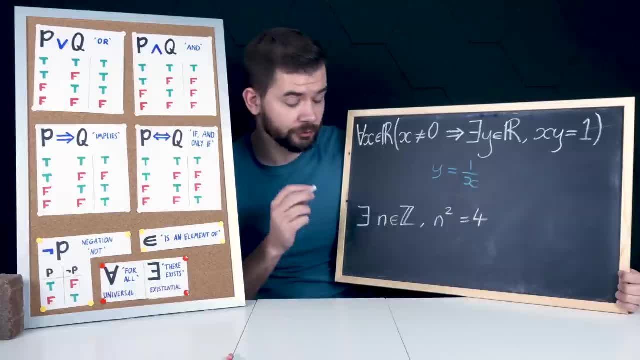 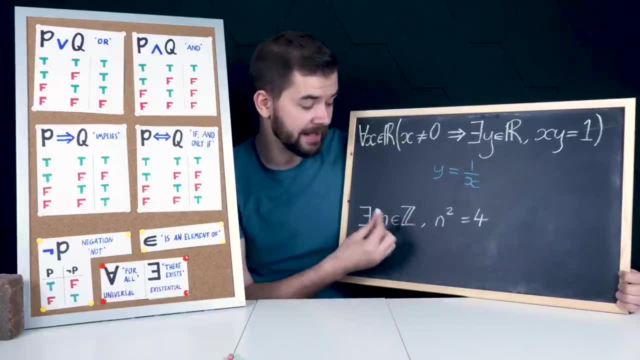 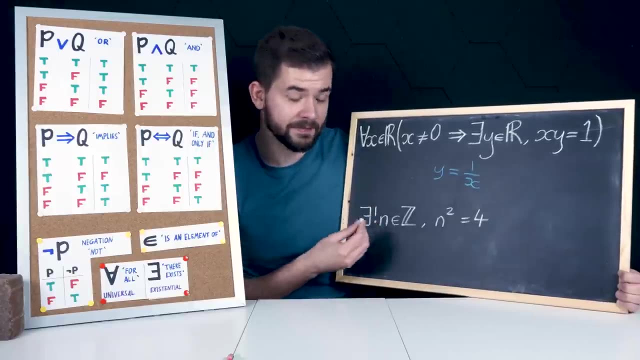 final bit of symbolic logic that you might encounter on your travels. So this is a different type of existential quantifier. Remember this one. here there exists an integer n such that n squared equal to 4.. If I add an exclamation mark here, then what this now says is: there exists an integer n. 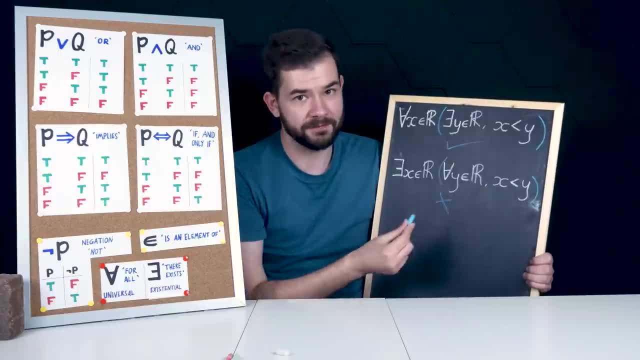 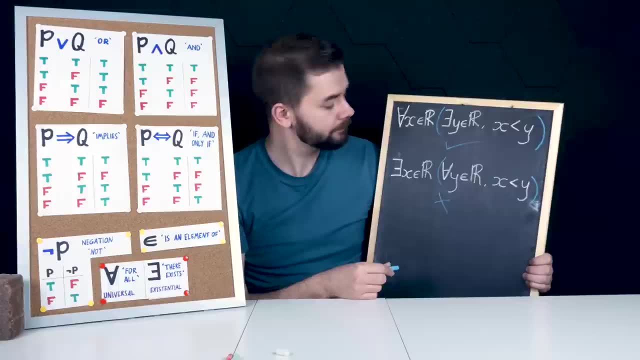 x, So we can always find a real number that breaks this condition here. So it's not true for all real numbers y, And so the entire proposition is false. And let's contrast it with this statement. here There exists a real number x, such that for all real numbers y, x is less than x. So this: 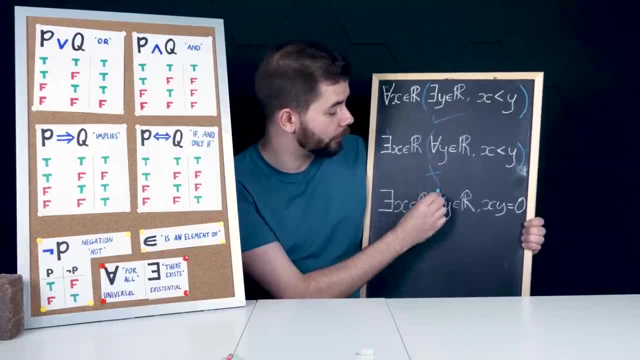 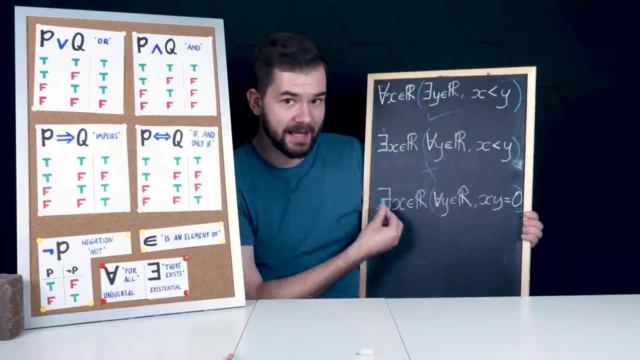 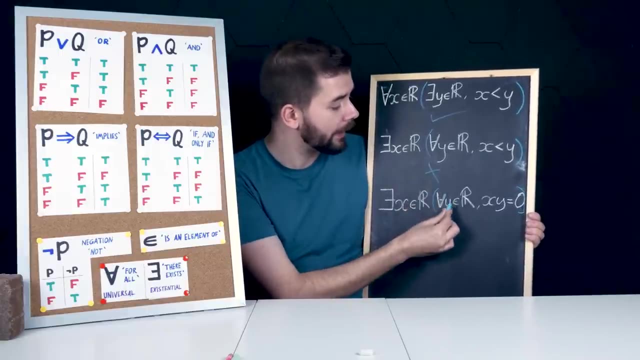 means that for all real numbers, y, x times y equals zero. So once again, this is making an existential claim. if I could draw that bracket in, There exists a special real number, x, so we just need to find one specific value of x for which the following holds: For all y real numbers, 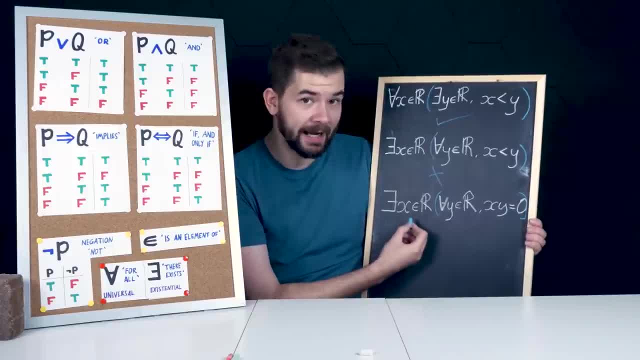 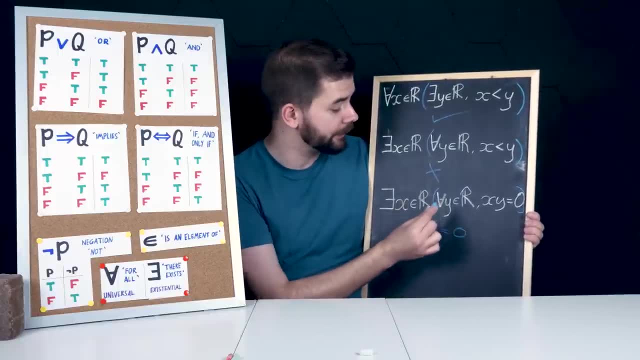 x times y equals zero. And we can find a specific value of x. x equals zero For all y. that's a real number. x times y will be zero in the case that x equals zero. This is an existential claim. It is. 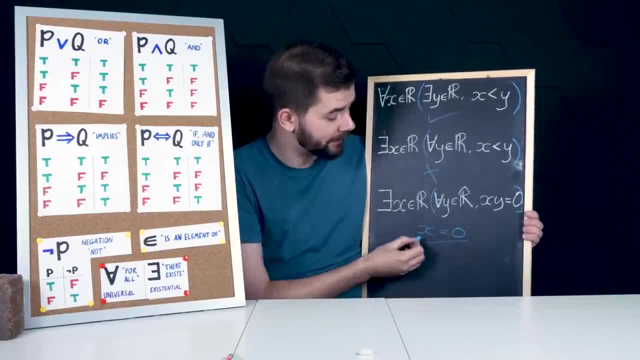 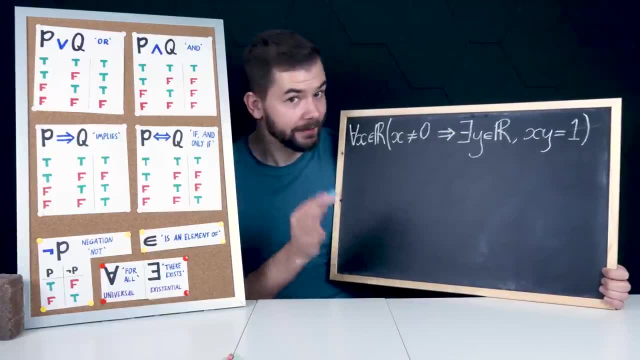 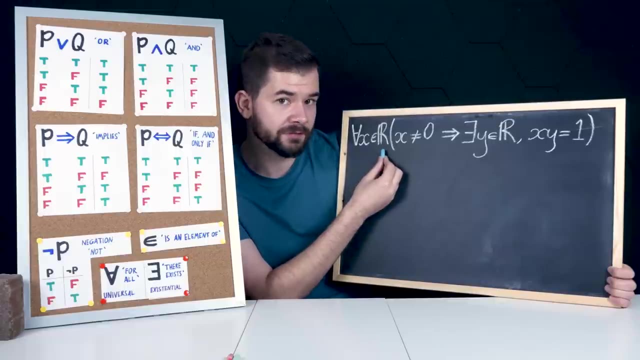 only claiming that such a real number exists. So by finding one example, we prove the proposition is true. Now let's finally examine the claim from the start of the video. Are you ready? I'm ready, I've been filming a long time and I'm quite hungry. So this says, for all real numbers, x. So for this. 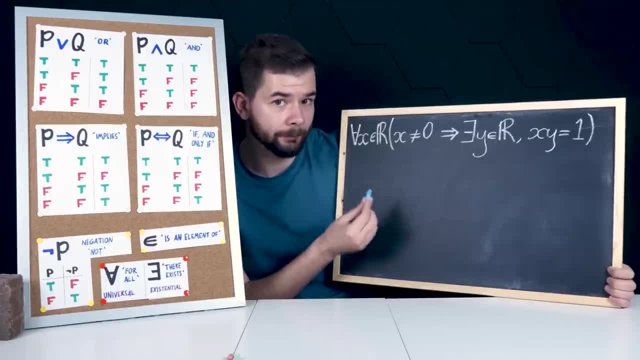 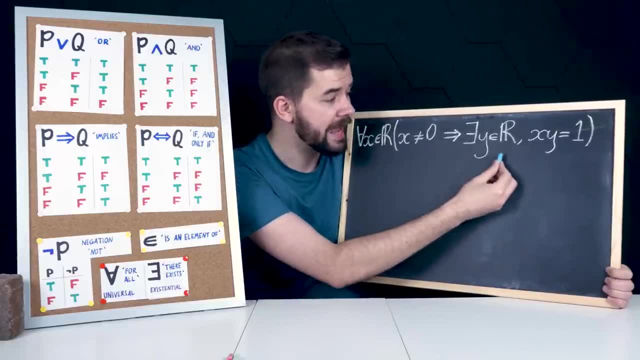 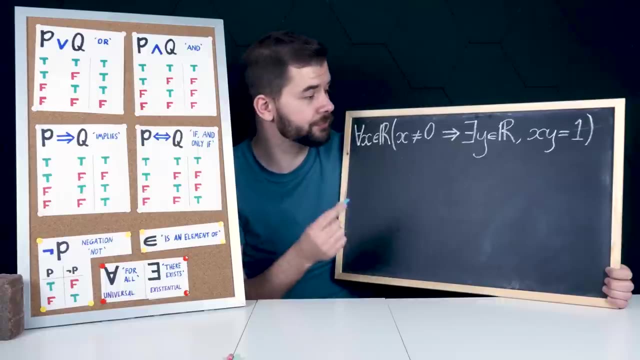 to be true. it has to be true for every real number. So for every real number, x. if x is not zero, then there exists a real number, y, with x, y equal to one. So in order to prove this true, we have to say that whenever it is the case that x is not zero, then it is the 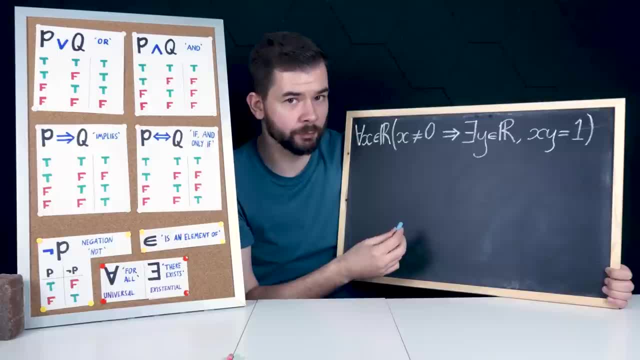 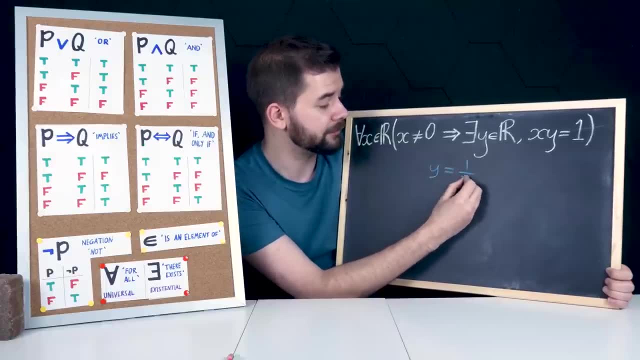 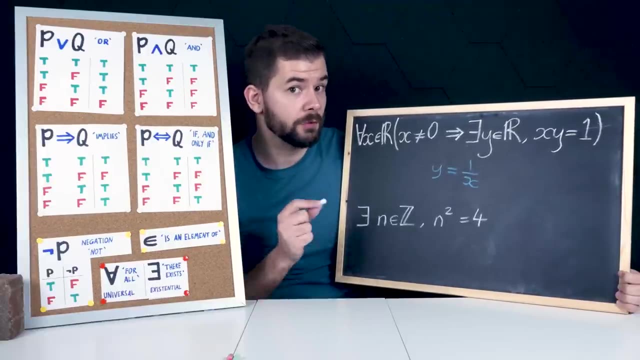 case that we can find a y with the property that x times y is one. And this is true because whenever x is zero, we can choose. y is the reciprocal of x and boom. But before we wrap up, one last final bit of symbolic logic that you might encounter on. 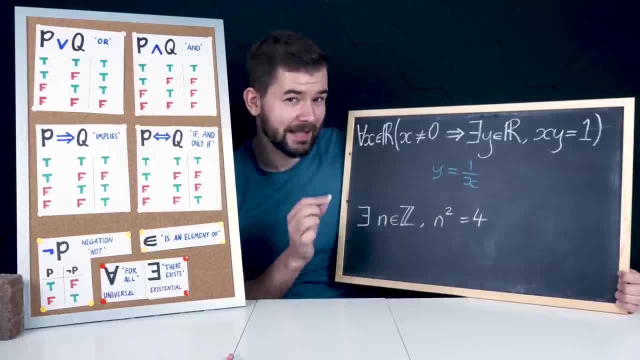 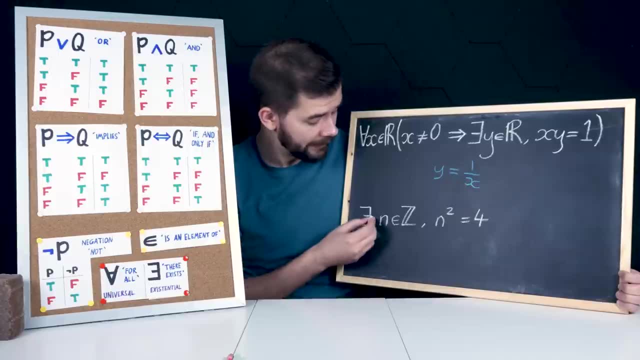 your travels. So this is a different type of existential quantifier. Remember this one: here: There exists an integer n such that n, squared equal to four. If I add an exclamation mark here, then what this now says is: there exists an integer n for which n, squared is equal to four.